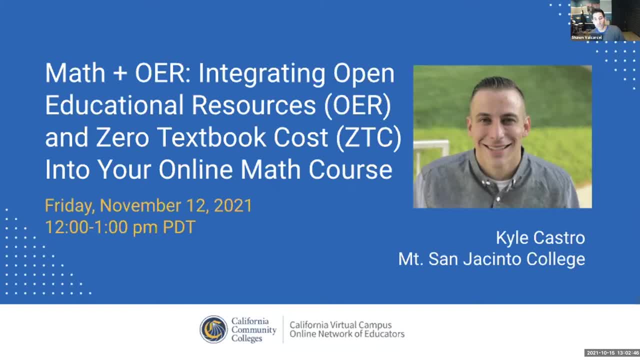 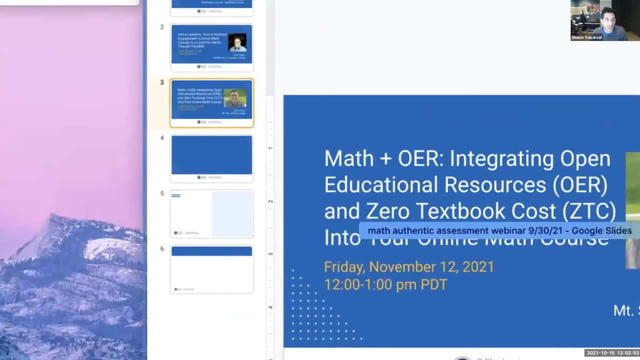 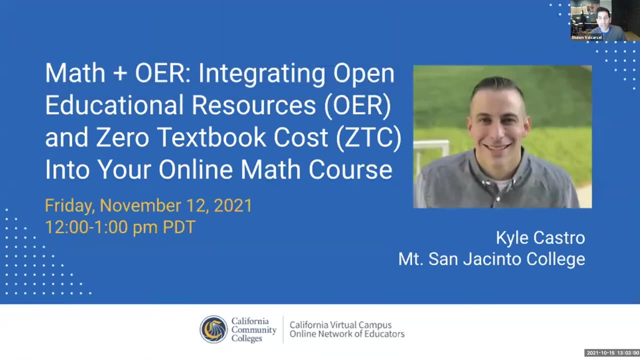 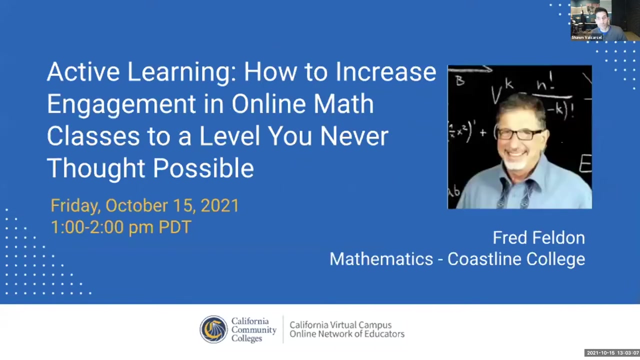 from Mount San Jacinto College So you can check out all our events at cvcedu: forward slash events And let me just drop that link into the chat. Okay, So now Mr Fred Felden from Coastline. He was chair from 95 to 2010,, co-chair from 2014 to 2020.. He was Coastline's teacher of the year in. 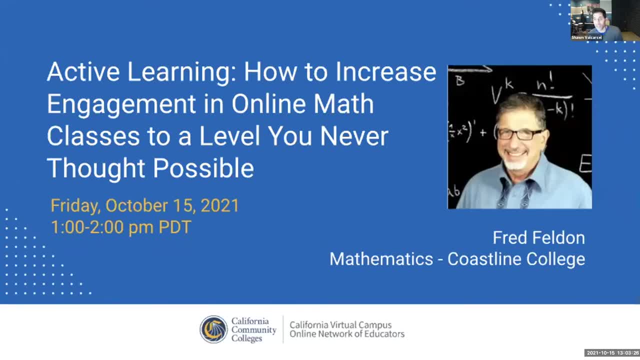 2016.. He is now retired, works as an adjunct And, as we were saying earlier, he enjoys playing classical guitar and riding his e-bike all over town. So already the little time I've gotten to get to know him is he's a great guy. So I think you guys are going to have a wonderful time. And here he is today. 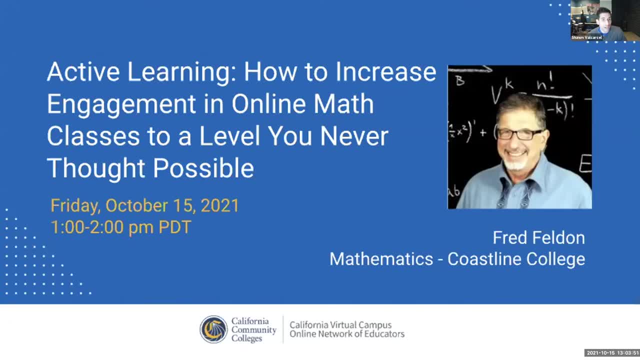 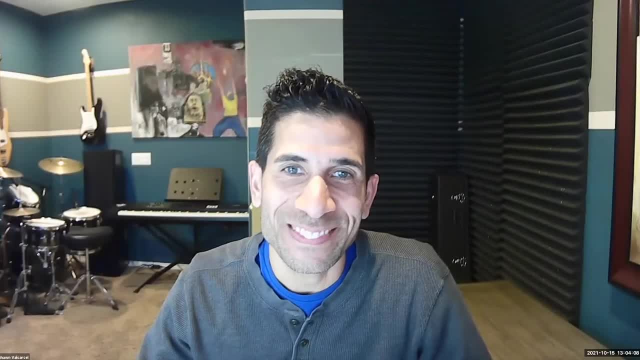 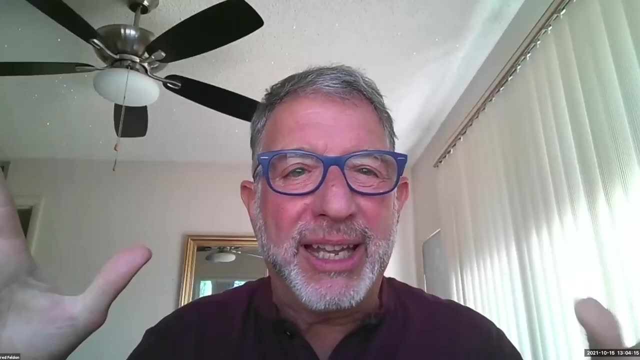 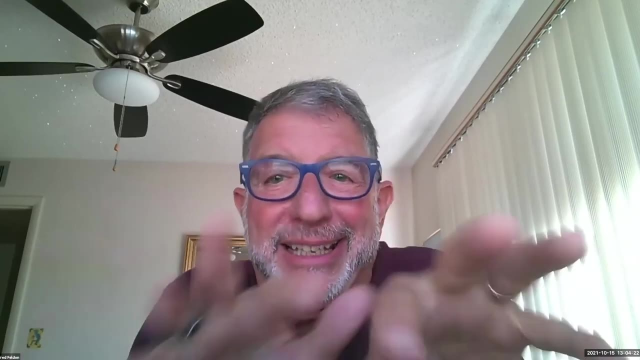 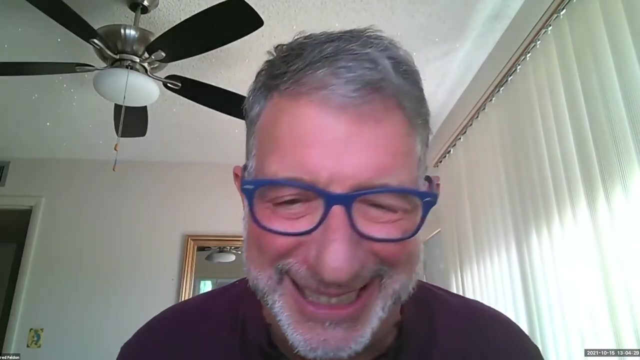 talking about active learning. how to increase engagement in online math to a level you never thought of talking about active learning. how to increase engagement in online math to a level you never thought of talking about active learning. how to increase engagement in online math at a level you never thought of. 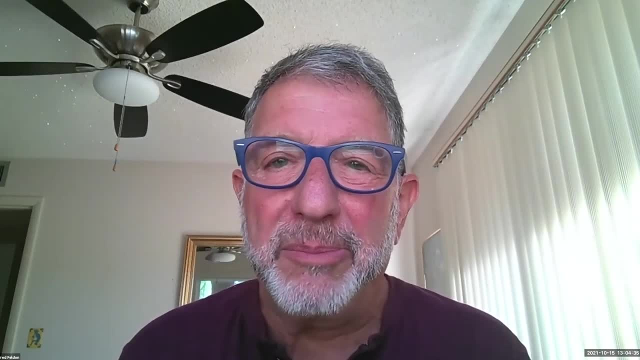 Bye, bye, Love that Shad. thank you, Fred. Wow, what an intro. Wow, what an intro. My God Sean, that's the best intro I've ever had. My God Sean, that's the best intro I've ever had. 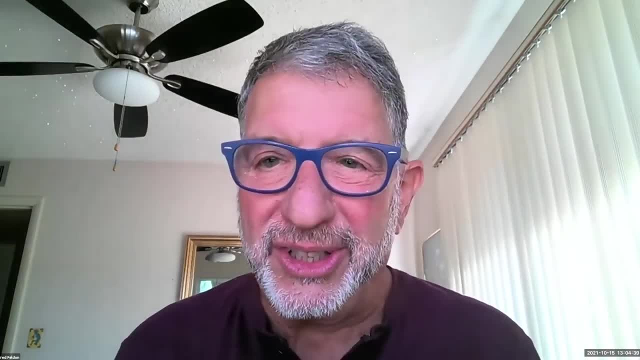 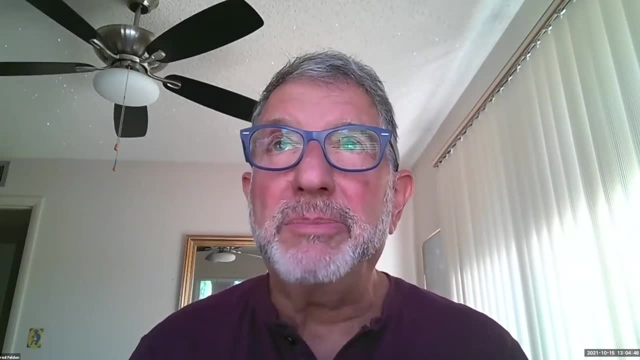 were talking about him having the best of both worlds- teaching and working for the cvc- and i've reached a point myself where i've got the best of both worlds- uh, riding my e-bike, playing music but still continuing to teach a couple classes- and the satisfaction you get from it, and not only not. 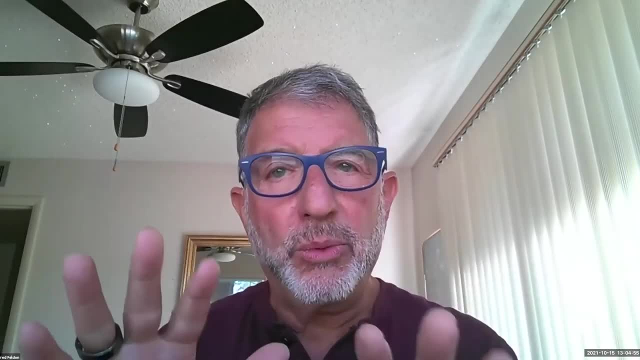 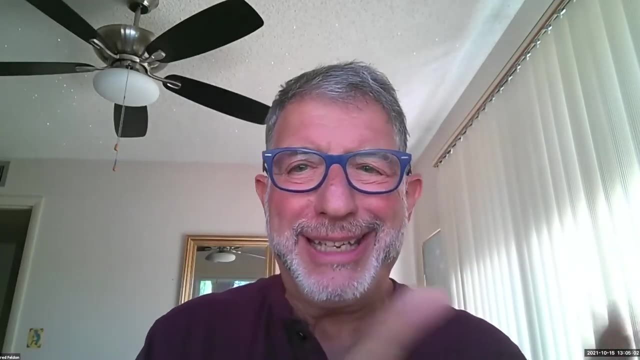 only that, but as a part-timer it's a whole different world. you know, when you teach full-time and you're teaching overload, as i always did, i always wished, i wish i'd had time to do this. i wish i had time to do that. well, as a part-timer, with only two classes, now i can really do the. 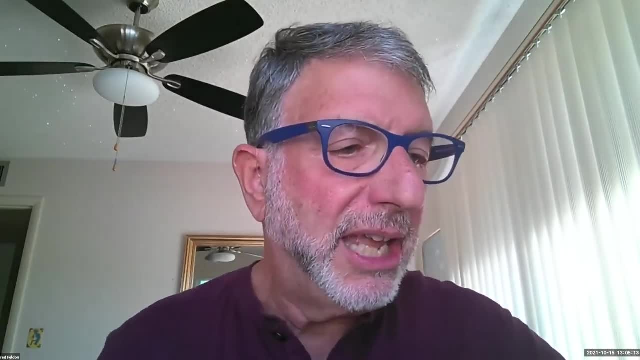 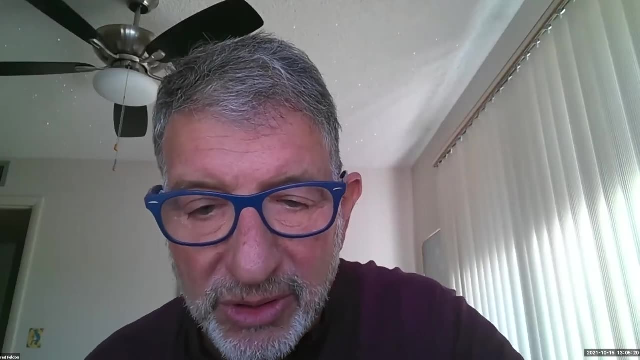 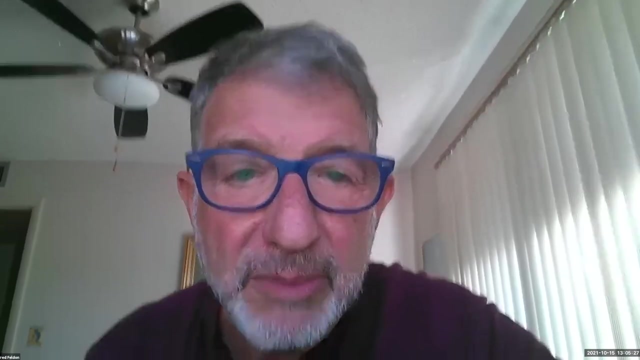 kinds of things that that that create engagement and activity and interaction that i just didn't have time to before. so i feel like i've got the best of both worlds right now. i'll go ahead and share my screen and i'm going to do a portion of the screen. 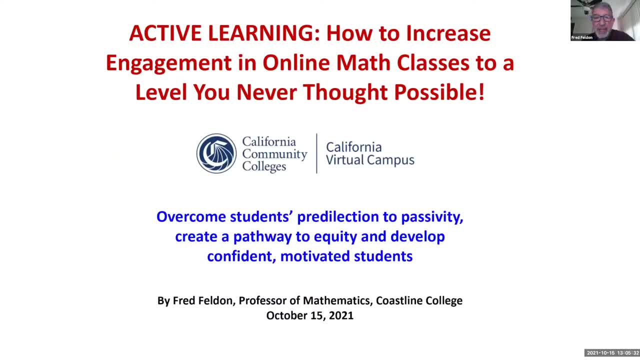 and there it is all right. my ambitious title, uh, the. the summary will be: to help you increase engagement and, at the same time, overcoming students predilection to passivity. that's a. that's a mouthful. i love it. i didn't create that. i read that somewhere. uh, i forget who i could attribute. 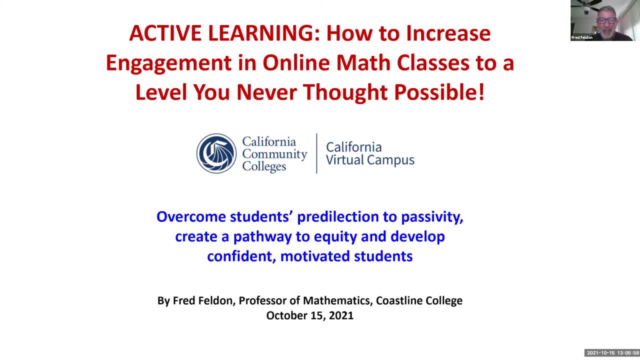 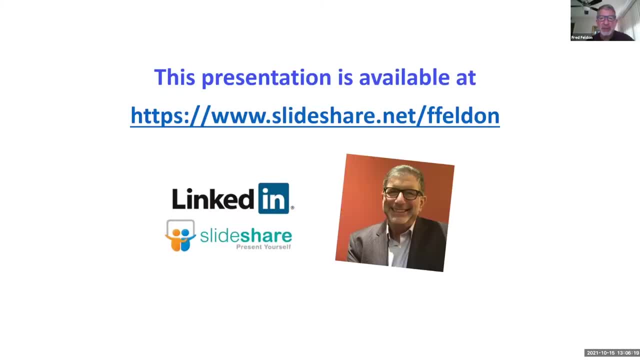 shut off their webcam and microphone and all you see is a you know black square with their name on it. if, if that, uh, by the way, uh, if you want to even go there, right now it exists at a website called slideshare, which was created, i don't know, probably 15 years ago for people who were doing. 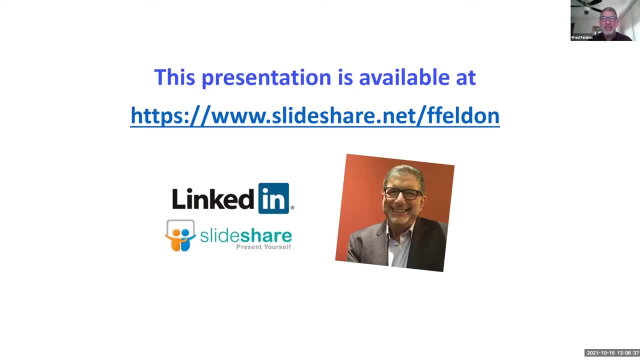 it for the first time, but it was a great way for people to share their powerpoints and, as a social media site, the most popular powerpoints rose to the top. you know how the internet works. the company was bought out by linkedin and actually now it's been purchased by scribed 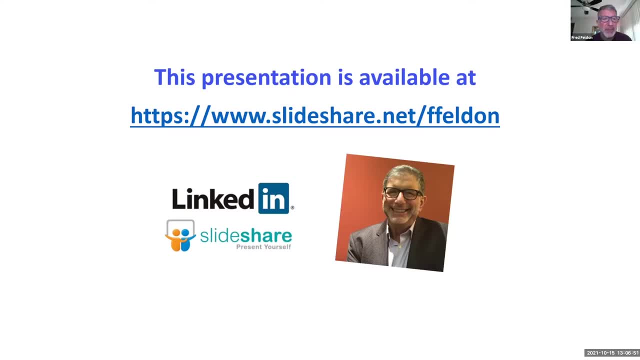 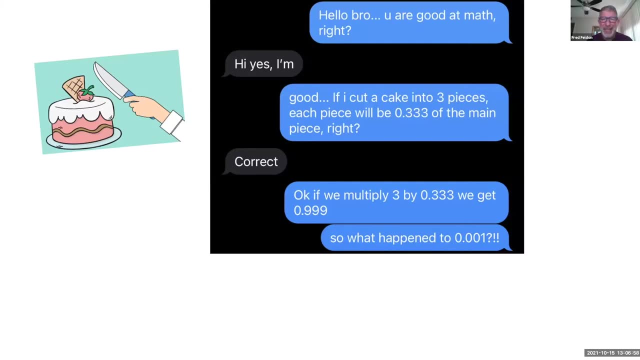 but that's where i host this, that's where i host all my presentations. all right, let's get started by establishing my credibility to you all as being able to have a good joke, a good math joke, in fact. are you ready? so here's a little. here's a little uh text thread. hey, bro, you good at math? oh, yes, i am all right. good, 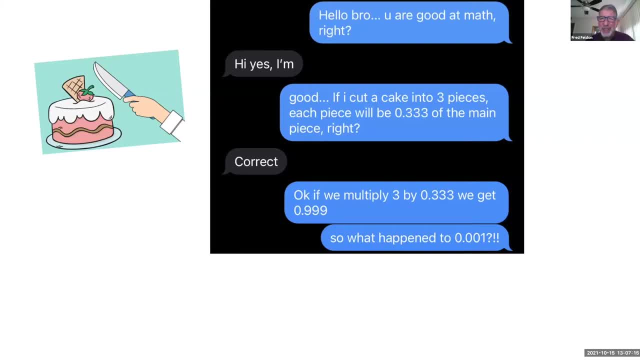 if i cut a cake in three pieces, then each piece will be point three, three, three of the main cake, right, correct? well, okay, if we multiply by three, by point three, three, three, we get point nine, nine, nine. so, dude, what happened to the point zero, zero one? you ready, you will find it on the knife. 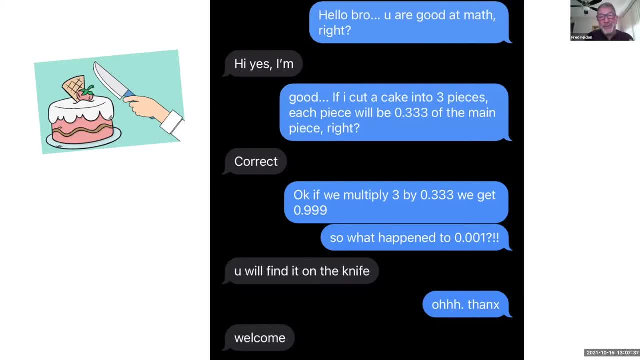 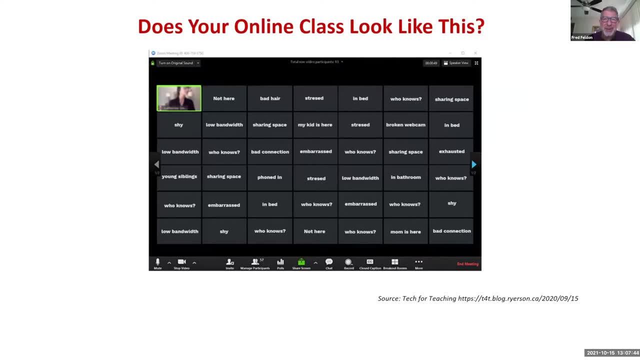 okay, thanks. so there we go. i hadn't heard that one before. i hope you hadn't either. so right off the bat, i'm establishing my credibility because i can share a good math joke. i do have a lot of slides and i will not be spending much time on each one. i'll be moving along pretty fast. 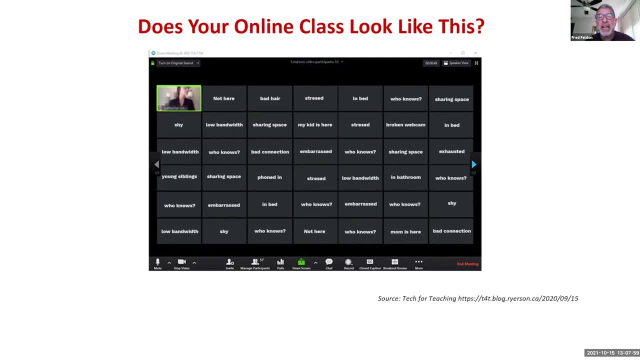 but, as i mentioned before, a zoom class often looks like a bunch of black squares and it's kind of for me like a bunch of black squares. but in the time i spent on them for the past three years- and i'm, you know, with the fact time- i'm pretty sure that i can easily fit into a bunch of black squares. 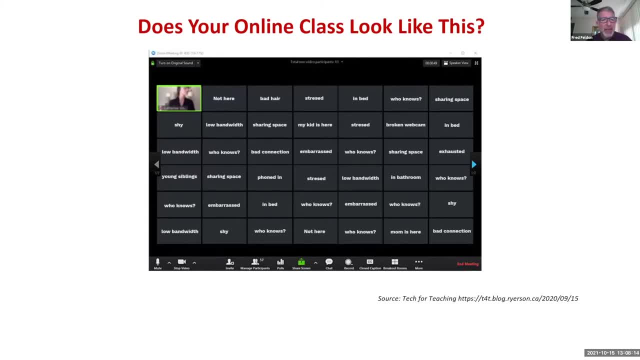 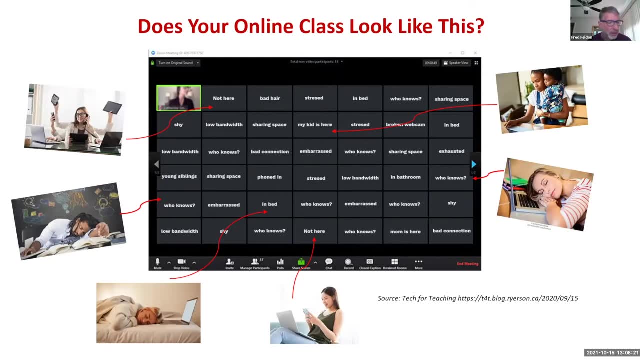 and i think being able to go and actually get in the class and don't get mean, i thought was kind of depressing. and you know, on the one hand, you can't force students to participate, let alone turn on their webcam and microphones. so how do i encourage them to do so when they may be? 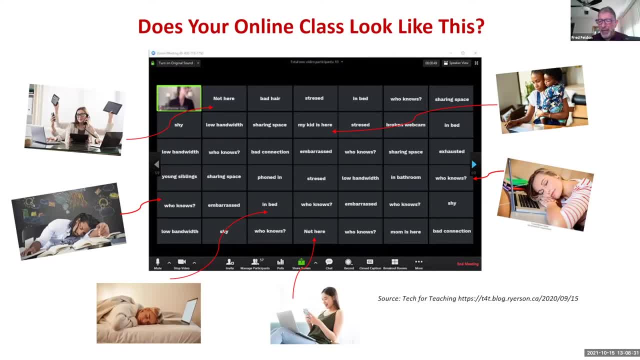 doing things like taking care of their kids or multitasking or catching up on their sleep in and have to ask to go to the bathroom in my own house Or another one online school. Oh, you mean the background noises when I'm cooking dinner, watching my kids or watching. 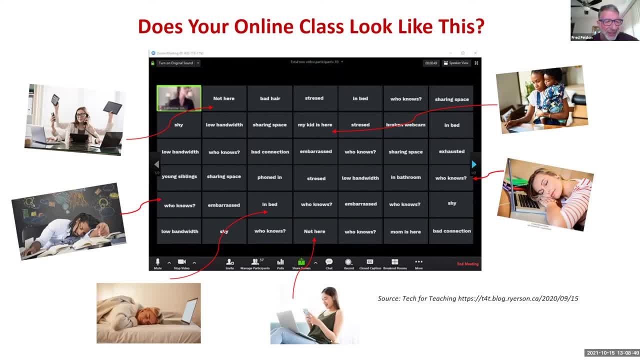 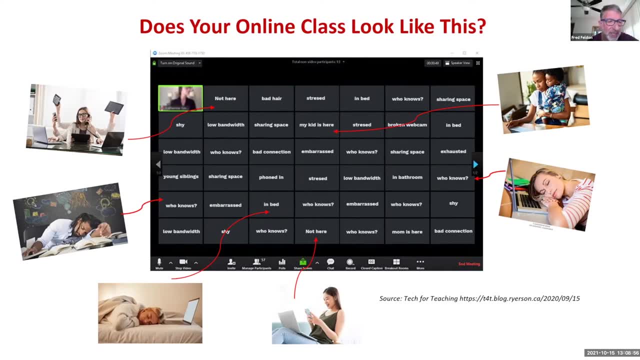 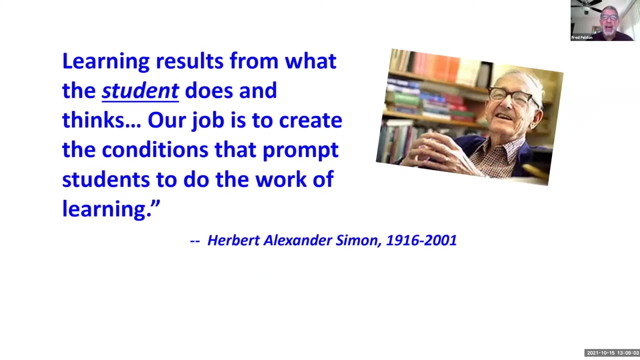 Netflix. So it's a whole new world out there for us And it's a big challenge to us folks that are teaching online. But your goal is to you know. what you do doesn't matter. If there's one hot point, that big point that I could make in today's webinar, is that you know in the classroom. 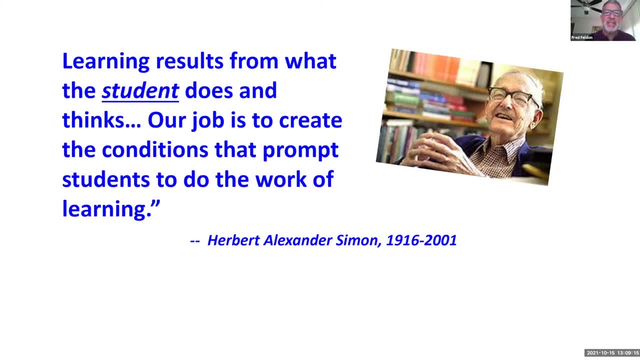 I thought I was an awesome teacher. I had all kinds of collaborative activities and group work and participation, where I actually sat on a seat with the students in the class and students came up to share their Thinking and explain their problems that they solved. And you know, doing that online was. 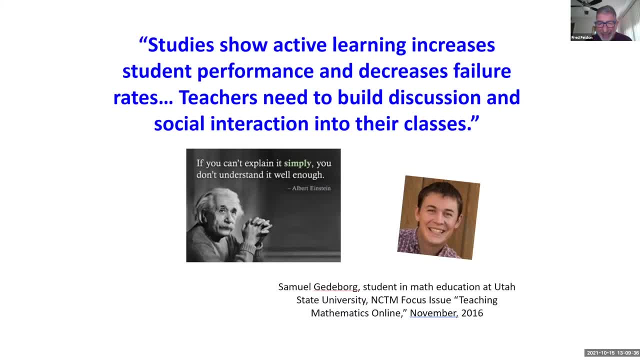 super hard, But, as this kid, who is a student himself at Utah State University, said, you just need to build discussion and social interaction into your classes, And if you explain it to your students that it's the way you learn best- if you can teach someone else, I think they'll get it. 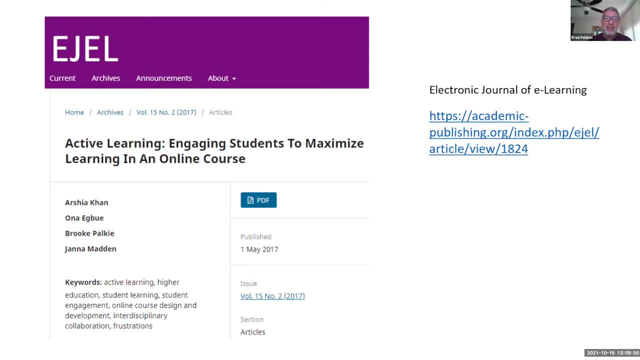 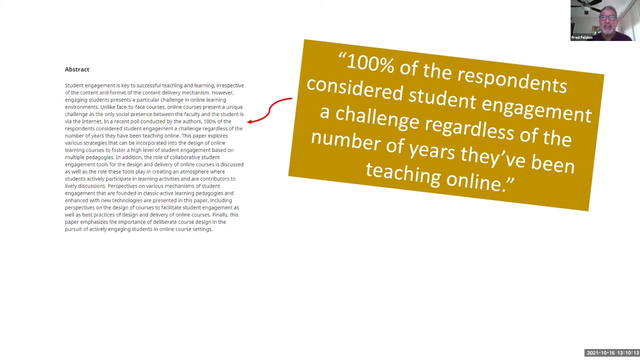 But even the researchers who've studied online teaching and learning in depth can tell you that, no matter how long you've been teaching online, student engagement is the biggest challenge, And it certainly was for me. I can tell you about 10 years ago I was at an AMATIC. 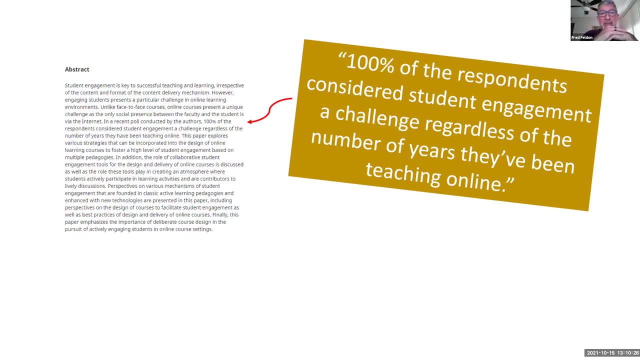 conference with one of my best friends and mentors, And I was at an AMATIC conference with one of my best friends and mentors, And I was at an AMATIC conference with one of my best friends and mentors, And I was at an AMATIC conference with one of my best friends and mentors, Maria Anderson. you. 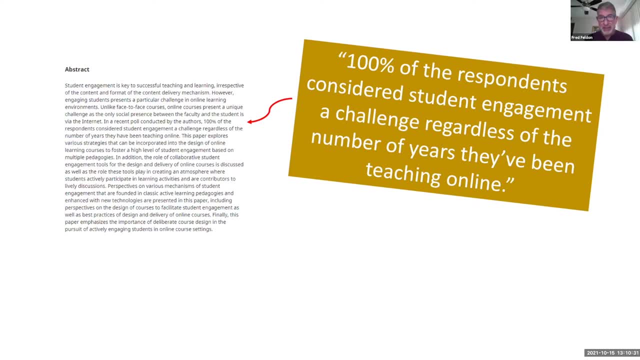 probably know her. She was a keynote speaker at a recent AMATIC conference And just a guru in terms of pedagogy and educational technology and teaching and learning. And it happened to be just the two of us and we were having dinner and she says to me: Fred, this was 10 years ago or so, Fred, what? 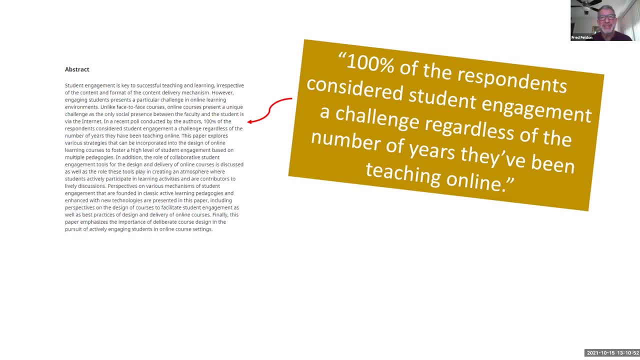 are we doing to these poor students? And that just hit me, even though she and I were probably leaders in technology. I mean, I've been teaching online since 1999.. I was a pioneer when it first began. I used WebCT, which is basically just an empty shell, and I had to fill it all in by hand. 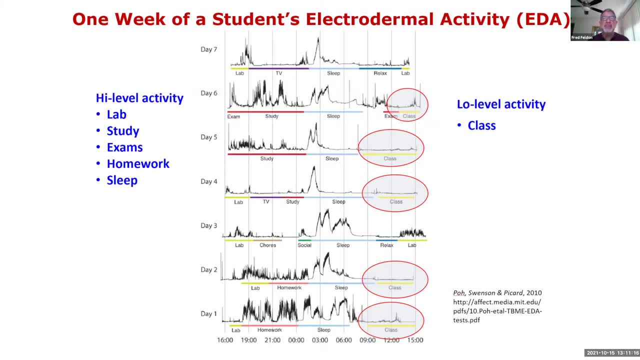 And then gradually, the publishers- Prentice Hall and Pearson- began to create CSMs and learning course management. And then gradually, the publishers- Prentice Hall and Pearson- began to create CSMs and learning management systems and it's really gone far. 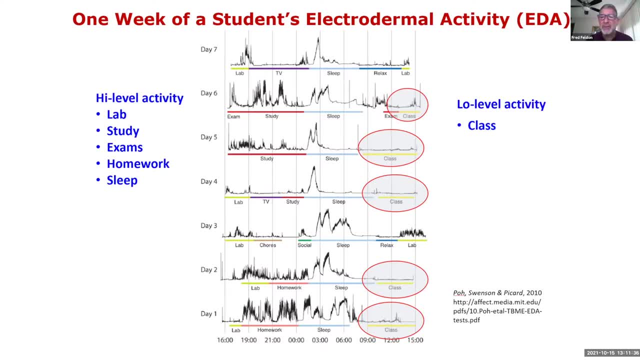 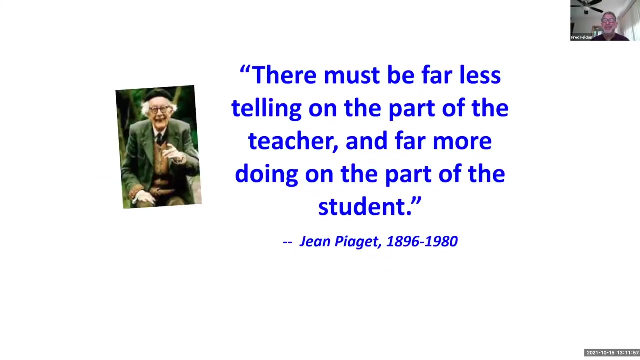 It's wonderful that the technical expertise that we have now from the publishers and from our peers, But the big problem is that class- but being in class in a physical room or online is basically, as measured by scientific experiments, students least brain activity where students least thinking occurs, and so what you want to tell yourself is: 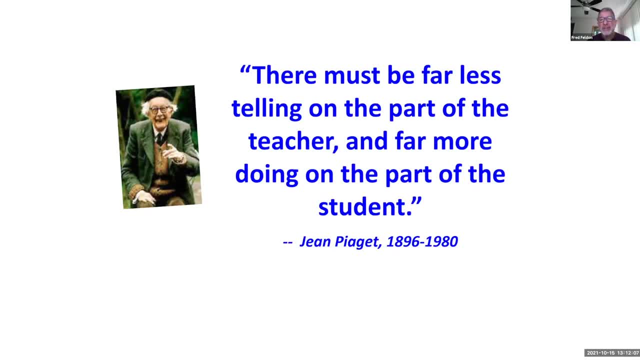 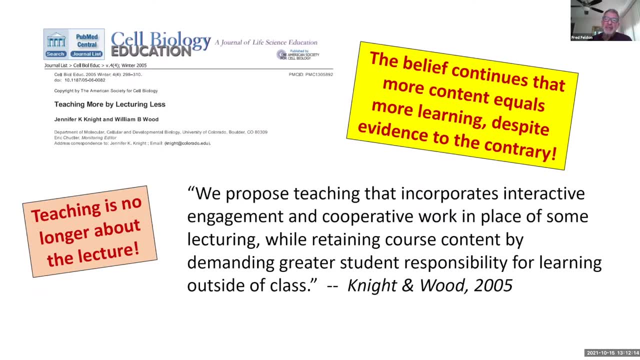 that the more I talk, the less they learn that that the biggest negative or the biggest challenge I hear from my colleagues is that man, we have so much content to cover so in the classroom and and online, isn't my job mostly to share that content with my students? I mean, I studied math. 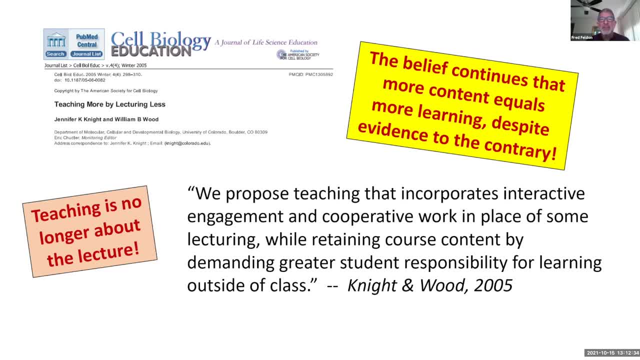 I have an advanced degree in it. I've worked with thousands of students over so long that I know. I know what they need to know, I know the shortcuts they need to learn, I know the procedures they need to become adept at. but it's. teaching is just no longer about the lecture and about delivering. 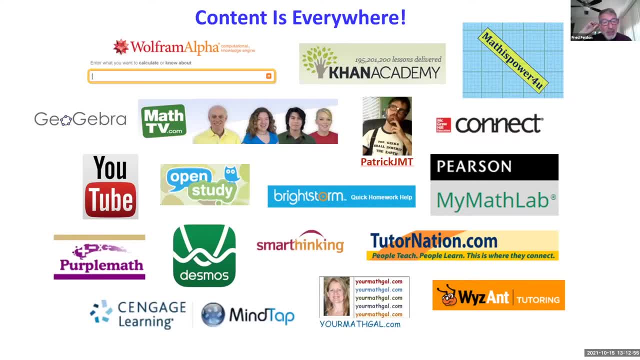 content. that's because content is ubiquitous. it's everywhere. you have internet gurus and textbook authors like Pat McKee. you see him in the yellow shirt there in the math tv picture. if you have never been to his website, it's awesome he. he covers material from the 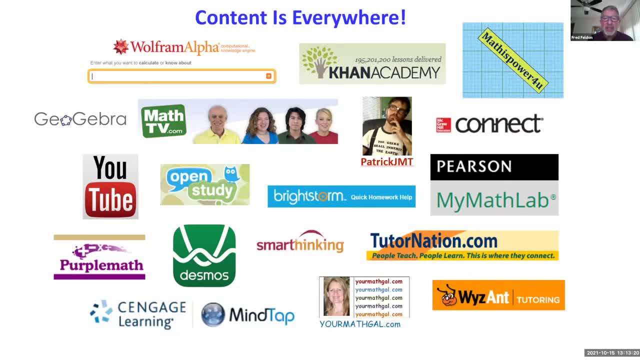 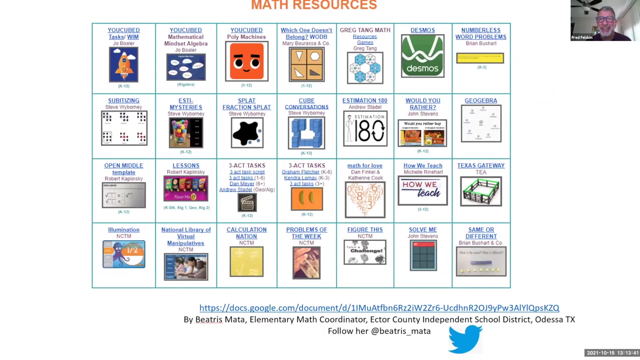 full range of classes we teach at the community college level. he shares a few problems and he has a group of students that share their problem solving techniques in multiple languages. it's just awesome if you're not following our k-12 brothers and sisters right like in the NCTM or locally here in California in the CMC, the California math council. 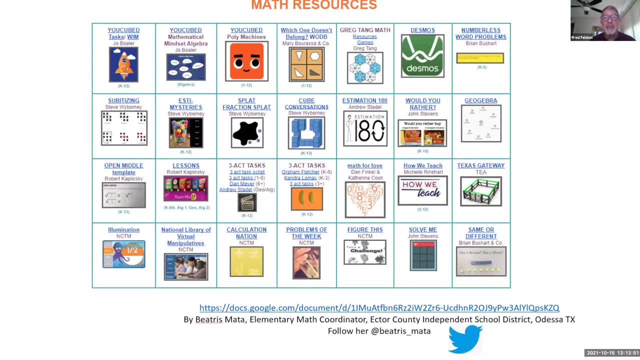 they have conferences. you should go to the CMC conferences. you could learn a lot from our k-12 peers because, let's face it, aren't we all teaching the same thing? I mean, maybe k-12 doesn't have linear algebra and differential equations. maybe they do, but they've got everything else, we're all. 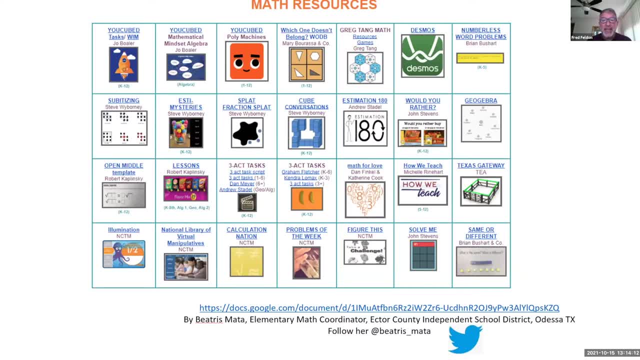 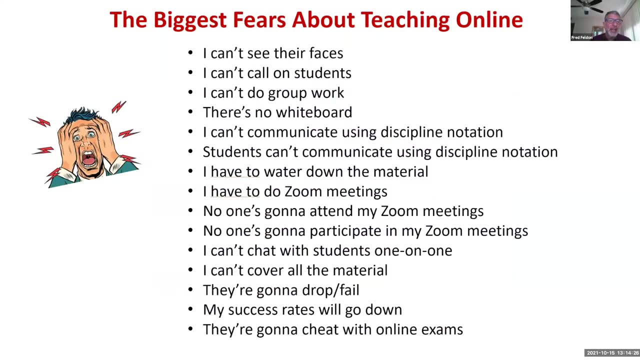 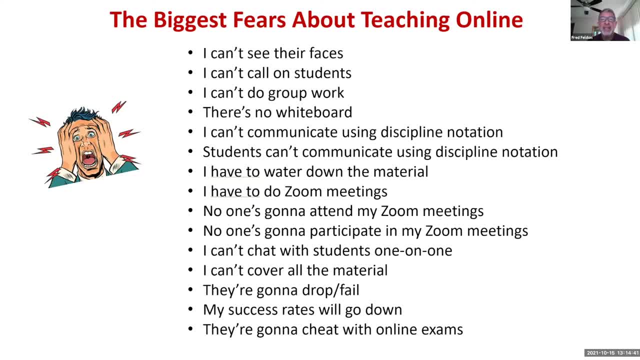 and a speaker and a presenter and an attendee at conferences all across the country. these are the biggest fears that I hear about professors and I'm worried about teaching online and I myself faced all these fears and I've missed any. you have to let me know if you, if there's another fear that should be included. 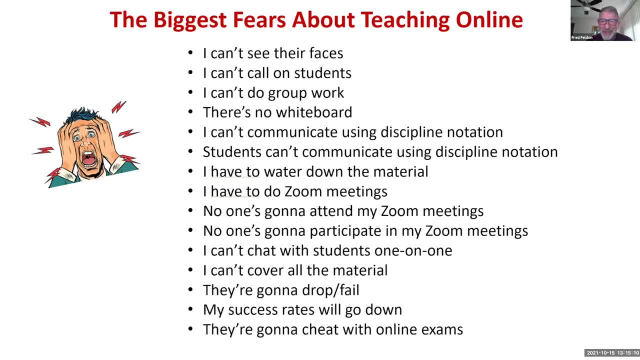 in this list, type it in the chat and, uh, Sean can share it to me. and hey, by the way, speaking of the chat, could you do me a favor? I'm assuming that the audience is community college math faculty, but I'm just curious: if you are teaching a discipline other than math, could you type: 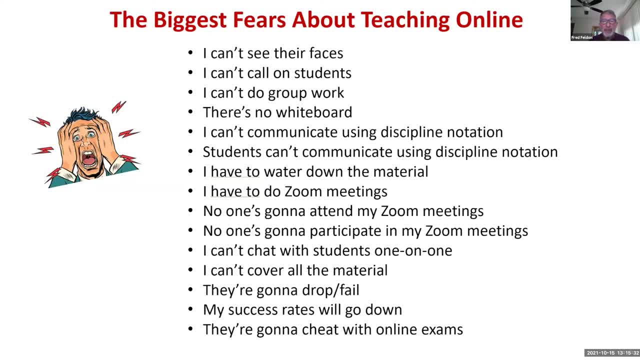 it into the chat box right now, and if there's nothing that shows up, I'll assume you're all math folks. otherwise, Sean, you'll have to tell me if there's any other disciplines out there besides math. well, we have some instructional designers, oh. so, uh, physics, um, we have a couple that teach. 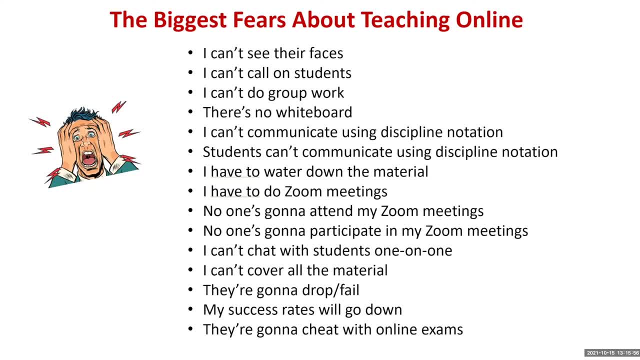 physics awesome. well, I would lump the physics in with math as a stem discipline where the notation is a challenge. almost every other discipline- history, sociology, psychology, you name it- you can type, you know, your your thinking, students can type their thinking, but with math it's very difficult to type math on a keyboard. 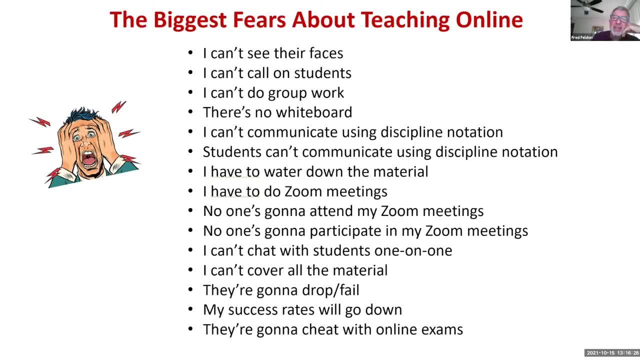 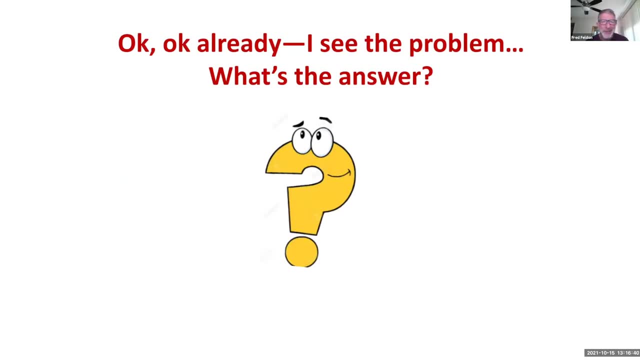 And I'll talk about that notation in a minute. But I think instructional designers and STEM faculty will benefit from this talk, as will the rest of us math folks. All right, so enough about the problems and the challenges. Well, what is the answer? 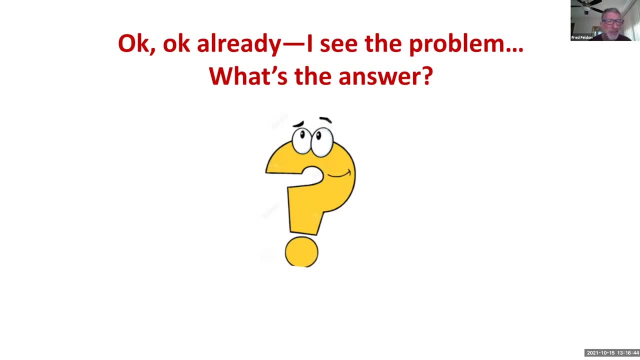 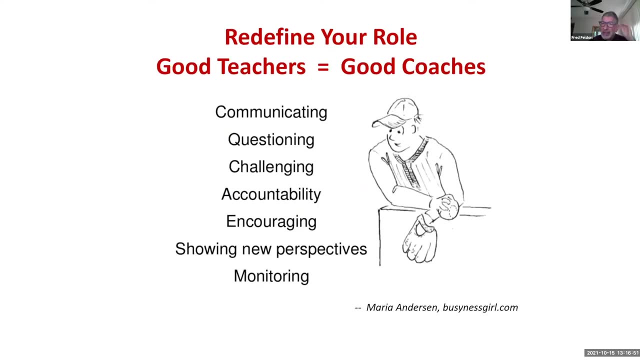 I'm hoping that I can address most of those problems that I had on the previous slide And I think the big thing is a mindset. You know, growth mindset especially is something that we're advised as faculty and instructors to encourage our students to develop. 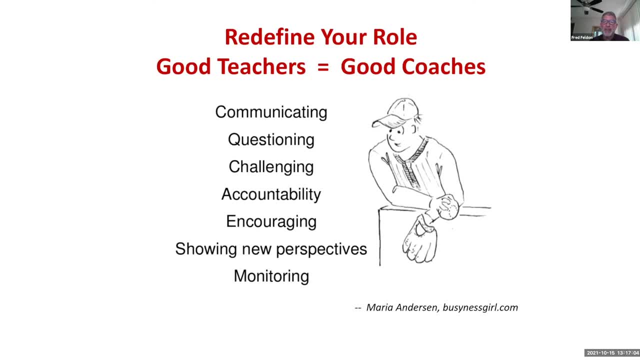 And I think the same thing is true for us. As I mentioned earlier, lecturing and delivering content is not our. it's a very small part of our role, And the roles that I have listed on the slide are the same as the roles that I have listed on the slide And the roles that I have. 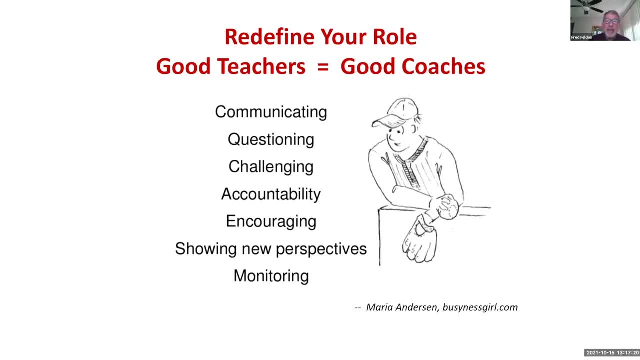 listed on the slide are the same as the roles that I have listed on the slide. And the roles that I have listed on the slide showing now are huge, And with the pandemic they've become even more important. I can't tell you, not so much now, but in the early stages of the pandemic, as I read: 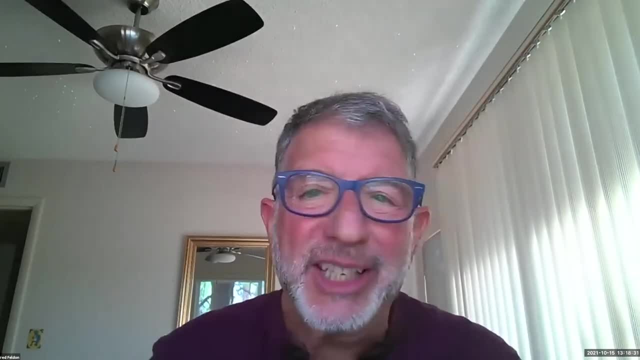 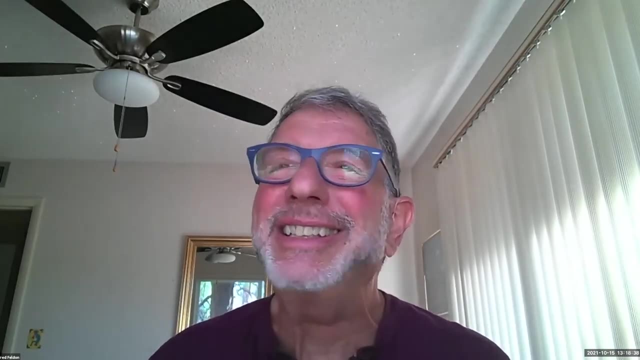 Here's where I was when I lost the connection. I'm actually speaking to you from a small town in Arizona. I'm in Sedona, I'm nestled among the red rocks in Sedona And my internet is pretty good, but I guess I did lose it. Thanks for letting me know, Sean. 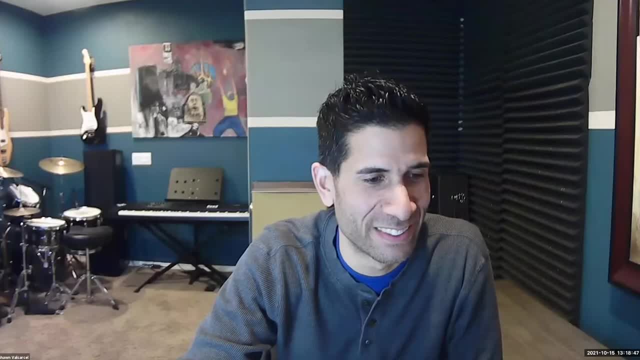 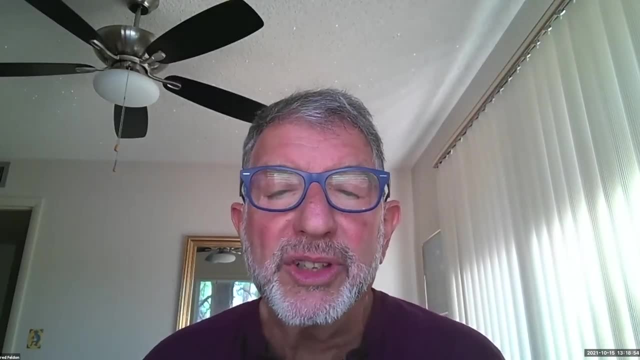 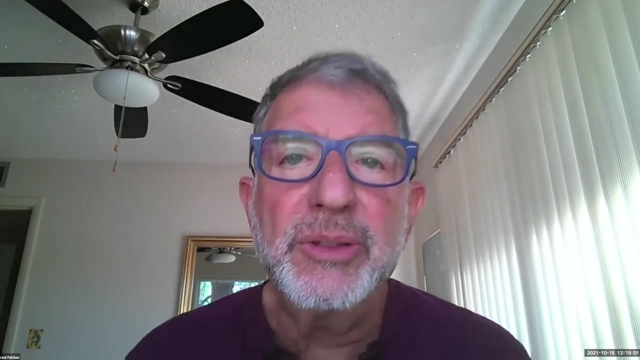 For sure. So, as I was saying before I got cut off that this was always an important role, And with the pandemic it's become even more so, especially in the early stages when I reached out proactively to students who were not keeping up with the syllabus, students who were not 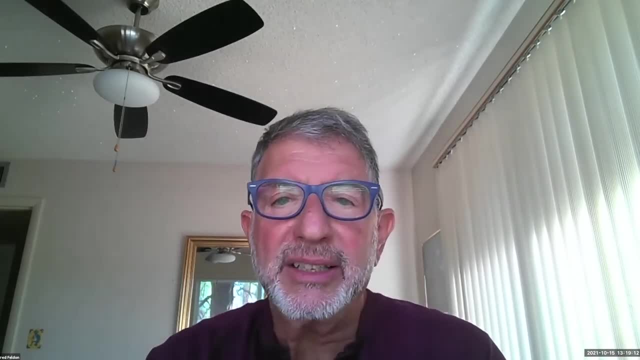 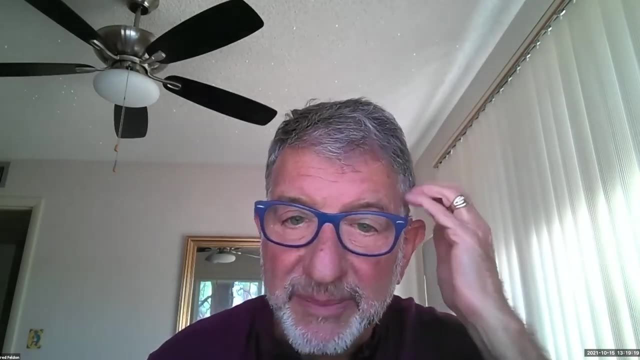 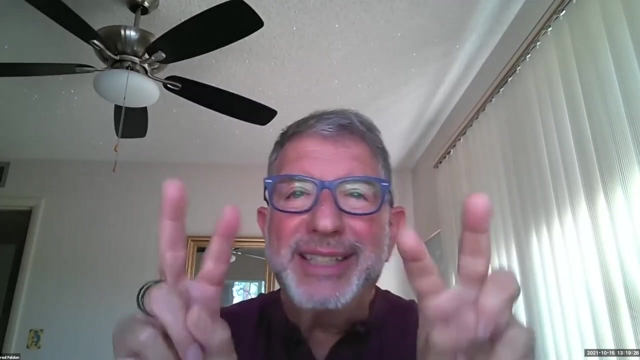 earning an overall passing grade Who are not attending Zoom classes. I heard some horrific stories and it's just really important to encourage everyone and offer huge amounts of flexibility And what you can. you don't need to worry about wasting time delivering content, because computers can do that. You don't have to. 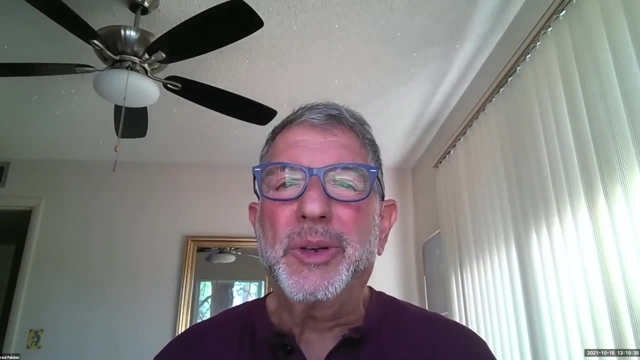 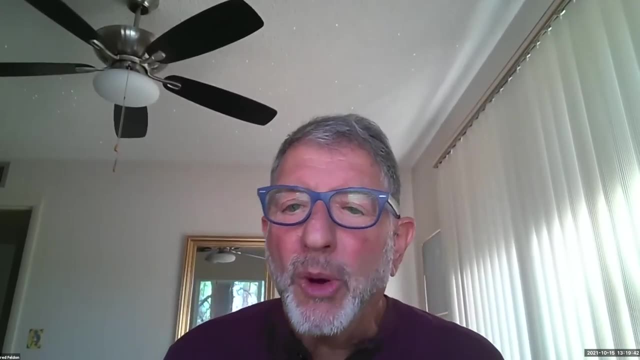 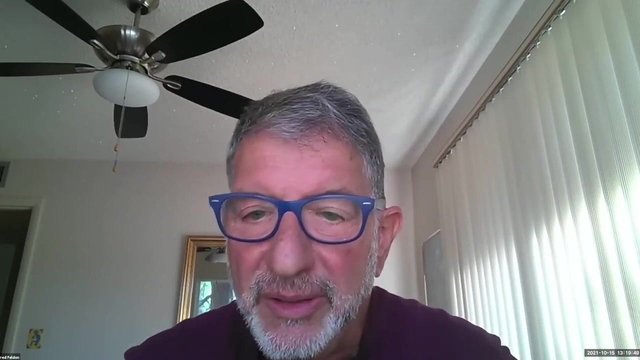 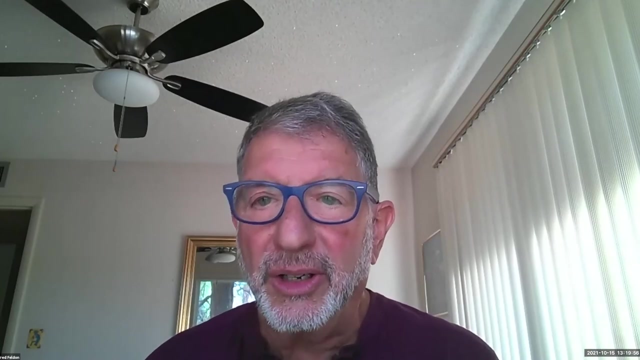 worry so much about answering questions on the homework or quizzes, because computers can do that. So your essential role is more facilitating and coaching, as you can see by this large survey that was administered to a thousand students. Well, you think is important that your teacher should be doing. 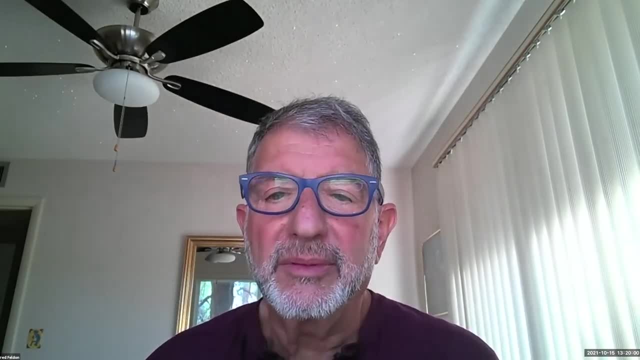 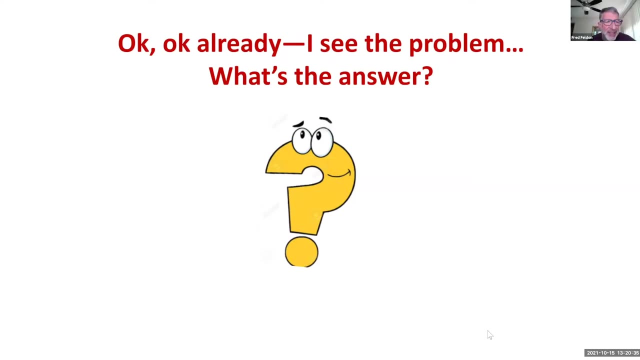 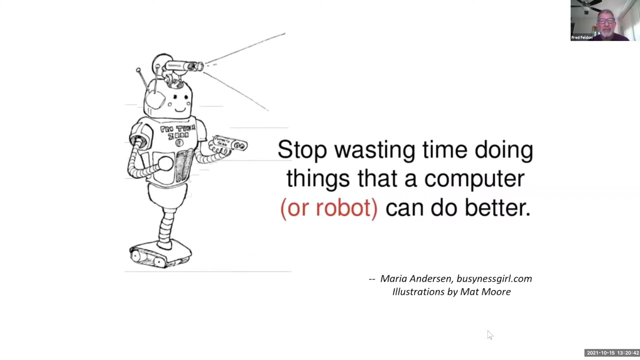 and notice that direct teaching was very low in priority. Sorry, So there, I was talking without sharing my screen, Thanks. So I talked about redefining your role. I talked about not wasting time to any great extent going over homework delivering lectures. 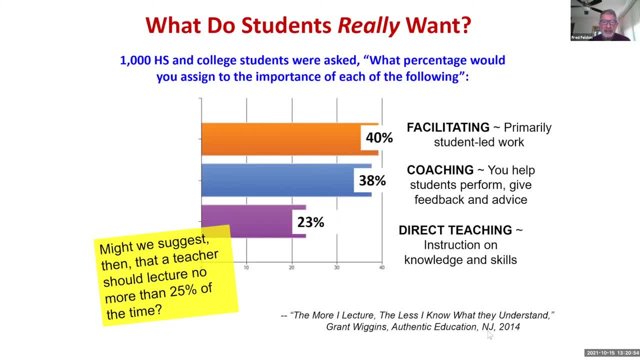 Computers can give instant feedback on homework and quizzes to students, And what I encourage students to do is, if they don't understand the feedback they are getting from the computer, to do a screen grab, post their question on a discussion board and ask questions to the entire class. 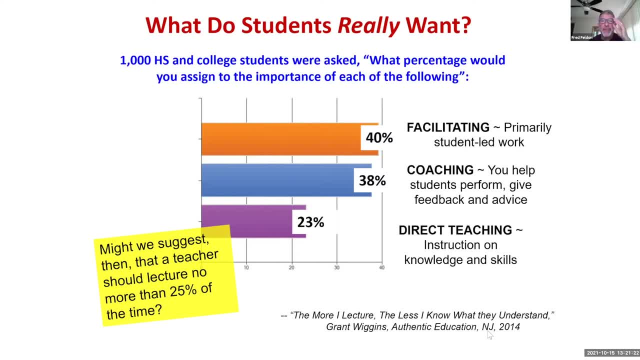 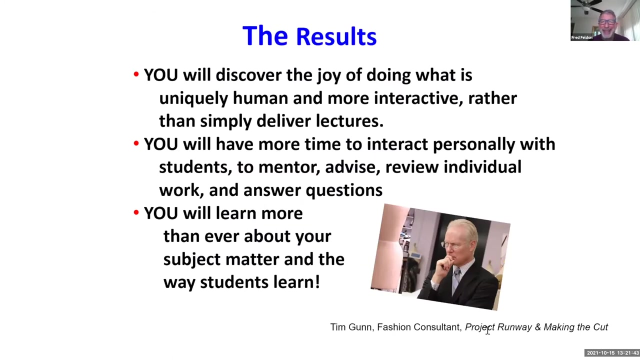 And in other words, to develop a learning community, so that I'm not bombarded with emails, that students learn how to ask their peers and become adept at peer instruction, So that lecture time becomes limited. Instead, you get to do things like having a good time and motivating students. 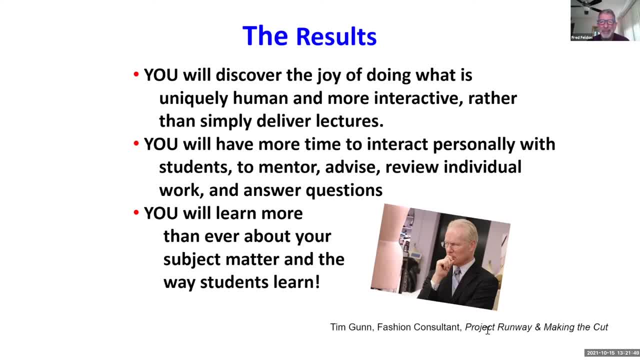 summarize and highlighting students, mentoring students And, frankly, I've learned more about my subject matter and the way students learn by talking and lecturing less, When I, as I mentioned earlier, I often in the classroom, would sit down and have students come to the classroom. 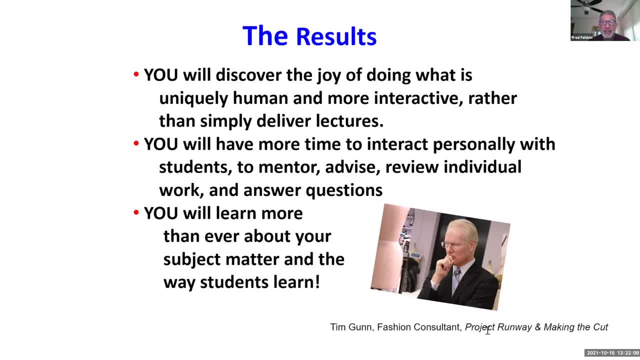 and talk to the board and solve problems And I would learn new ways that students got answers And you know they would ask me: is this right? And we would. in fact, I have to tell you a story real quick about my most amazing 20 minutes of teaching in my 25 year career. 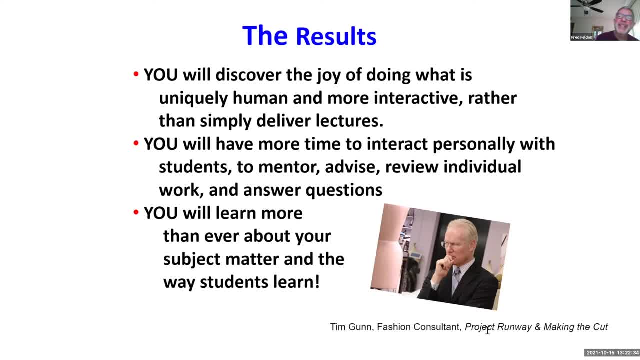 It was in a basic math class, believe it or not, And we were going over subtracting mixed numbers with borrowing Like: what's seven and a half, take away three and seven, eighths, Right, you've got to borrow and rename, and all kinds of good things. 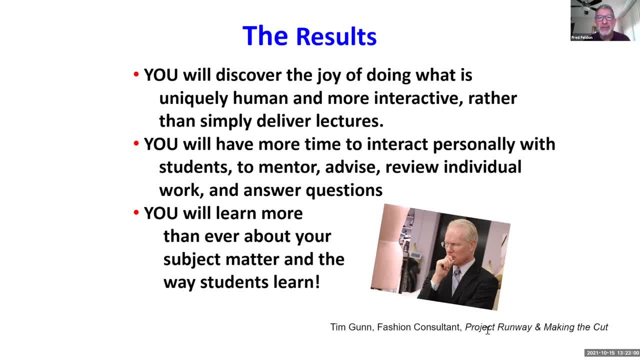 So I said that's a great question, Would someone like to share what they did? And a student came to the board. I said I stood off to the side and they worked it out. The answer was wrong, but I didn't say that. 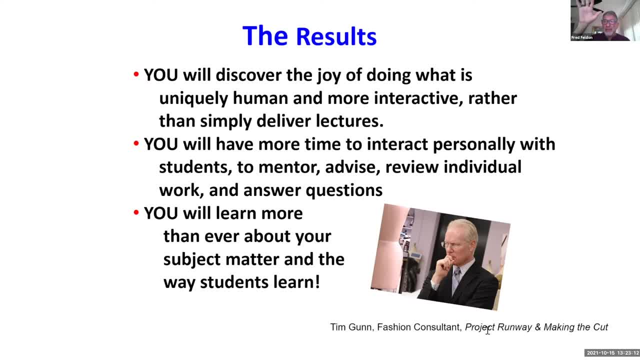 Instead I said: did anyone get a different answer? Sure enough, another student raised their hand. They came up, worked it out alongside the first student. got a different answer. It was also wrong, but I didn't say that. I asked instead: did anyone get a different answer? 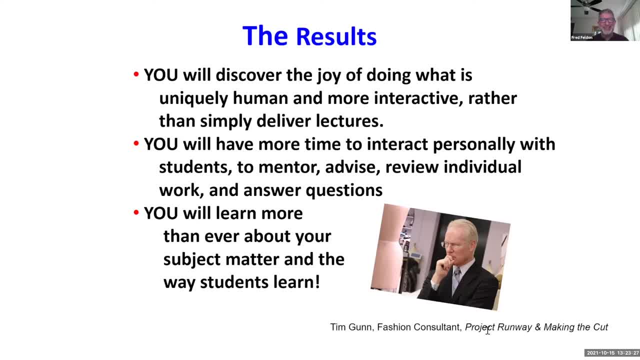 Third student came up, worked it out, got a different answer. It was also wrong. I was loving this And I said: did anyone get a different answer? The fourth student came up, worked it out, got the right answer. But I didn't say that. Instead I said one of those answers is correct. 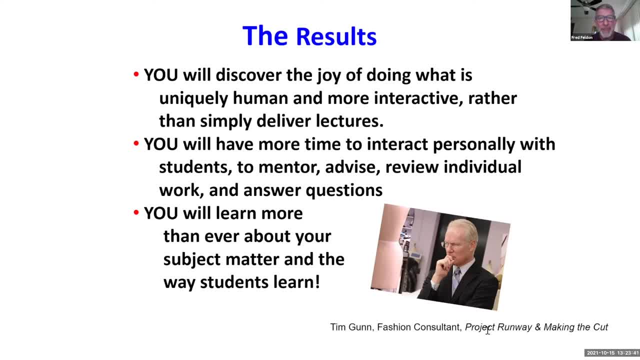 Which one is it and why and what happened. And they just started breaking up into groups and chit chatting away And, man, there was a lot of learning going on and a lot of peer teaching going on, And when we were done- I you know- I said what do you guys vote? 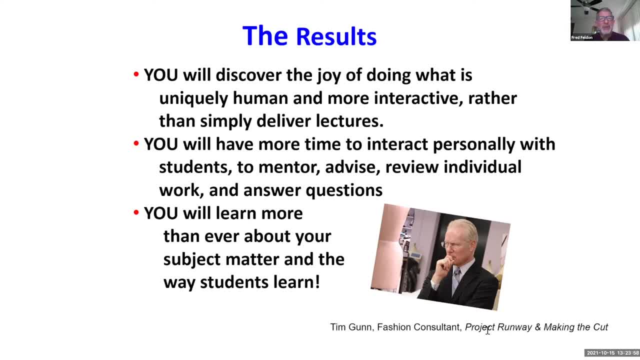 Which do you think was the right answer? Who can share what they discussed in their groups about what the students made that led, Yeah, to the wrong end? You're back, Oh good, OK. OK, yeah, I'm getting a message. My Internet connection is unstable. 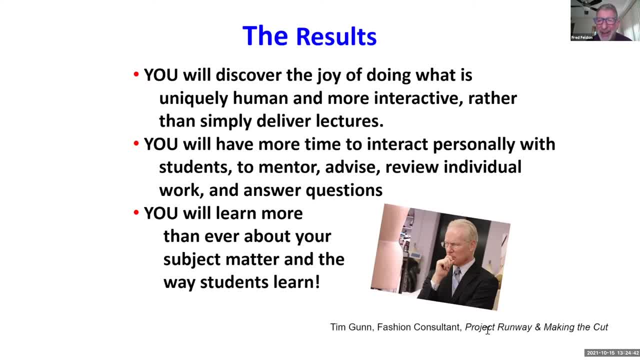 Boy, I've got the latest and greatest 5G at the house, But so backtracking. I was just saying that it took over 20 minutes to explain this one problem- subtracting mixed numbers with borrowing, And I had to tell them how valuable that learning experience was. 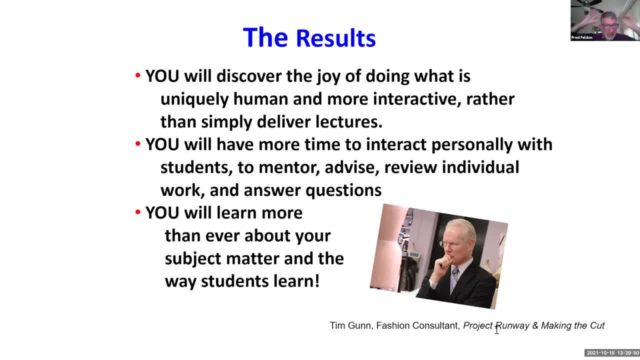 OK, so I was saying about this great 20 minutes, the 20 minute lesson, and the importance of selling what you do to your students, Because they may expect just traditional lecture and they may resist your emphasis on deep understanding, your emphasis on collaboration and cooperation, and you have to sell it to them. 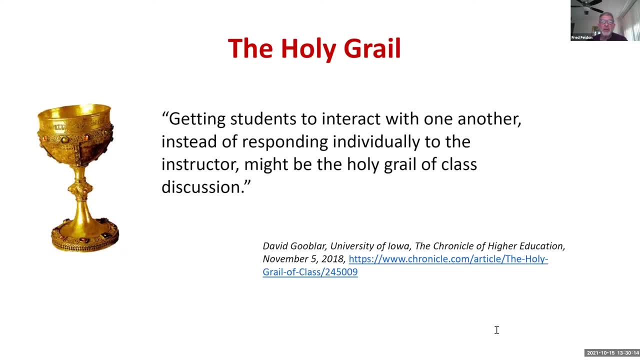 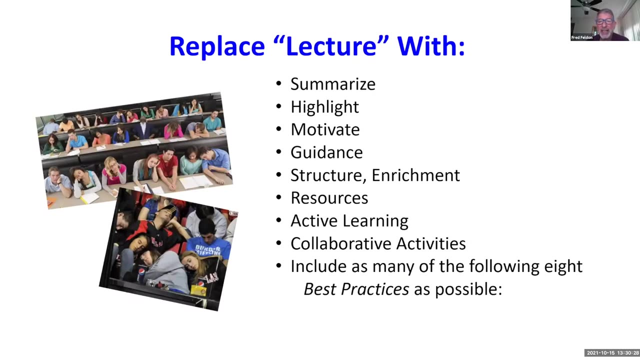 But I love this quote that the Holy Grail may be getting students into. The Holy Grail may be getting students to interact with each other, because the less you talk, the more they learn, And what you can replace lecture with is summarizing, highlighting, motivating, providing guidance. 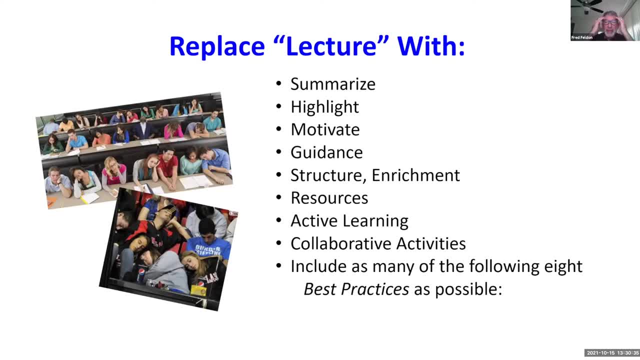 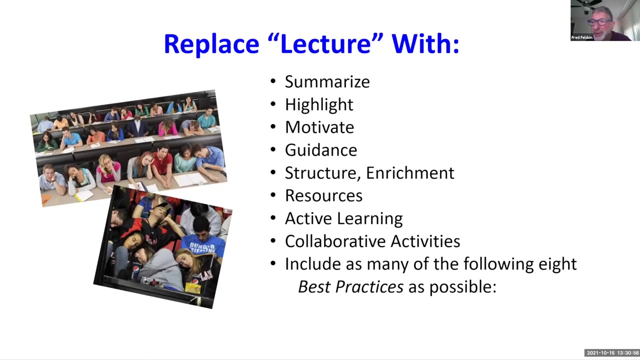 You need structure. of course, And because you may, I was involved in a great Twitter debate with a K-12 hashtag About the- The movement nowadays to minimize advanced placement classes, and parents are freaking out because they're gifted children will not be challenged. 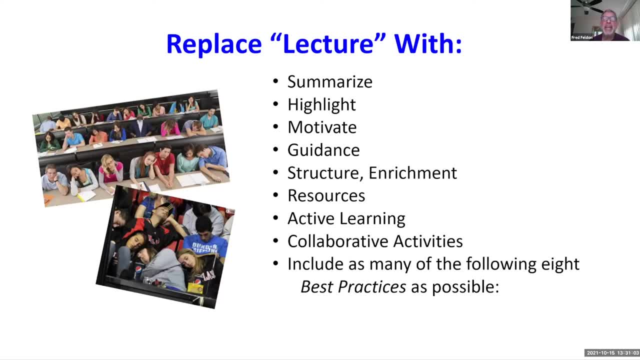 Similarly, if you're facing a class of heterogeneous students, you are going to have some students that will be gifted, And if you can provide enrichment to them- which I do in the shape of extra credit- Everybody loves extra credit- I'll find a challenging activity that's related possibly, or maybe even not related, to what we're studying in the class, and post that. 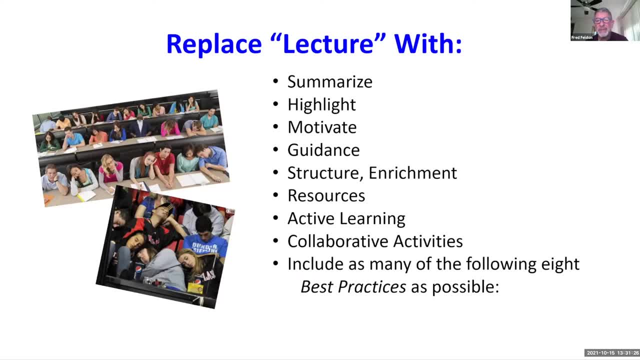 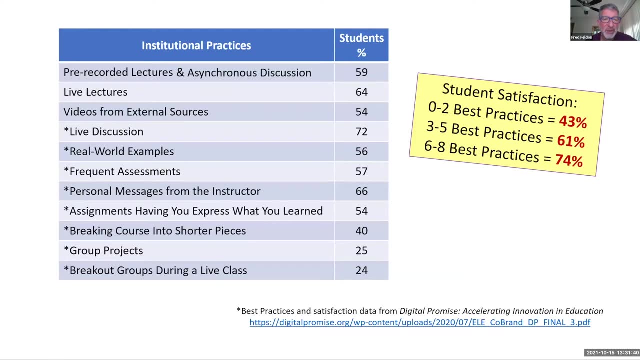 So that should be part of your instruction as well- Enriching gifted students with activities that challenge them, In addition to active learning and collaborative activities, and you want to include as many as the following eight best practices as possible. All right, So the top three are what all come to mind when we think of our role as a community college instructor. 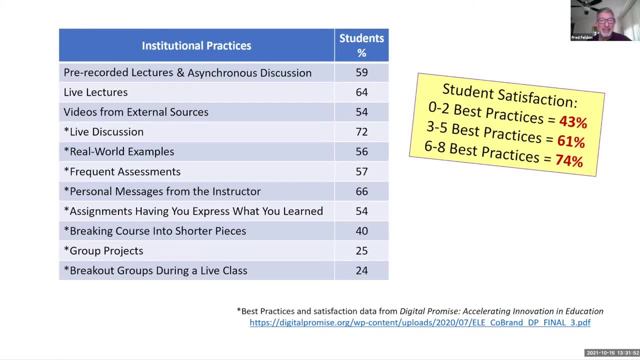 But the next eight are said to be best practices, And the more of those you can include, The more effective your teaching will be, The more successful your retention rates will will be And the more student satisfaction you'll experience. You know, you just. 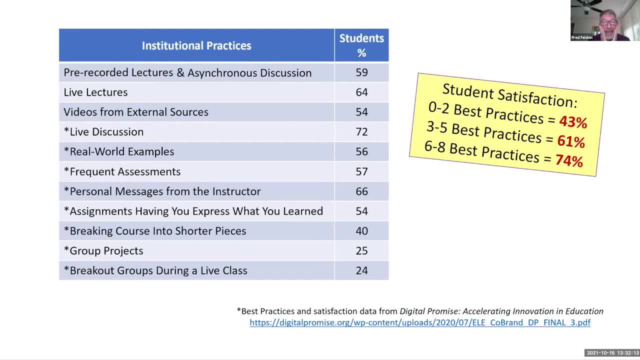 You know you're going to be able to do the things you may not think about, and I don't do them all. I have to admit my failing is in the group projects. I still don't feel comfortable with administering and incorporating group projects in my online courses course. I never did it in the classroom either. 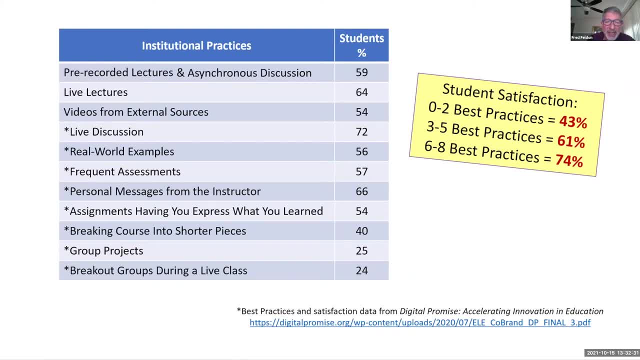 I did a lot of group work And you know, but I haven't done a group project. But notice that I've done. I think I've done all the others. so I'm right in there between the six to eight For optimal satisfaction. 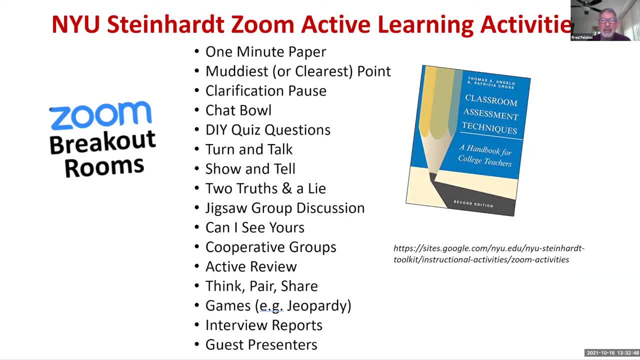 NYU has a great website for prospective teachers. They have a toolkit, the website I give you there and small print on the screen. And you know, I've done almost all of those things. I think my favorite might be two truths and a lie. 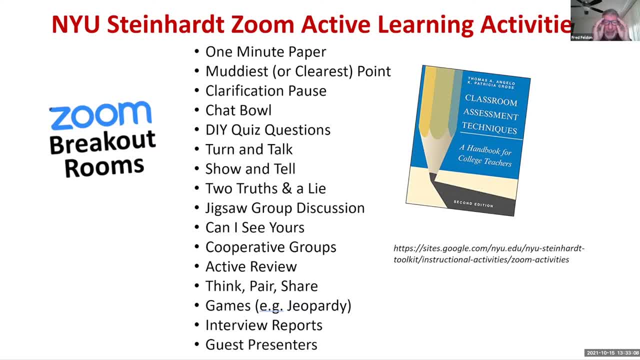 I'll, I'll pick. I'll pick a couple of statements from a topic we might be learning. I'll pick three of them And I'll say all right to two of those state, to those statements or equations or whatever are false. One is true, which one? which ones are? they break up into groups and I'm going to give you 10 minutes. 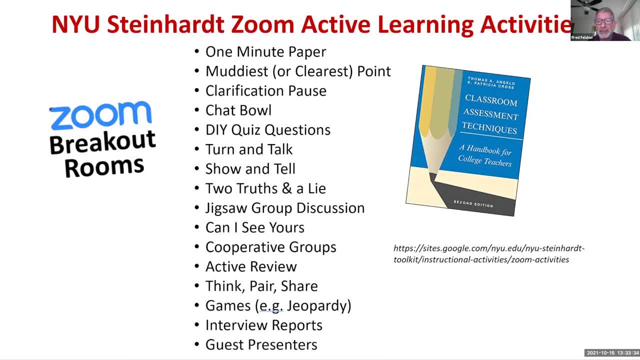 And then we're going to regroup as a whole class and do a share out, And I would do that in class and I do it online. And may I say one great thing that I've learned about pedagogy: That when you do this for 10 minutes, 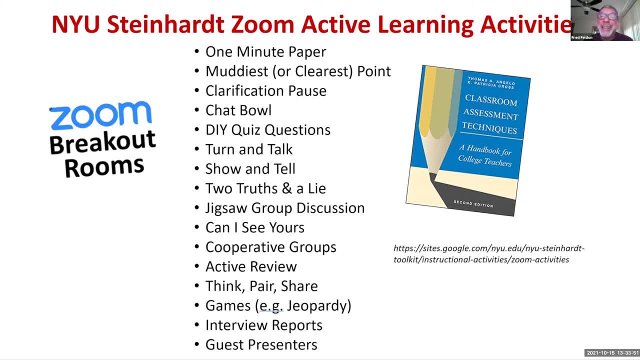 Do not check your email to know. but you can leave the room And if I'm teaching online, I will step away from the camera and out of my office. And I was talking about doing that with my dean Who said: wow, that's wonderful what you're doing. 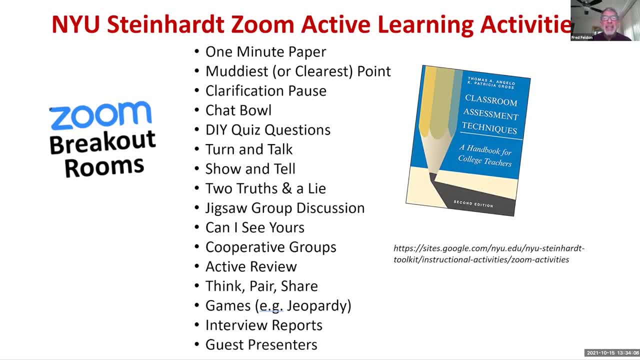 He had the description for it. You are removing the, the authoritarian in the room, and allowing students to be more free and open, have free and open discussion. So wow, Tom, Dr Neil, that's awesome. No wonder that's such a great practice. 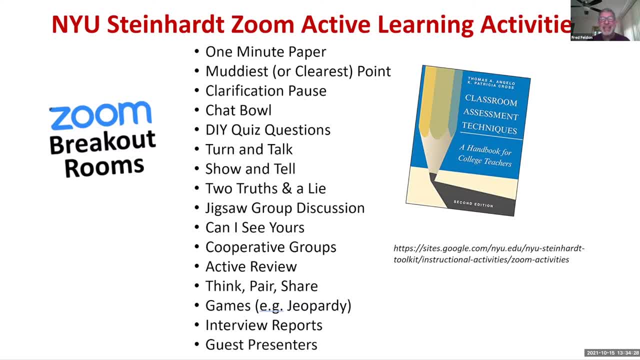 If you can leave the classroom or step away out of the office and yet the teaching continues, That's the sign of a great teacher and it also gives you a break. I mean I, I would leave the room and I'll go out and have a glass of wine with my wife. 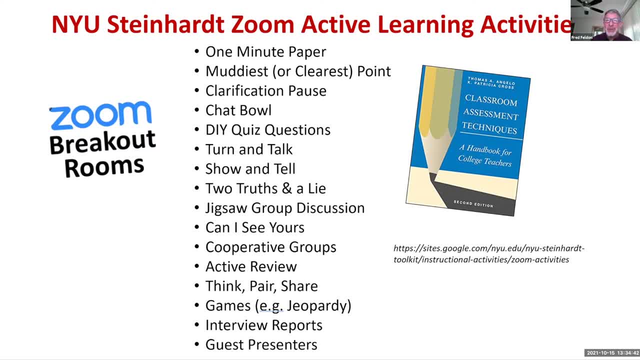 And I'll listen into the audio because the students can talk to hear and see each other and I will listen in through my open door to make sure the learning is going on. And if there's some other chat- low level chat- about you know, a beer they drank or a party they went to or a movie they saw, That's fine. 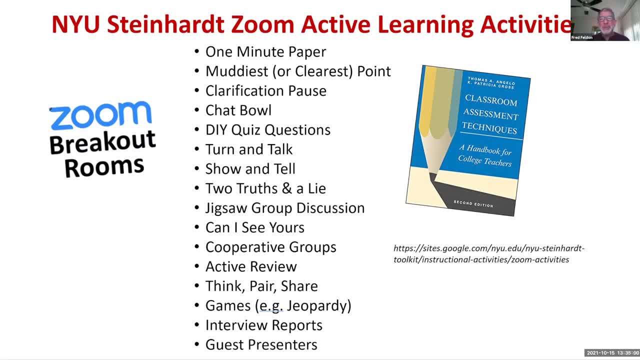 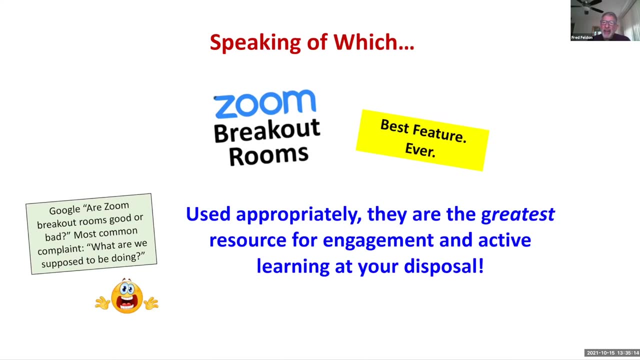 You know, our job is to foster community, So I don't expect 100% of the interaction to be disciplined based. I'm happy with that, So All right. Speaking of zoom breakout rooms, I did a little research on what students really feel about them. I just googled our zoom breakout rooms. good or bad? Oh boy. 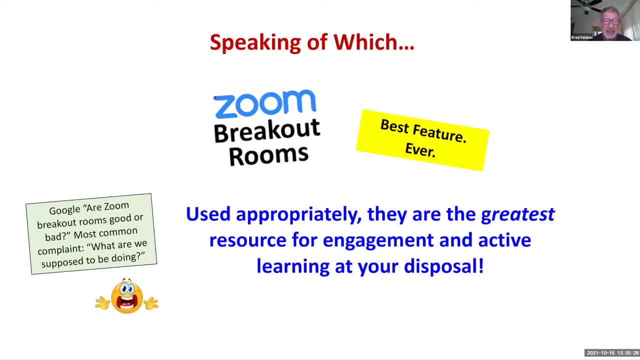 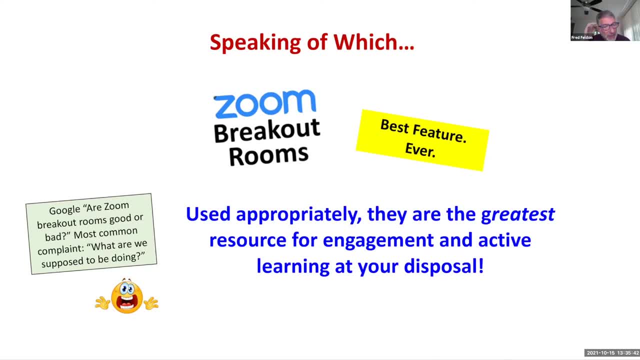 I can tell if they're allowed to use the green and the orange. I can tell if they're allowed to use the blue and And used it appropriately. I can. I can see What they might be thinking. So what I'm going to do is is have a little interactive activity. 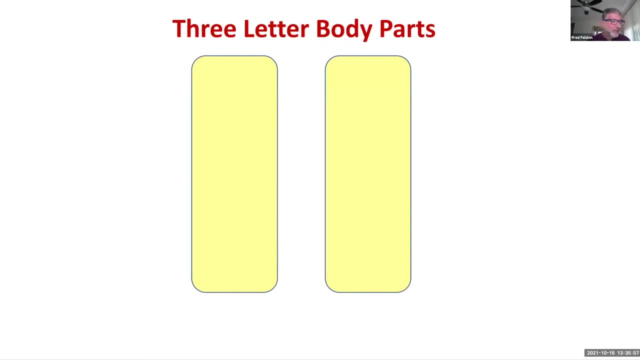 It's going to take, I don't know, five to six minutes or so, And don't worry, Cause it's not going to have anything to do with math. Could you use that? Because you may be holding what you write up to the webcam for your attendees, your fellow attendees, to see when I break you up into groups. 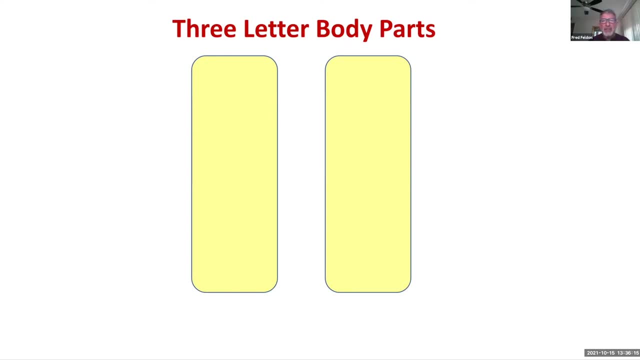 I'm going to give you one minute, starting now, Individually. no talking, no chat, no interaction. just quietly think to yourself. And, Fred, the cameras are disabled for everyone. Oh, OK, We can work with that. OK, we can, But I can still break them up into groups. 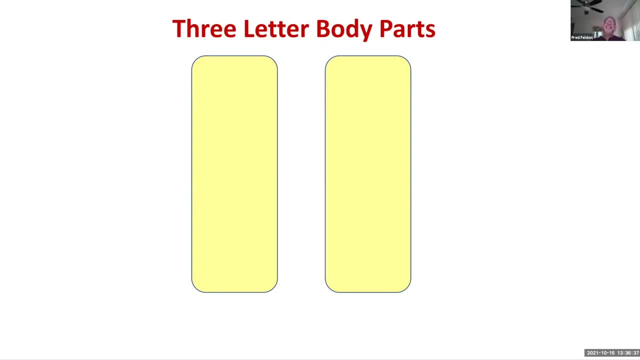 We don't have breakout rooms set up. Oh crap, I apologize about that, but we could break this. Or if you want them to type in the chat, or if I, we have 50.. So if I do my quick math calculation, 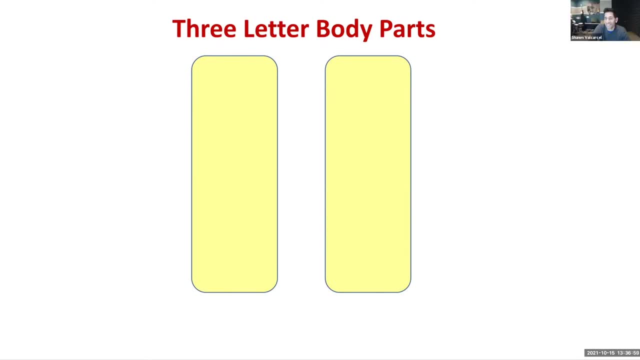 You know, I don't know if this is going to All right. All right, Here's what we do. Here's what we do, Do not? You can type in the chat, but do not hit enter until I give you the signal. 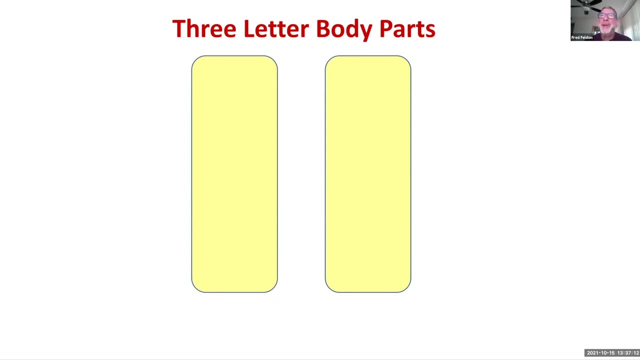 OK, and this is. this is so awkward because here I am trying to promote collaboration act online and we can't do it, But the workaround is. this will be somewhat similar. It won't be quite as effective, but do not hit. enter Type a three letter body. 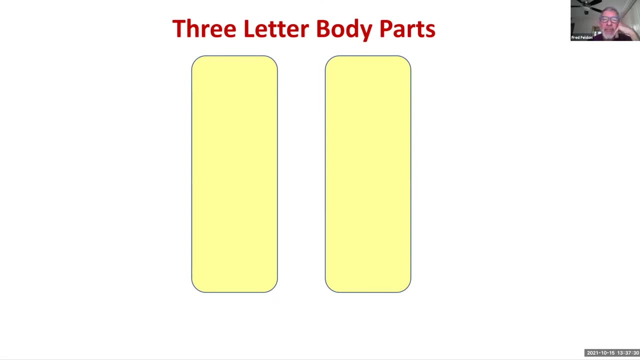 Part or as many as you can You can think of Into the chat, but do not hit enter until I give you the signal. OK, I'll give you a minute, starting now. I'll just pause. Give you 10 more seconds. 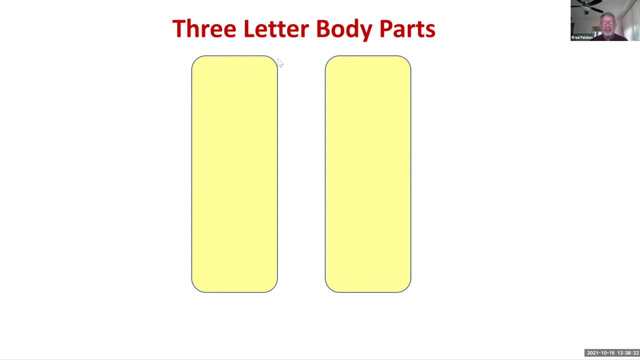 Now what's going to happen? Don't do it yet, But when I give you the signal, what's going to happen is you're going to see it. All these chat messages go down and Let's try it. Five, four, three. 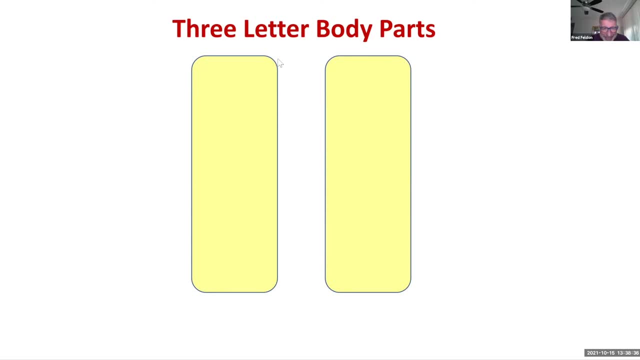 Two, one go, Hit enter. There they go. We are up to 30.. 30 chats. OK, I'm scrolling down and I see bunches of them. All right, Well, let me tell you the structure of what I was going to do. 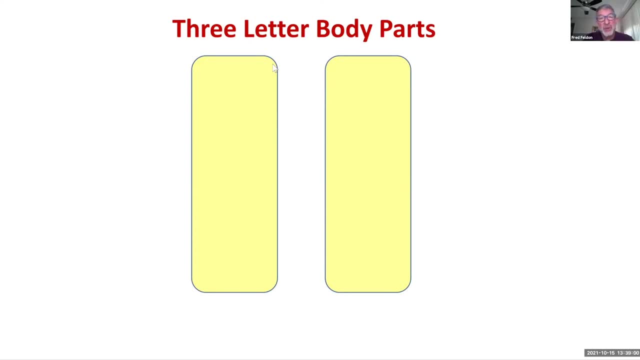 I was going to break you up into very small groups of just two. where you have a partner, That's it. And I was going to have you share, by holding up to the webcam or speaking out loud into your microphone, Your two letter, two letter, three letter body parts, and then have you combine them into one longer list. 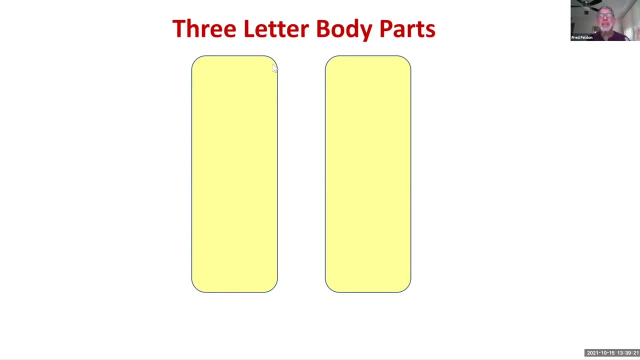 I was going to do that for maybe one minute And then I was going to break you up into a larger group of five, Five or six students people and have the five and six of you share your list by holding them up to the webcam or speaking into the microphone. 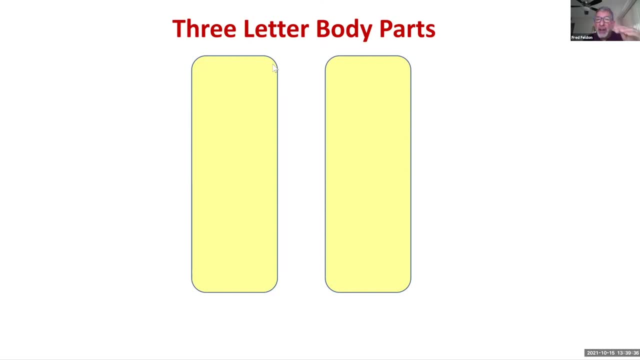 And having you compile a list which should be even longer still, And then we were going to do a whole class share out, which we're kind of doing right now. But the effect of that was- I may ask you what you think- 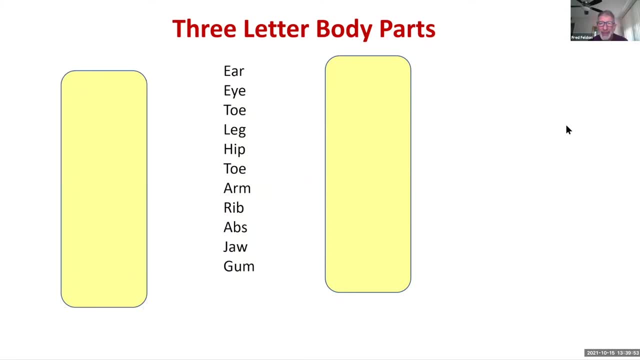 So I've done this several times And you may compare the chat with some of these that I've collected over the many times I've done this. So let me hear some comments. Unmute your microphone or type into the chat room. What do you guys think was the goal of this activity and how do you think it went? 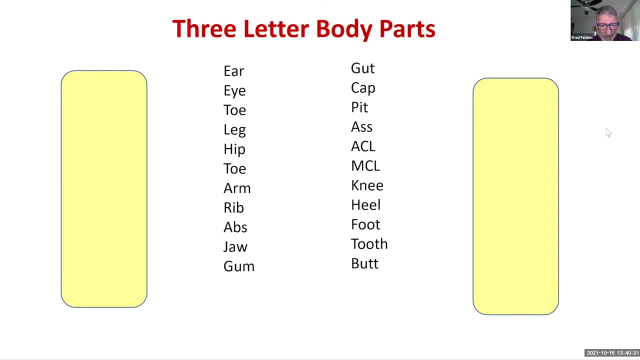 And would you? was it a good one? So we can have you. I can unmute you if you raise your hand. I know, Chow, you've had your hand up for Just a minute. Yeah, I'd love to hear some input from a participant or two. 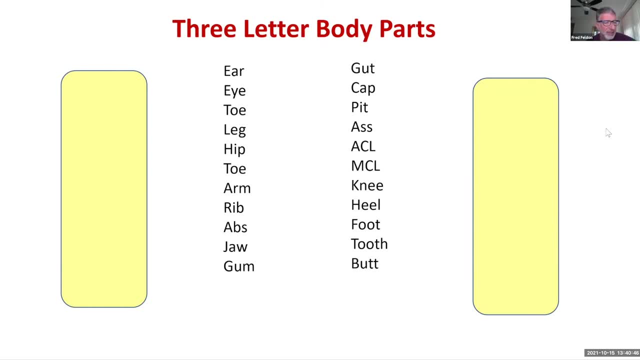 What do you think was the goal of this activity, and was it, did it work? Two participants have their hands raised, So let me go with Jennifer first. All right, Jennifer, so you're on Awesome. Well, I was thinking that one of the goals was to teach the students. 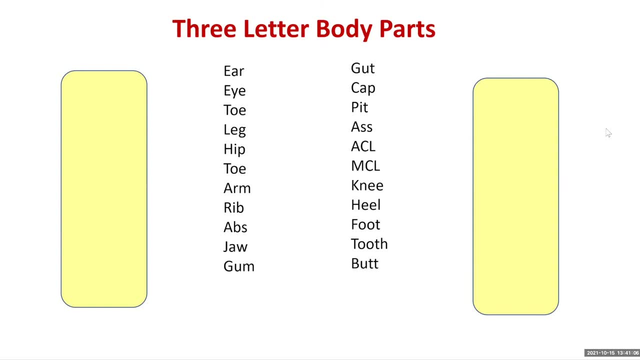 That they could learn from each other and that there was a lot of knowledge in the room that wasn't coming from you Also gave them the opportunity to see a clear path towards communication and sharing out of that information. Beautiful, I couldn't have said it better. 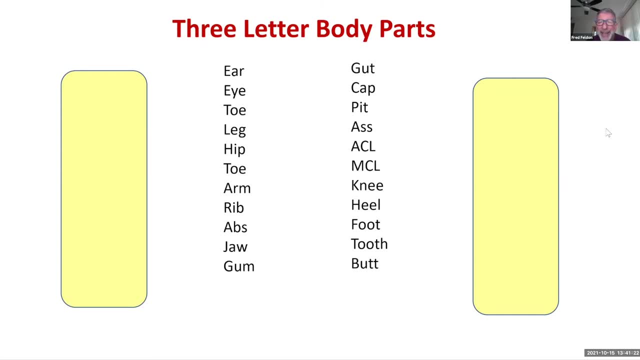 Jennifer. thank you Anybody else? Well, let me share a comment that I did. I did this last week, or was it two weeks ago, with Glendale, Glendale Community College. I had about 30 participants. It was a different presentation, but I included this activity. 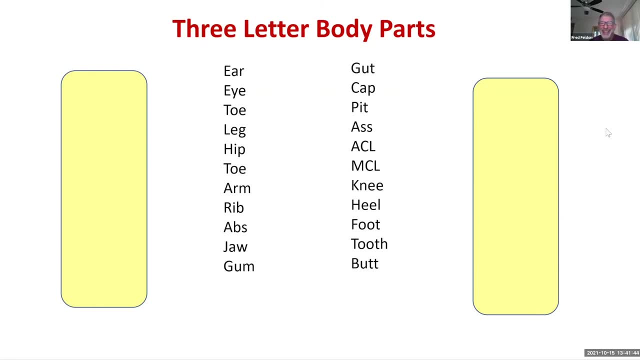 And when I asked for comments, you know what somebody said? Yeah, I don't. I think somebody doesn't know how to spell, So we had to have a discussion. you know what were the rules? You didn't tell me the rules, dude. 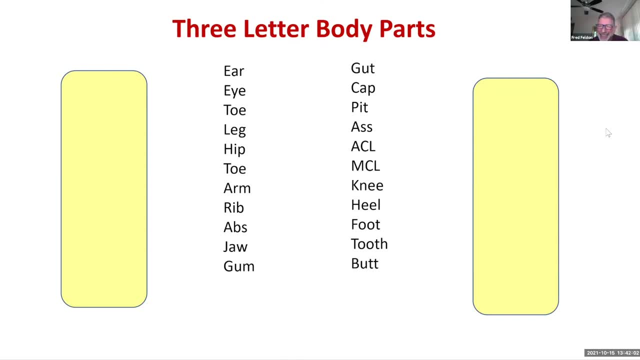 You didn't say we could use the same letter twice. You didn't say we, you know, you know? I mean it was just a funny discussion. I thought it was. Let me get Chao now, because she does Okay. 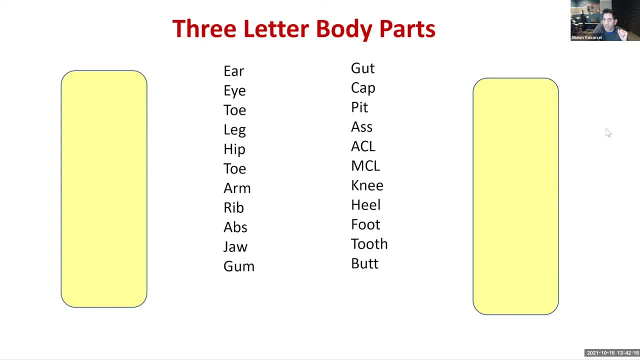 So, Chao I, I unmuted you now I think I did Okay. Can you hear me now? Yes, Yes, Thank you. Yes, Okay, I have. I raised my hand when Fred mentioned about extra credit. Okay, 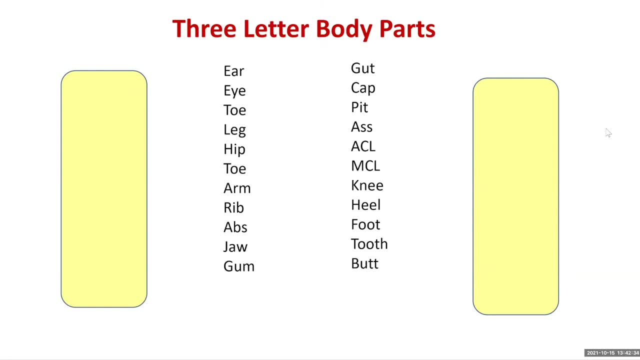 My first question is Yeah, What is the percentage of extra credit? Because now we are facing with the situation that we have many students come from high school And we see the assessment now is one of the regular question, because we have many students come from high school. 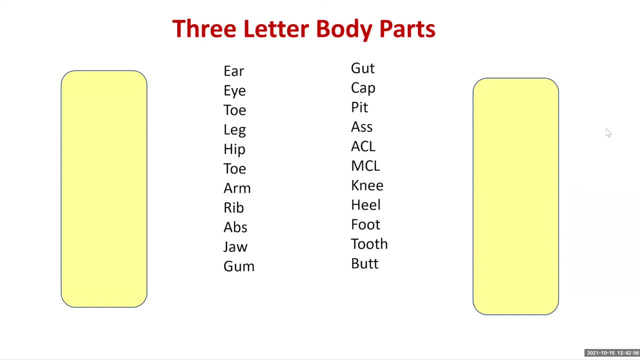 They said that, okay, they come to the class and with the extra credit, that will be enough for them to pass the class. Correct, Good question. And I, I do Get asked that and it's you know my answer is not much. it's not worth very much, to be honest with you. 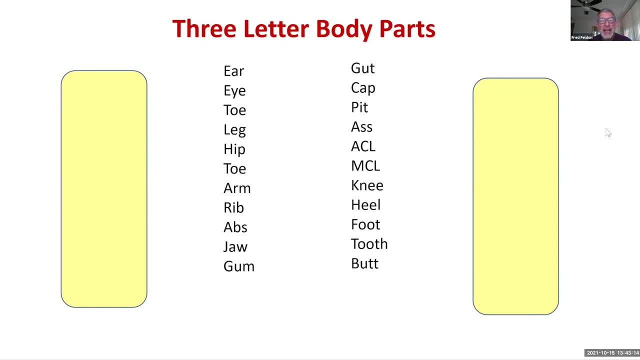 And I tell them that the reason I do it is for fun. I add a fun, I incorporate the real world because I'll take a. I'll take like a Superbowl game or a tennis match or a baseball game and, and you know, like somebody's Jersey number or a score or the Superbowl 53.. 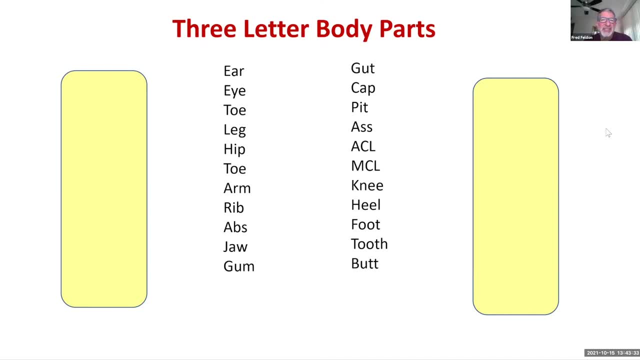 And what's interesting about the number 53. It's kind of just extra credit. So the price, the cost, theства that the people who come through is usually just fun shit, Right, I mean stuff, fun stuff. And I say, however, I do want to reward you for participating in this extra credit. 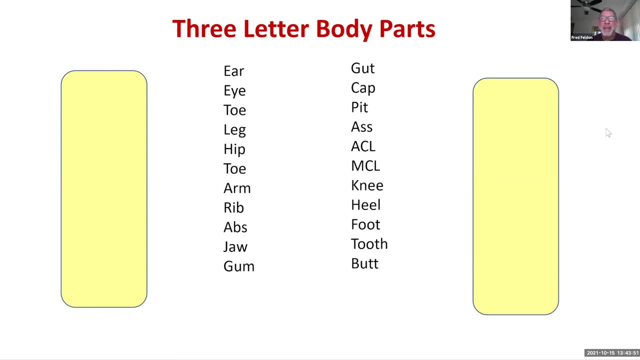 Unfortunately, the Pearson, my lab, does not have a field for extra credit. I tell them it may have by now, but I tell them it doesn't, And so what I'm going to do is add points to your participation score at the end of the semester. 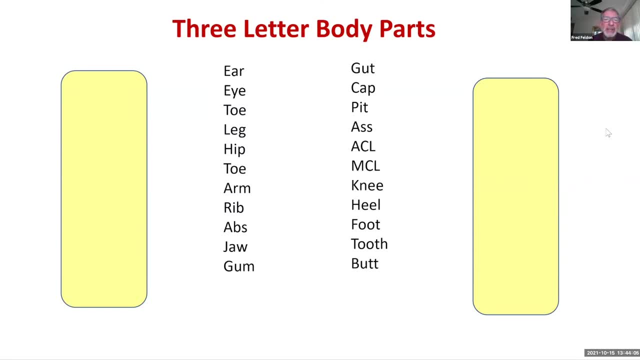 cured marriage. Yes, No, sir. your overall average is 89.9 percent, or 89.8 percent close to the next highest grade. i will use your extra credit activities to push you up to the higher grade and child they seem happy with. 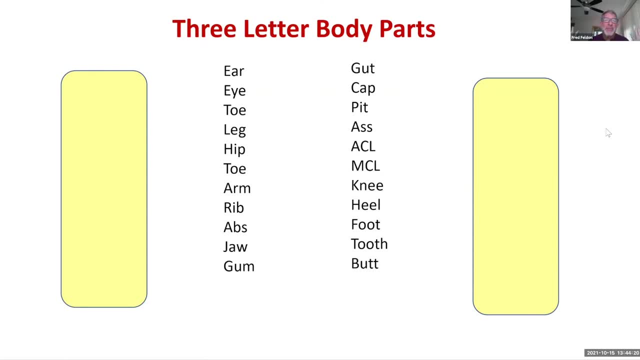 that. so the whole semester they never know how much their extra credit is worth. but it's just a fun. it's just adds fun to the class and i do use it to help decide if a student is right between two grades. okay, so i hope that answers your question. thank you very much. i have another one. 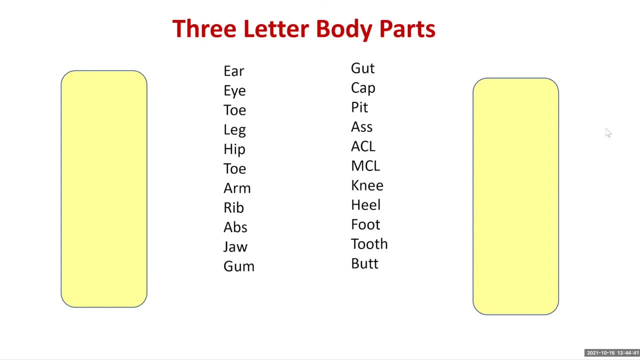 thank you very much, fred. always, always, i do appreciate your opinion of technology and you see that now i use a padlet. the padlet is one very, very powerful tool for student engagement and i think that we we need to mention that padlet. yes, yes, i am aware of it. i haven't. i've heard of it, i've watched youtube videos on it and i 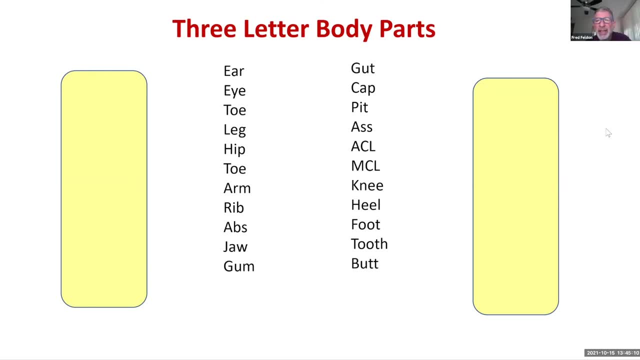 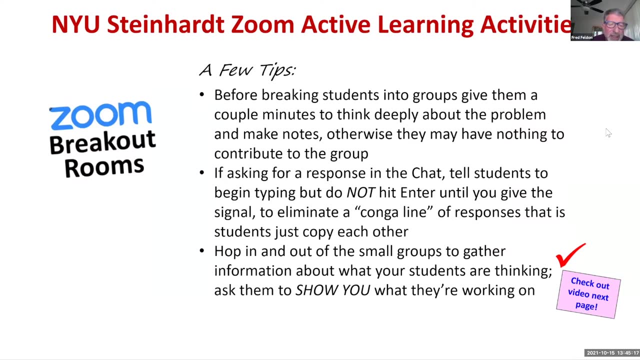 i'm i, it's on my list of things to try. i i agree, i've heard of it, thank you, thank you, all right, let me uh before we leave. zoom, uh, i've got a couple more slides. um, the first bullet point says i would not throw students directly into. 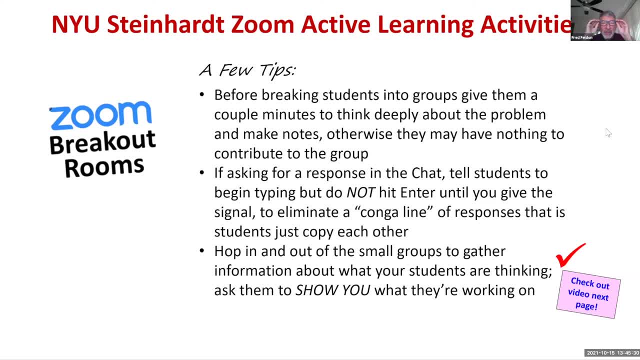 a breakout group. in fact, i even did that today. if you'll notice, i had you spend a minute or two just thinking quietly by yourself to add something to your list of body parts, and i would do that with a math activity or whatever. i would have them think carefully. 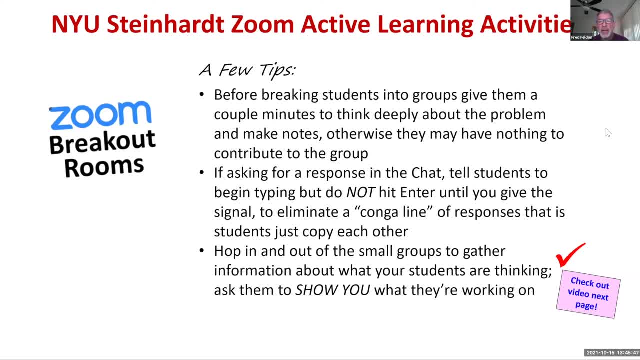 for a couple minutes alone, quietly, before you break them up into groups. it's part of a japanese learning technique called think pair share, where you give students a problem and the first part is to just think quietly by yourself, no talking, no interaction. and then the pair part is where you have students turn to their left or their right or front of them. 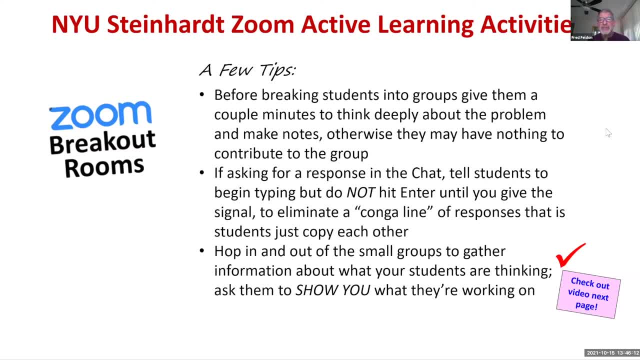 and behind them and work with a partner and look at your answers, compare your answers if they're different. you need to go through each other's work, convince someone else that your answer is right, and then the share part is: i call on us on a volunteer, and i say volunteer in quotes. 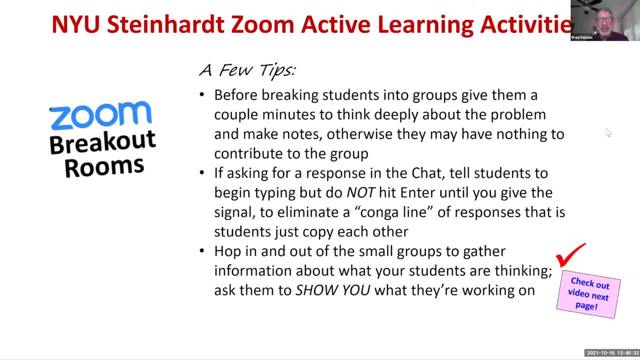 because i very carefully spread the participation out equally among the class. i really don't ask for volunteers because you know if you do that it's always the same group of students and so i would not call on a volunteer without a think. pair share activity first. if you call on somebody cold, that can be very distressing. 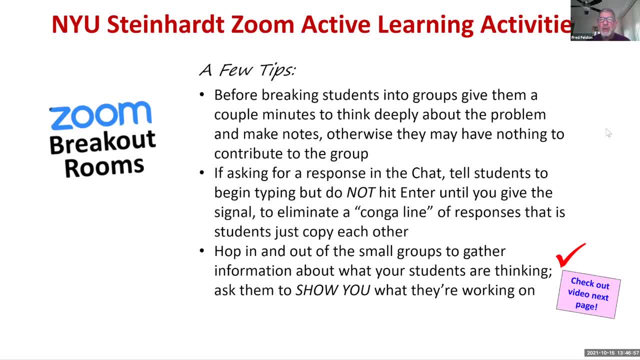 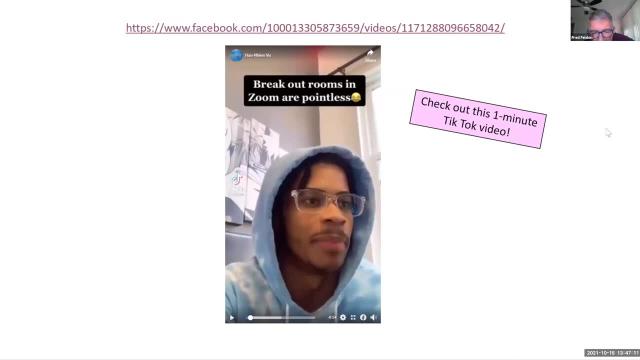 and it won't work. so i will call on students at random, but only after they've had a chance to discuss the problem and in their groups. all right, what i'm going to try to do now is is share this one minute video with you. so what i have to do? okay, here it goes one minute. 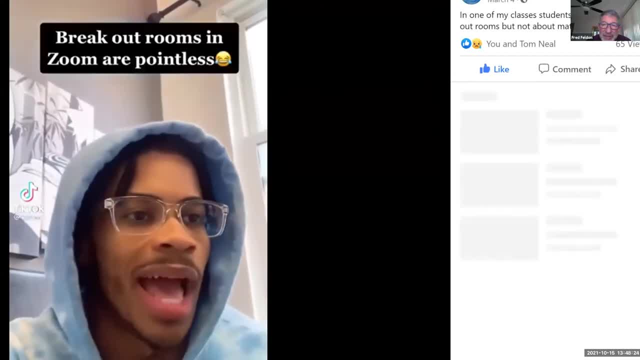 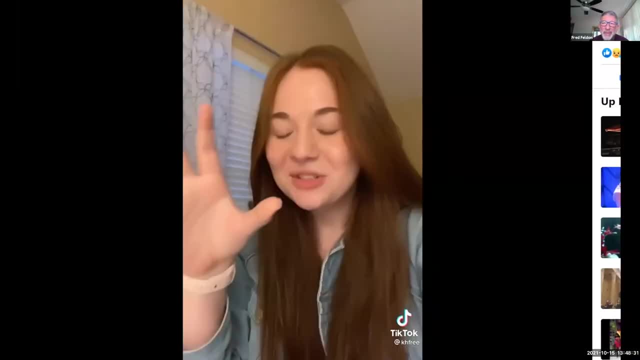 bro, teachers really be thinking that we actually talk to each other when they put us in breakout rooms. the amazing thing is that teachers do this too. this whole year i've been a student teacher in a first grade classroom. during those teacher work weeks before the kids come home, i'm actually 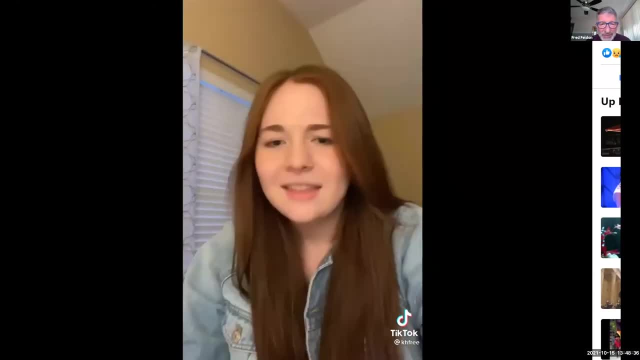 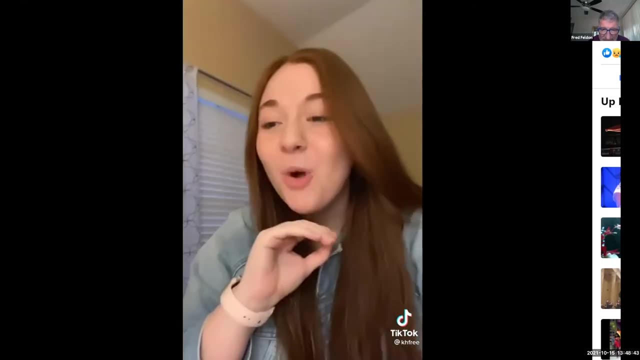 kids started school. there were a lot of Zoom meetings. This one meeting, held by the district, put all of the faculty into breakout rooms so we could further discuss. whatever the meeting was about, No one was saying a word. I looked at my mentor teacher and I was like we're not actually. 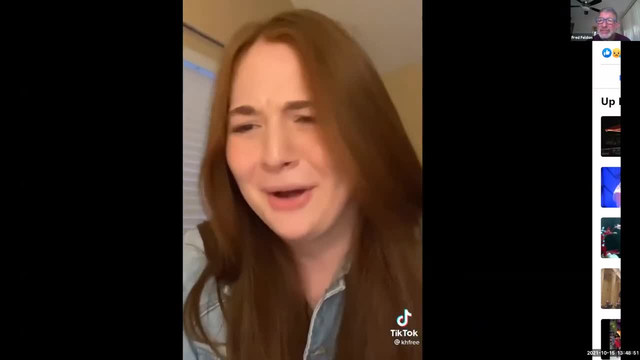 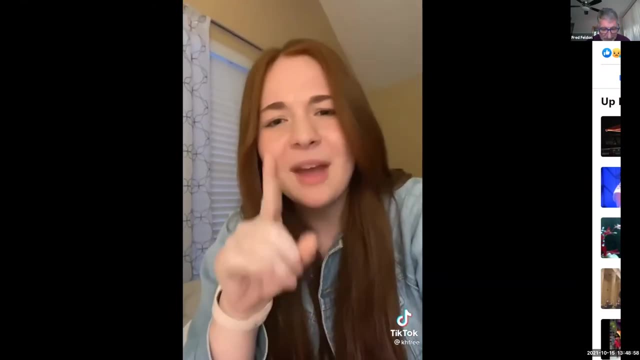 going to discuss anything in this breakout room, right, And she just goes. no, Of course the district people were hopping from breakout room to breakout room to listen to our discussions. District person hops into our breakout room and, without missing a beat, one of the fifth grade. 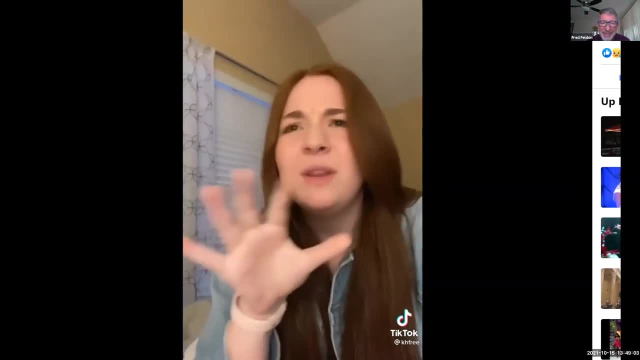 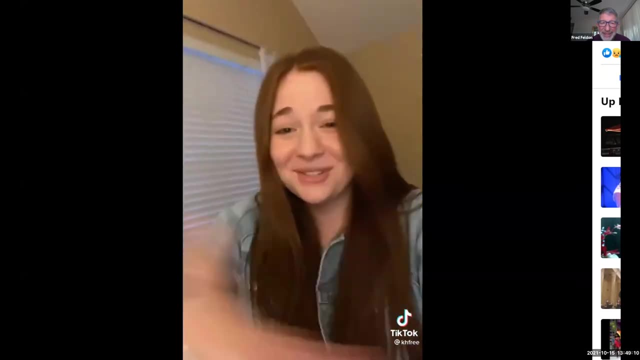 teachers just says: all right, does anybody else have anything to add? or do we think we've pretty much covered it? Every teacher in the breakout room unmuted themselves and was just like: no, that was really good, really valid points. So the district lady left and that same fifth grade. 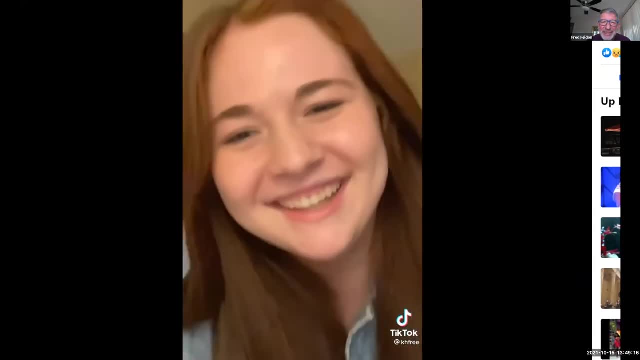 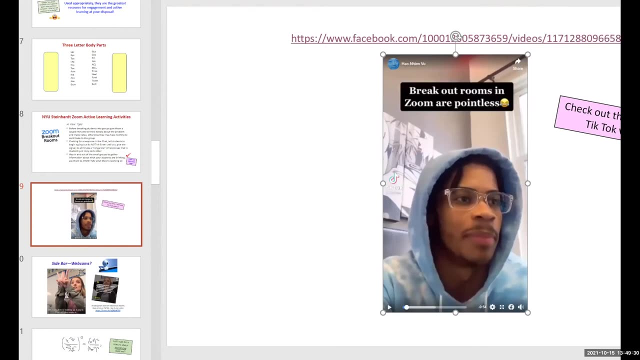 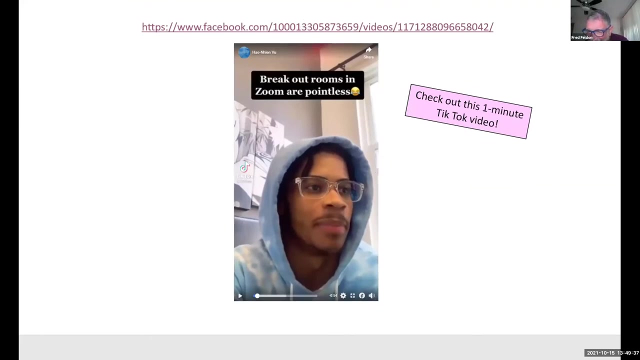 teacher. as soon as she left. he just went- oh good, she's gone, And we went back to doing nothing. Did that work? Yes, it did. Yeah, Awesome, It was great, Isn't that cool? Oh gosh, a lot of people agreeing here in the chat. 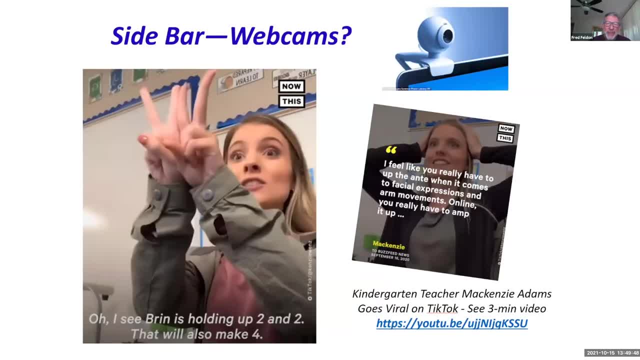 Awesome, All right. So enough about Zoom and breakout rooms. Let's talk about webcams. It is controversial. I was involved for about two weeks with a Twitter war about a group of college professors over the use of webcams And I kind of gave them an argument that I used with my tutor as part of AB 705,. 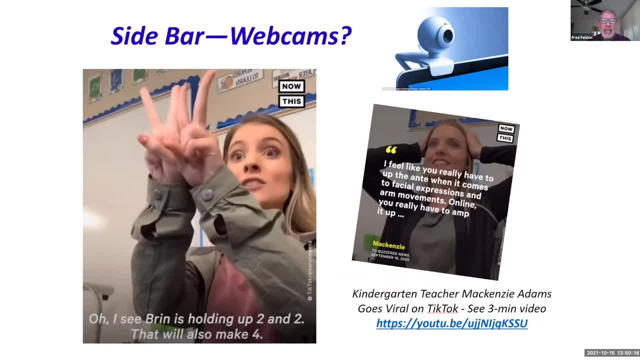 our college instituted class tutors And I had one who joined a college algebra class that I was teaching online And before he met with students he wanted to confirm that he was not going to use his webcam. And I said I'd prefer you do use your webcam, because let me ask you a 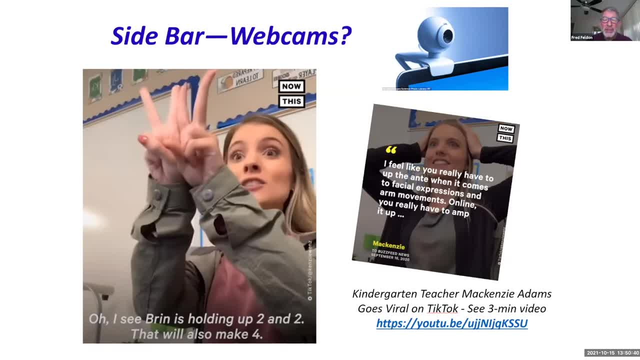 question. And he said: when you meet with students to tutor face-to-face, do you put a bag over your head? Kind of harsh, right? But he said: yeah, you're right, Fred, Okay, I'll share my webcam. And he: 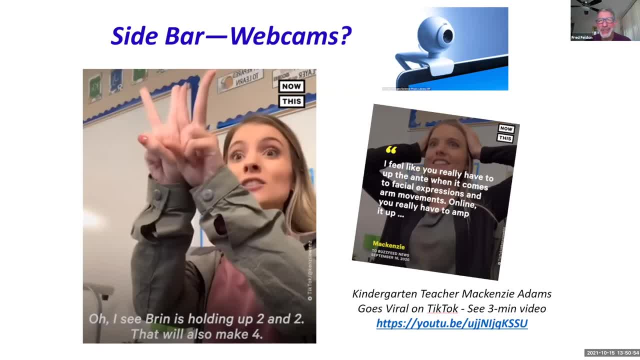 did, It was not a problem. So I kind of used that in this Twitter war. I said: when students enter into your classroom, do you have them put a bag over your face? Oh boy, that heated. That heated up a lot of debate And they said: of course not. But let me ask you this: Do you make the 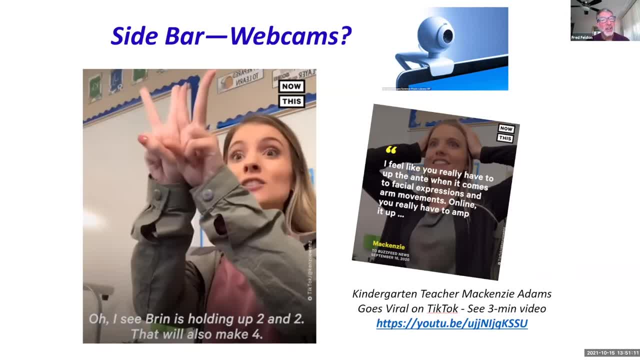 students wear a mask, Do you let them strap a mirror to their forehead? Because it turns out seeing yourself in a Zoom meeting is a known disability. I don't remember the name of it, but it can stress people out seeing themselves if their webcam is turned on. And, of course, 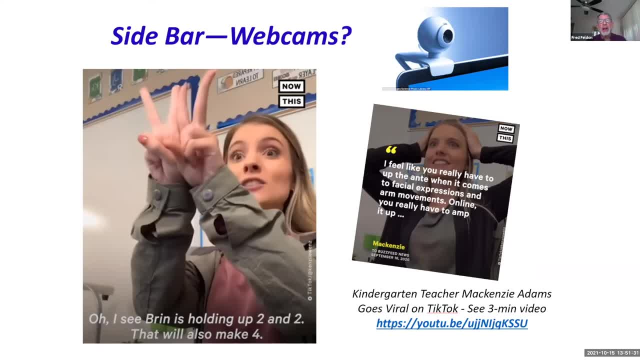 my argument for that was: well, Zoom has a feature where you can turn off your own webcam. I mean your own video. You can allow your professor and classmates to still see your video, but you yourself are not distracted by it. And, of course, the other argument was background. I don't want to share my 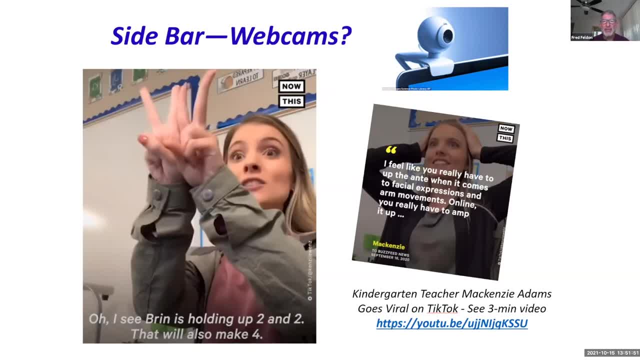 house or my private space, And well, you can have a virtual background. And then the counter effect of that is: well, not every student has the technical expertise to create a virtual bag. And it just went on and on and on. And then the state chancellor's office chimed in with their rules, as 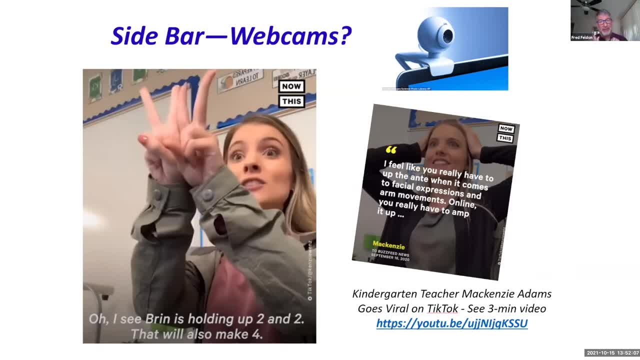 the controversy expanded. I believe I follow the state chancellor's memo which said you should discourage the use of webcams unless it's vitally important to your educational integrity and the effectiveness of your teaching. And the second thing you need is you need to give them an opt-out. And the third: 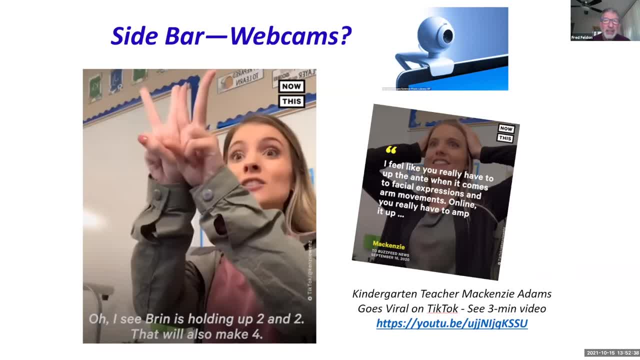 thing you need is to let them know in advance when you will do that, And that's what I'm trying to do. So that's what I do At the very beginning of the semester. I say we're going to have five asynchronous Zoom meetings And I tell them the dates and the times. And because I want to, 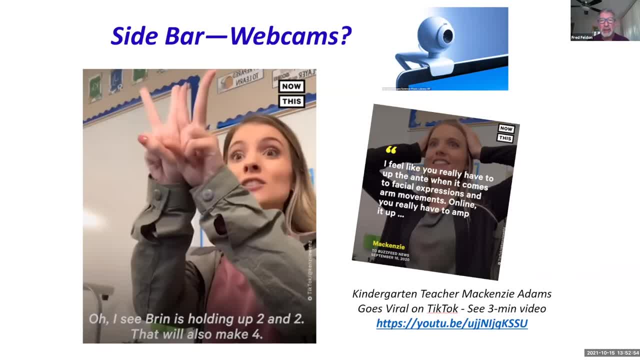 authenticate who is attending those meetings. I will ask for microphones and webcams to be turned on. If there's a conflict and you can't attend the meeting, you can watch the recording. You can post a short summary of the meeting to receive your full participation. 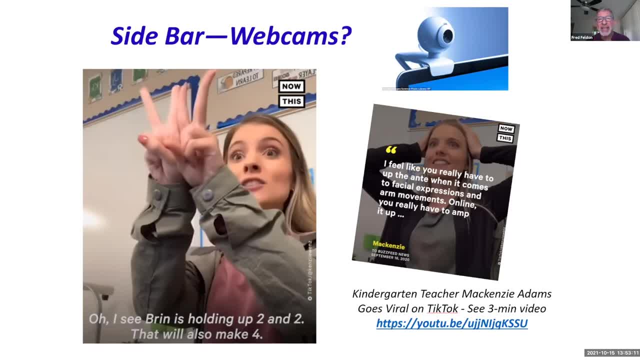 And I'm on them. If a few days go by after the meeting and they haven't posted their report, I proactively reach out to all those students with an email, a direct email. hey, I noticed, you haven't. you didn't. you did not attend the meeting live and you did not watch the recording and post your report. 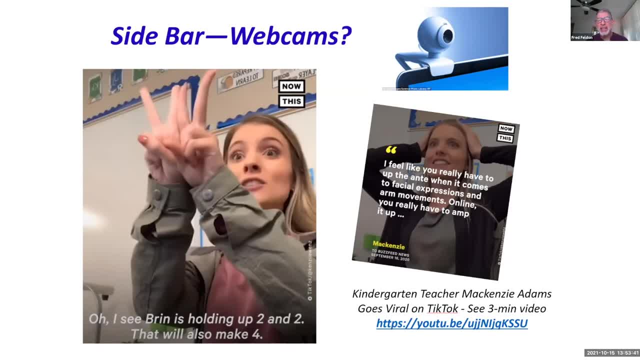 I'm on them. If a few days go by after the meeting and you don't watch the recording- and you didn't, you didn't, you did not attend the meeting live and you did not post your short summary, the material presented and the discussion that took place was valuable and you will also get a zero for participation points for this meeting. Don't let that happen. There's no time limit. Just as soon as you can- the sooner the better- Go ahead, watch the recording and post your short summary, and that seems to be working. 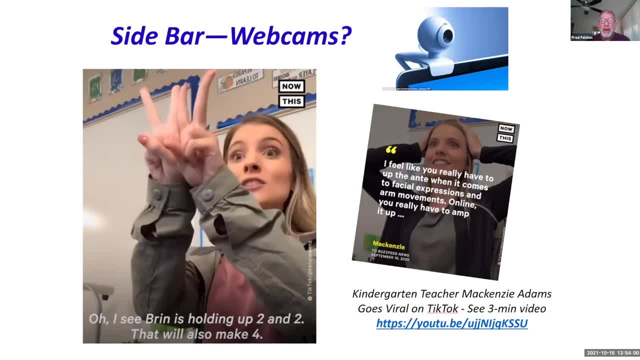 I don't know if you watched the Biden acceptance when he became president, but they featured this kindergarten teacher. I'm on them, mackenzie adams. she was doing tiktok videos of her zoom meetings with her kindergarten students. she's freaking awesome you've got. i'm not going to take the three minutes to do that now. 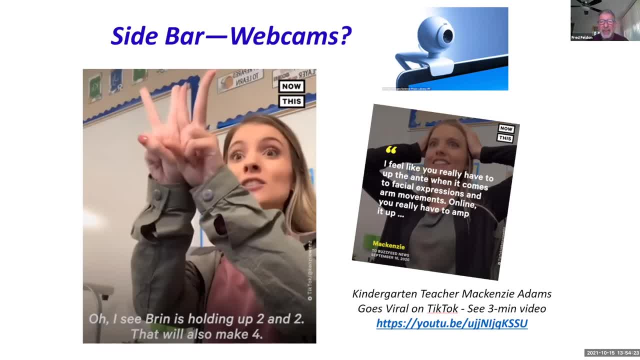 uh, we're running short on time, but follow that link. look what she does with her kindergartners. she has them make turtle faces, she has them hold up uh, uh signs- you know that- with smiley faces. and she does it all with webcams. don't be afraid to use your webcam and encourage the use of it. 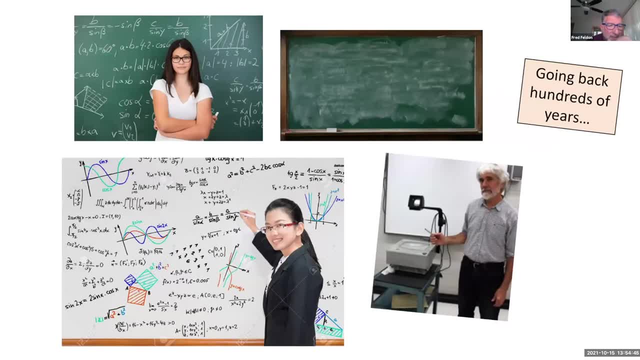 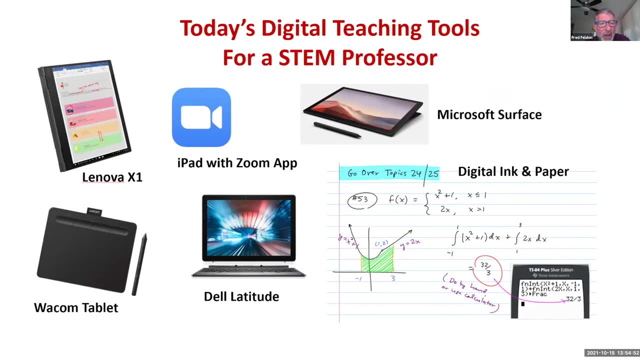 and then, speaking of notation, um, you know, historically we had chalkboards and overhead projectors and white and white smart whiteboards. now we have great technology. i myself use a microsoft surface book three. it's got a huge 15 inch screen and a stylus. i love it. uh, there's. 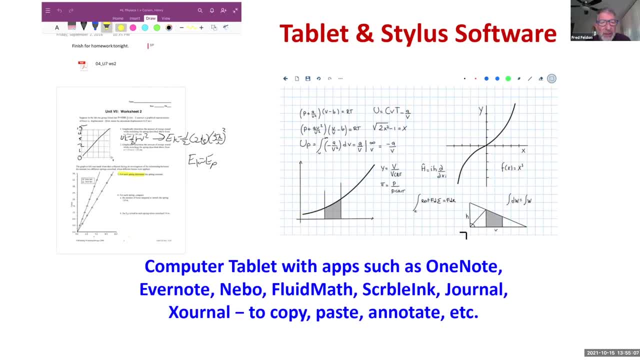 great technology. i myself use a microsoft surface book three. it's got a huge 15 inch screen and a software that we as professors can use. your school may provide site licenses. if they don't get equipment and software, pay for it out of your own pocket. it'll last many years. it'll be well. 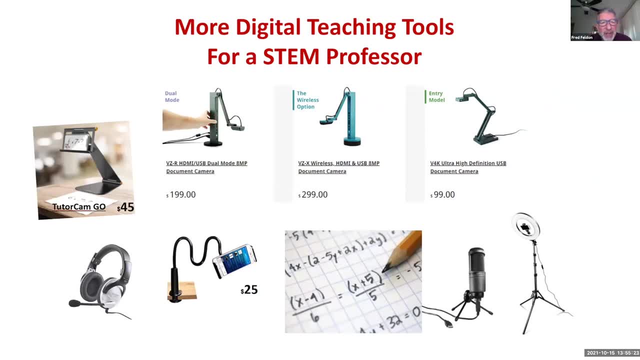 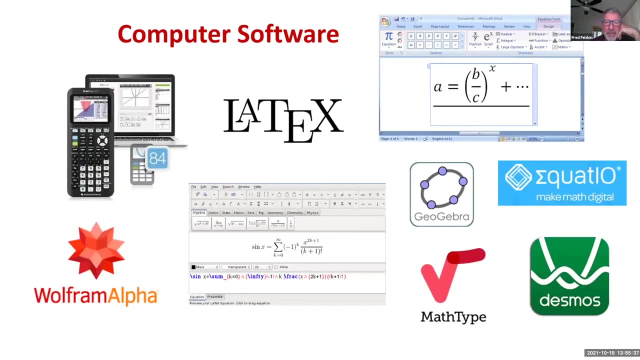 worth it and if you need to, you know if your budget's tight. that little uh camera you see at the top left of your screen for forty five dollars. it's so cool. it folds flat and fits into your briefcase or your backpack- really cool. your school probably has site licenses for some of. 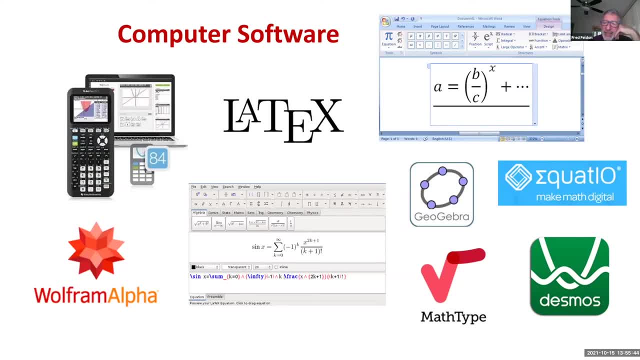 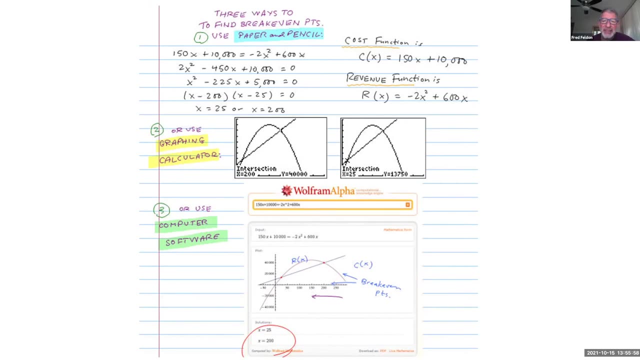 these programs if not pay for it out of your own pocket. i i'm not advising you to spend hard-earned money that you can't afford, but leverage your school, because then you can do things like this in the classroom and online calculator. screen grabs highlights, uh, underlining: um, it's amazing. 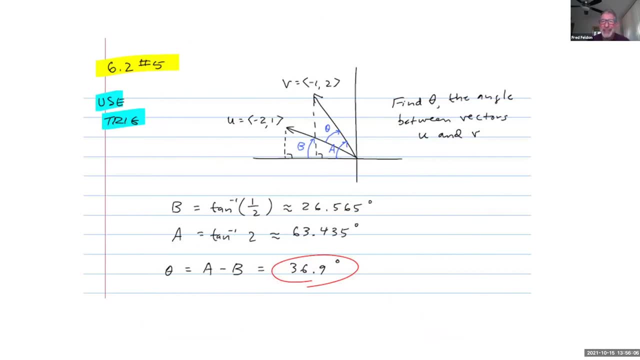 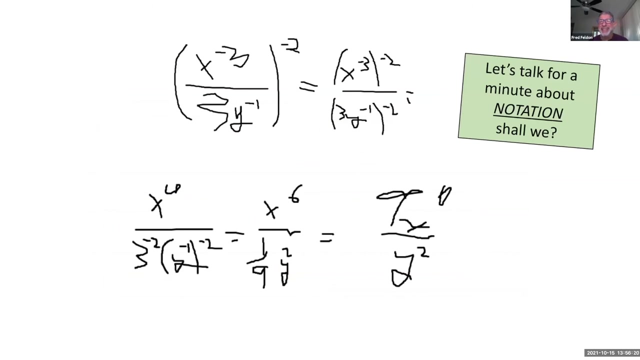 you know you can't do this on a keyboard. look at that. could you do that on a keyboard? and you can't. you can't really do it on a digital whiteboard either. digital whiteboards look like this and at least from your students point of view. so you've got to get yourself some tools. 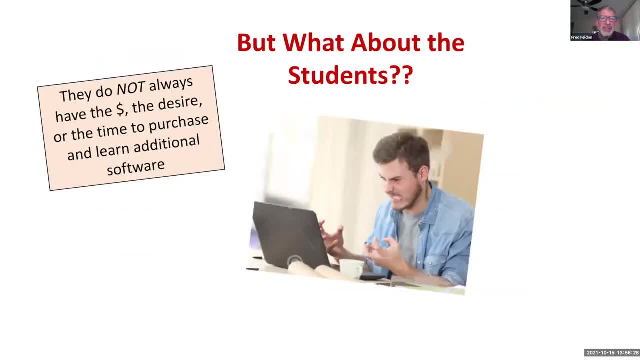 and then let's talk about what the students can do. they may not, as i mentioned, they may not have deep enough pockets where the desire or time to learn additional software. so i probably spent a year seriously asking all my colleagues all across the country: what do you do? how do you get the students to communicate? 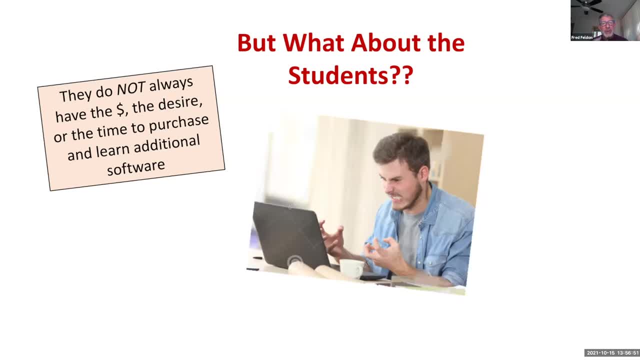 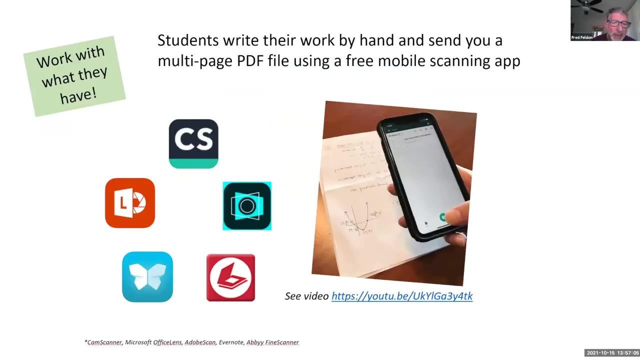 mathematically with each other and they were doing things like zoom whiteboards and jam boards and padlets, and i just was not happy with how that looked. so i i've come up with a couple three solutions. the first is to use a free multi-page pdf mobile scanning app. 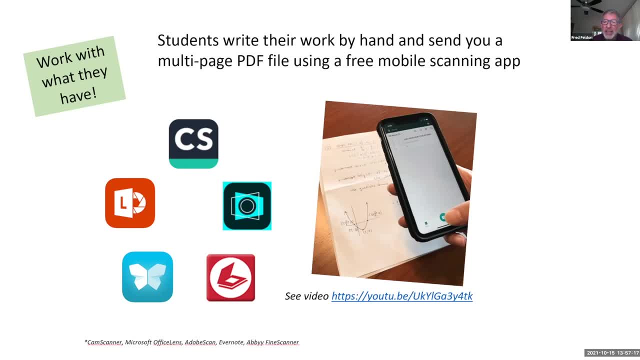 like the one i use is cam scanner, and i can tell you how freaking amazing this app is. in fact, i have a hp printer slash scanner- you know slash fax machine- in my home office. i have not used the scanner for two years because cam is a really good app and it's a really great app and it's a really 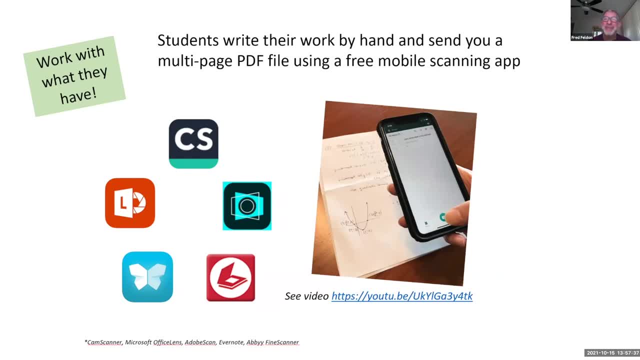 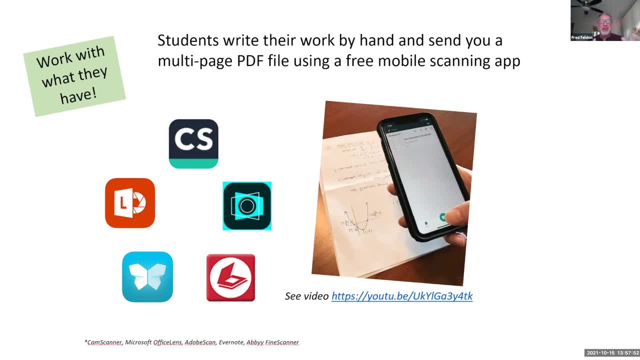 folded, you can erase shadows if, if you know you're leaning over it and there's a shadow, you can enhance the black and white contrast. ah, and it's free. so i i've created on youtube a few five minute videos to show students how to use this. i think there's a link showing on your 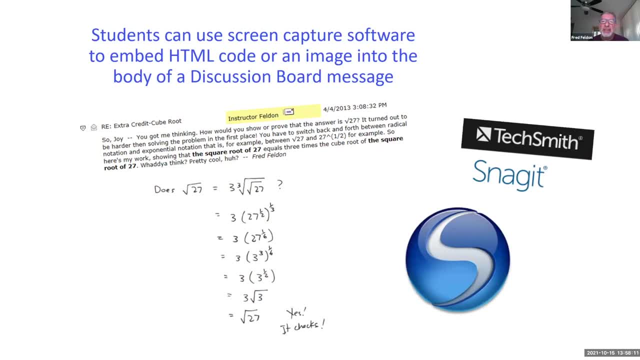 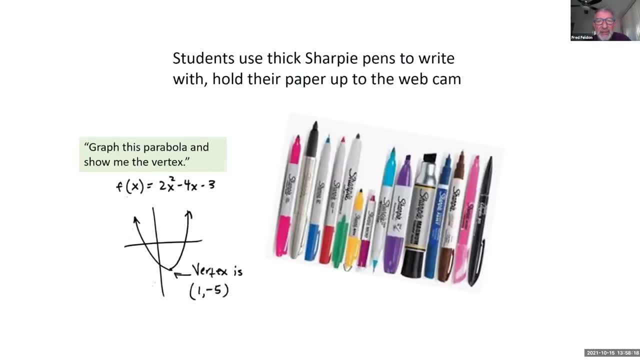 screen. the other thing you can do is ask students for a way to embed html code onto the clipboard, and you can do that. and finally, my most genius low-tech solution is to get a thick sharpie. a regular pen or pencil won't work. get a thick sharpie, write on paper and hold it up to your. 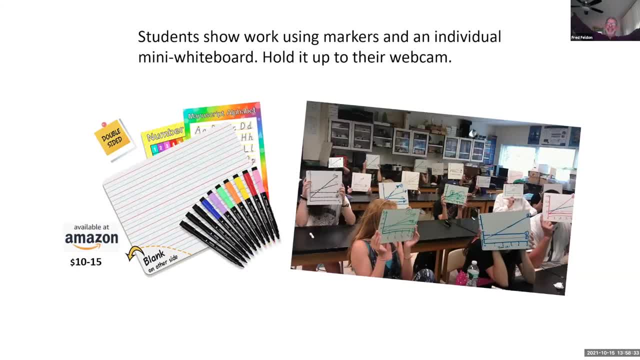 webcam you and another solution, and yet there's more. on amazon your students can spend a few bucks and and get a little handy package of mini whiteboards and pens and erasers and you know how some of you have probably done in the classroom or use the professor. you stand up in the front of the room. 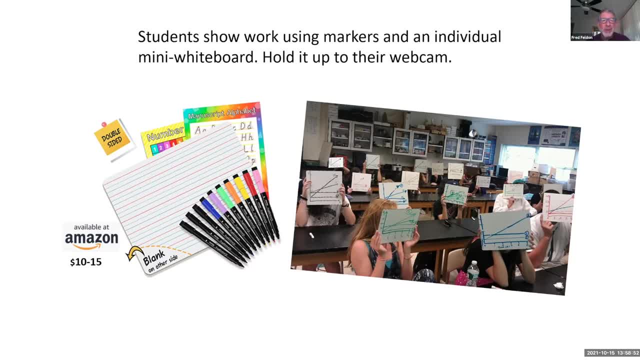 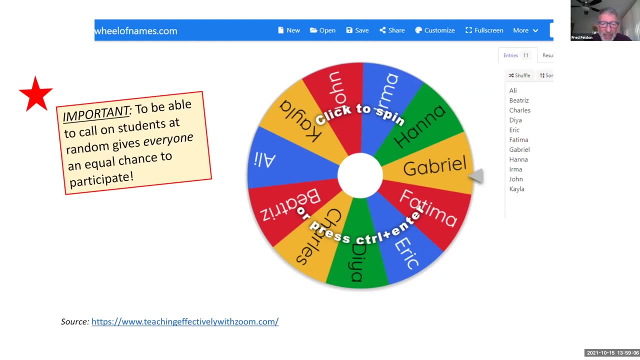 and students hold up their mini whiteboard. we'll have them hold it up to their webcam. okay, i'm gonna skip a couple slides. they are just basically other professors who have used breakout rooms successfully and they're all at this website called teaching effectively with zoomcom. 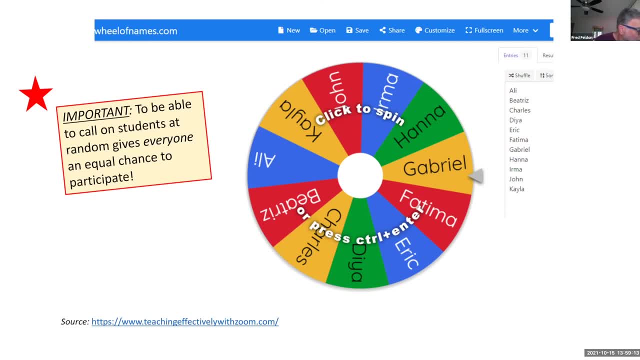 and one of the amazing things i got from it was a way to be able to call on students at random: the wheel of names. i used to be able to, i used to, i used to use my graphing calculator to generate, or i used to use google to generate a random number based on their position on the roster in the 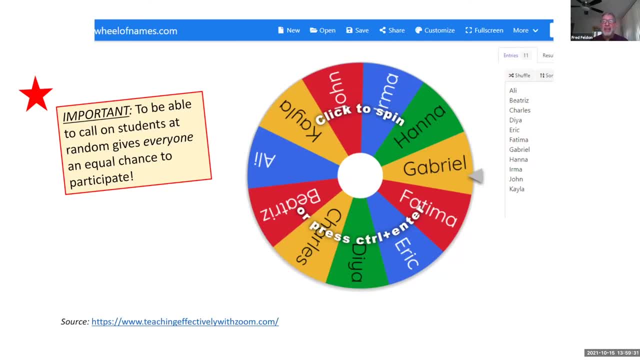 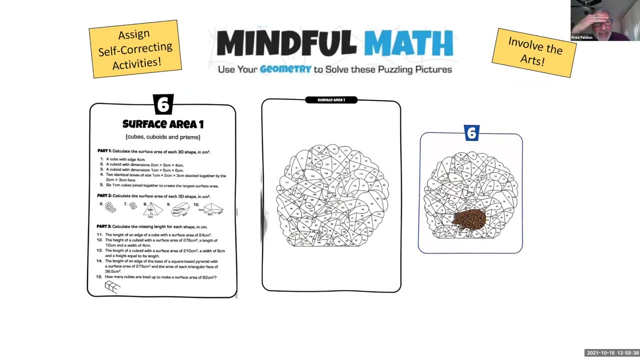 classroom to call on students at random. but this is a cool way: you click it, the wheel spins around, you type in the student's name and it picks on someone at random. a few more slides, because i know my time is running out, to increase equity. involved the arts: 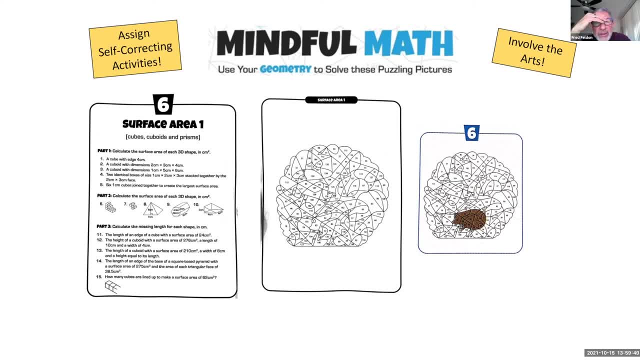 pass out or email self-correcting activities. rectangle recognize blank. when, when someone display displays an and ability to understand the room that people live in, putting jobs in as long as possible. remember when, the moments you live in those times, because the school or the day thingsош. 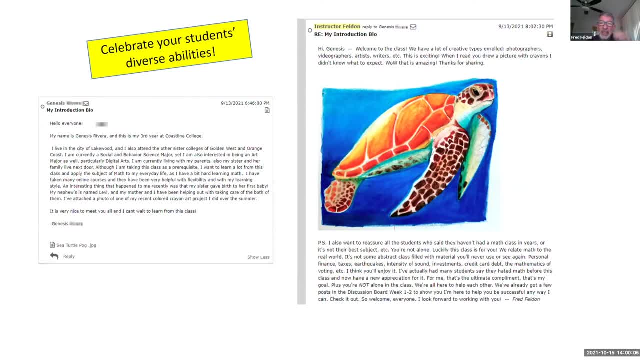 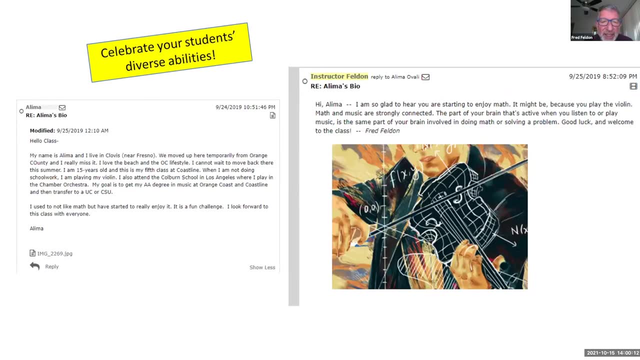 ability other than math in your class. someone posted this in their student intro. another one: hey, sean. speaking of music, this student was a music major and always struggled with math. she said it's starting to come to her now. so i pointed out the relation between the brain and and music and math. there is a connection. 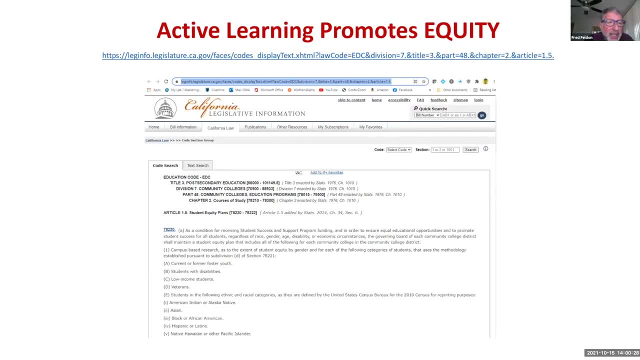 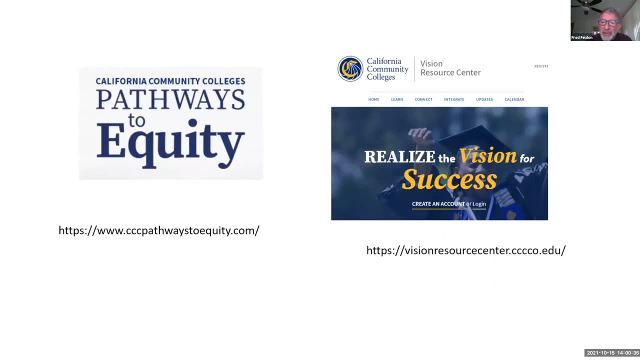 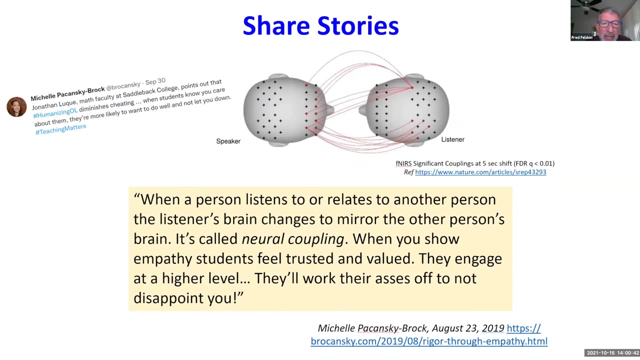 activity and engagement promotes equity. there's the actual legislative code and there are some great articles at the cvc and the chancellor's office website, and one of the people i recommend you follow on social media is michelle pakansky brock, who said that if you get students to 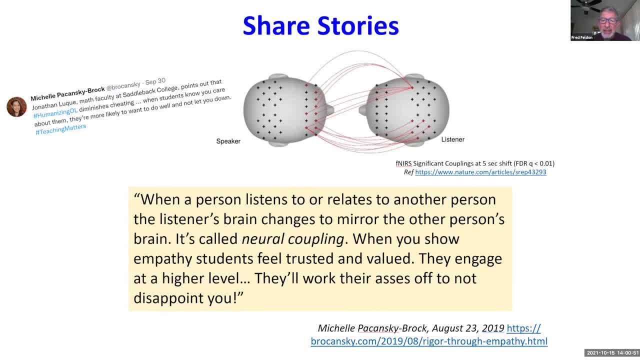 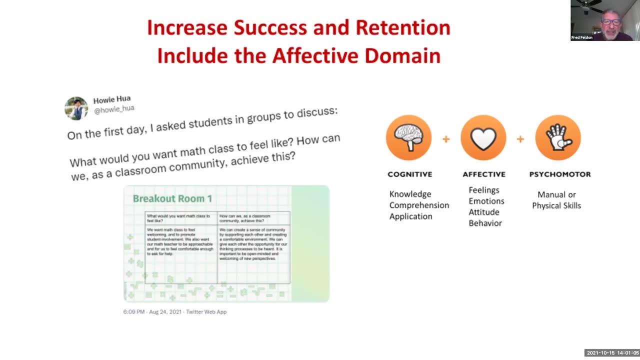 talk to each other. there's a scientific phenomenon that will change their, their behavior and their their brain neurologically. so that was cool, i thought. another mentor of mine that i follow is howie wah. he's a math ed professor at fresno state, and if you follow him on twitter, 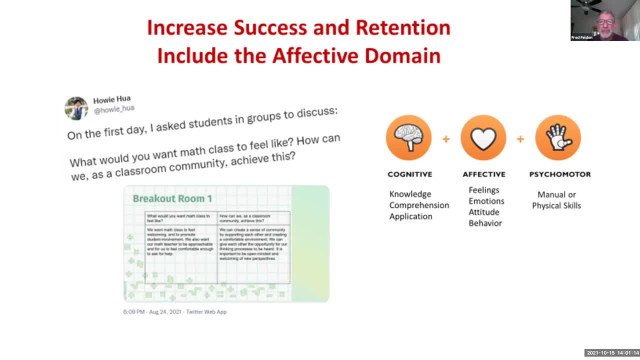 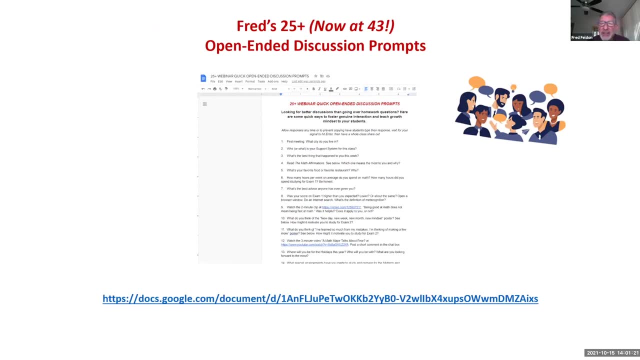 every few days, you will get an awesome hot tip that relates to the effective domain, which is important to include. i myself have a link to some prompts that i've been collecting. i'm up to over 40 right now. these are really, really quick. i just do one of these every time we have a 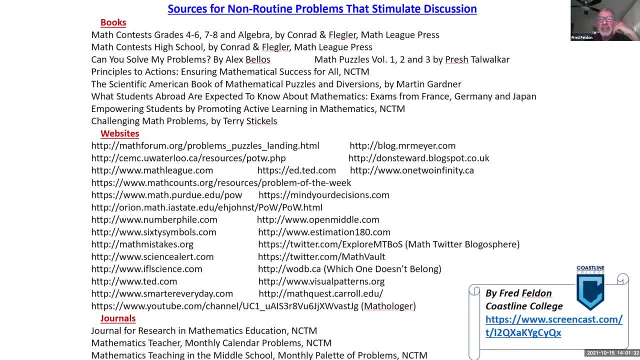 zoom meeting. i also have a collection of non-routine sources to get you away from doing routine homework problems. those aren't in my mind. those aren't really discussions i i want discussion prompts that are open-ended, with no one correct answer, and here are some great resources. okay. 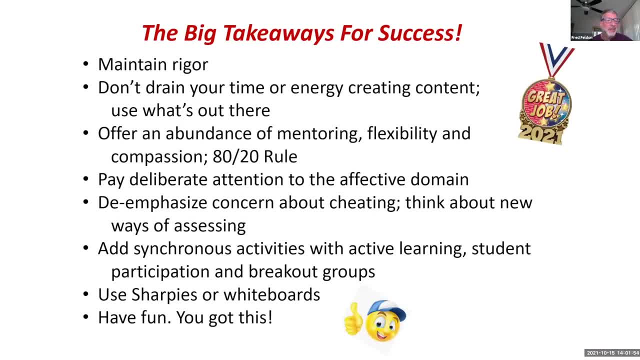 i show that my time is up. i have my last slide right here. some bullet points to summarize: don't water down the curriculum. just because you're teaching online doesn't mean you should skip anything in the course outline of record. uh, don't worry about taking time to create content. you've got, like i said, internet gurus and textbook. 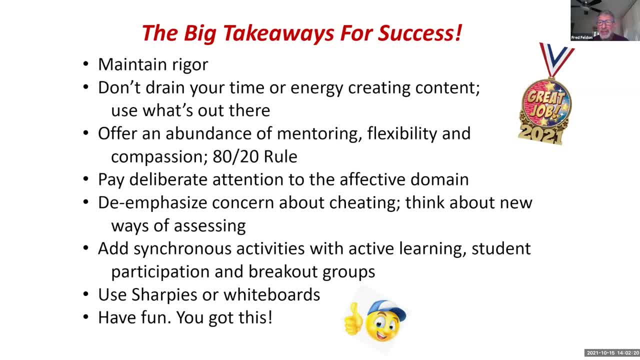 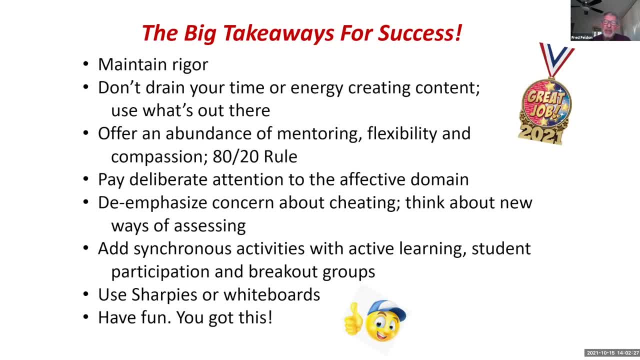 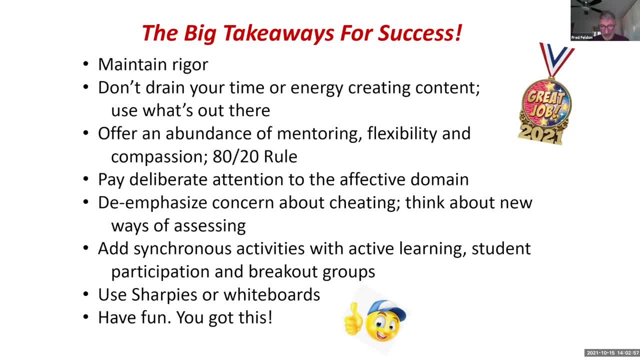 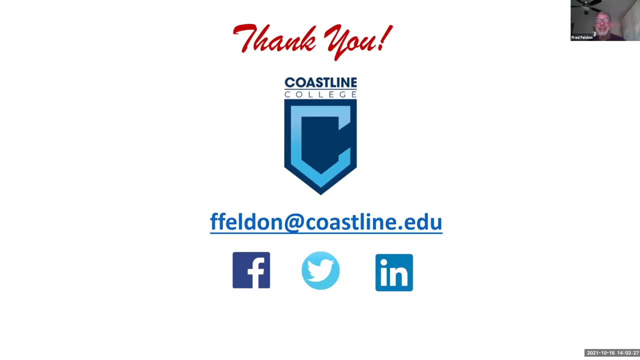 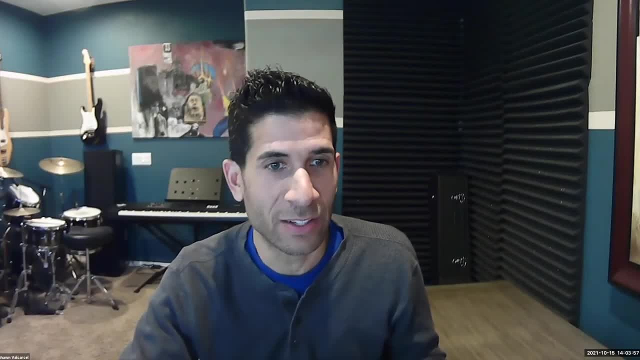 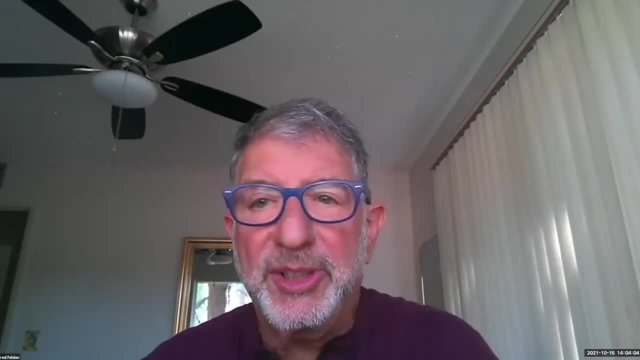 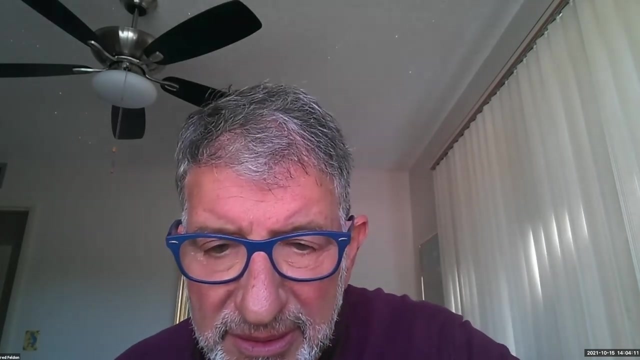 question, and then chow was raising his hand. so, uh, in fact i'm gonna go ahead and, um, well, if you want to go ahead, i stopped sharing, did i did? i knew, do i need to put that slide back up with my email or anything? um, if i assume not, you could put: yeah, you could put in the chat, and okay, and then i just 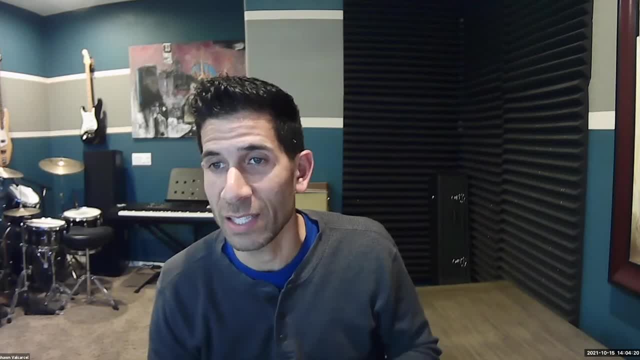 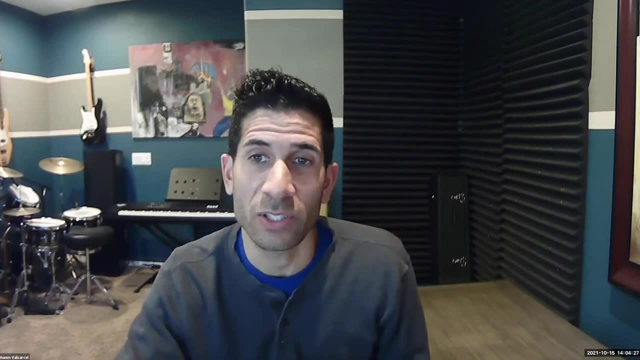 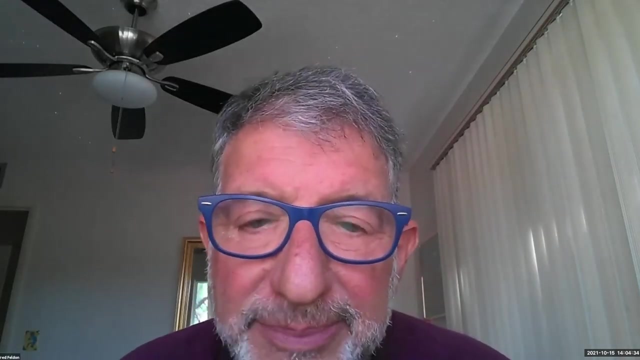 want to let everyone know that cvcedu forward slash events. uh, you'll be able to see the archive of the video to this session. if you want to go back and do that, so okay, i just typed my email in there. so now i have the chat open and i see allison's recommendation and then, if you look, 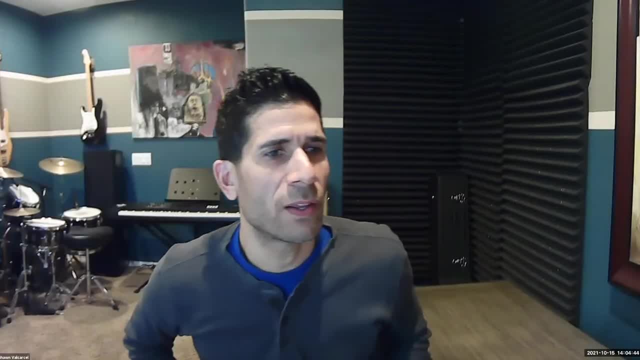 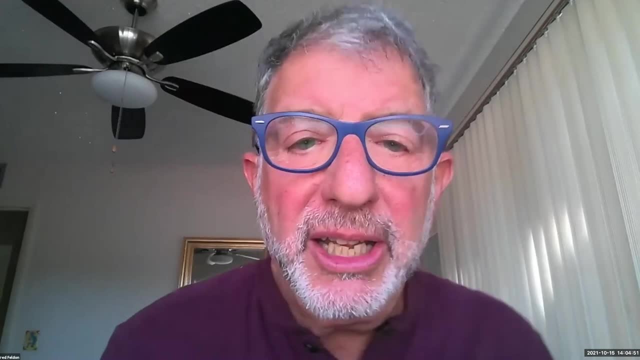 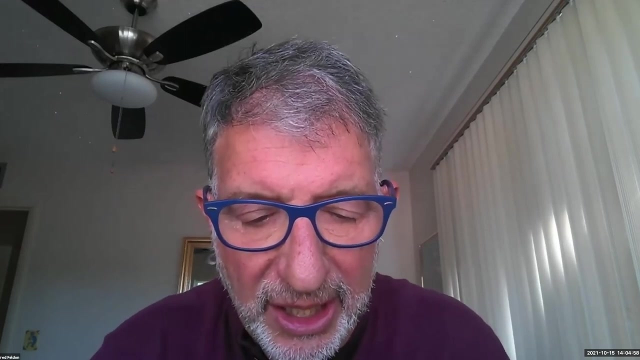 at the q a, uh ming had a question. okay, i'm here in the chat, i've got a, i've got a great three minute youtube video. allison is asking: how do i deal with fear of math? because it's, it's definitely out there and i i say go, i'm going. 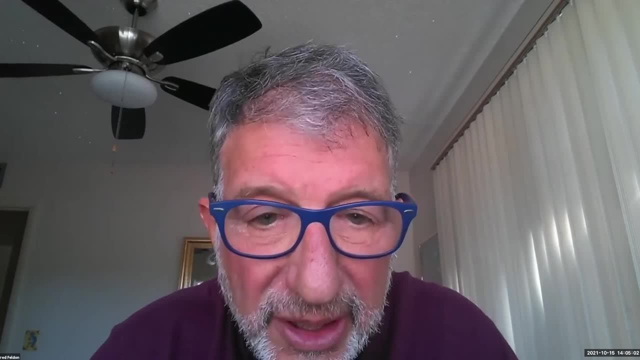 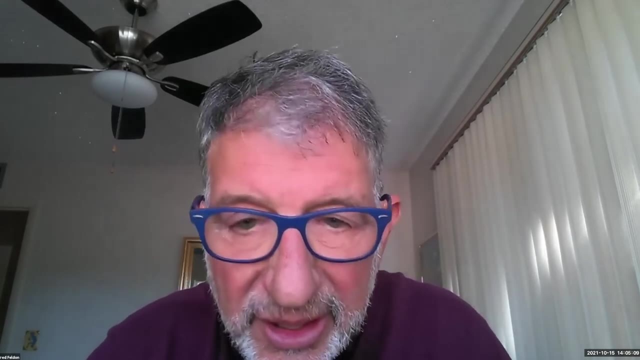 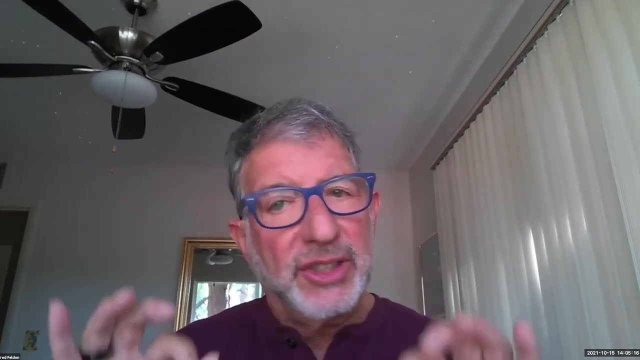 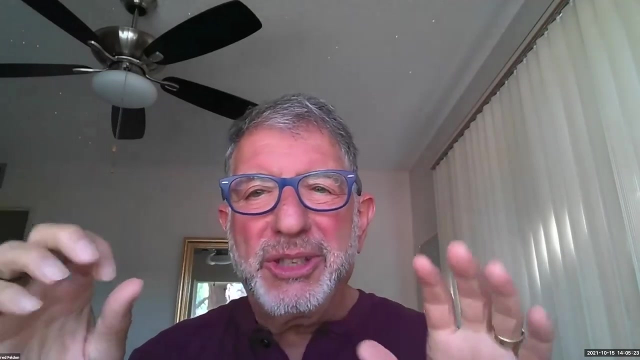 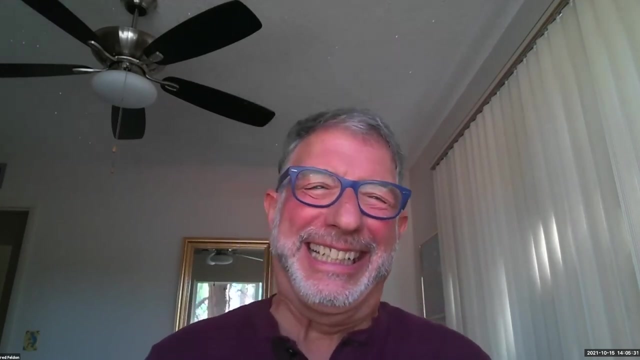 to type in the chat, go to youtube and google. a math major talks about fear. it's a very popular short three minute youtube video of this cute blonde math major student with big eyes and an expressive face who talks about what happens when she goes to parties and she introduces herself to people as a math major and their 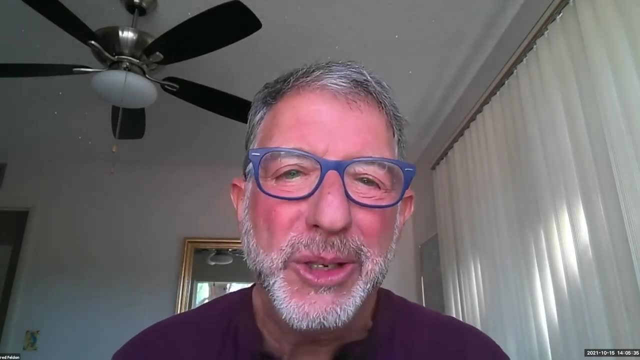 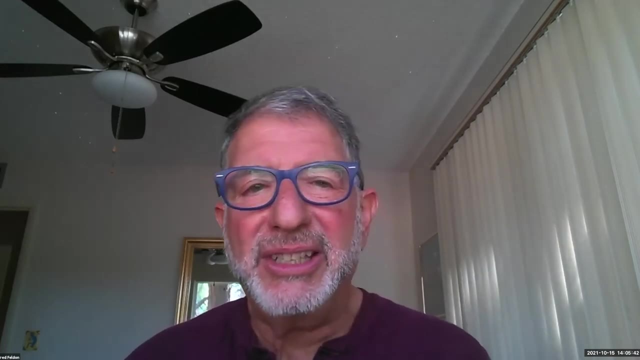 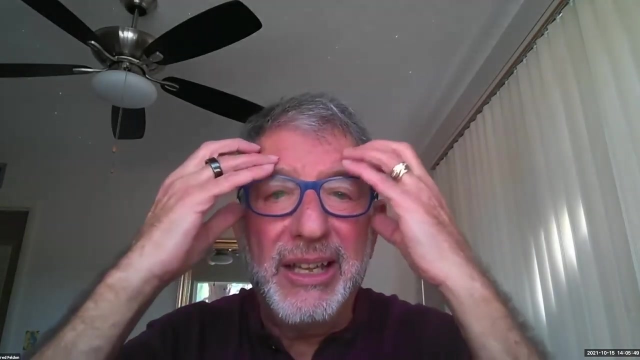 reactions. and then she talks just about what you brought up: allison math phobia and the fact that you're in a class and there's all these other students that seem so much more knowledgeable than you and you're feeling stupid. and she describes allison math phobia and the fact that you're in a class and there's all these other students that seem so much more knowledgeable than you and you're feeling stupid and she describes- you know how to handle that mentally. 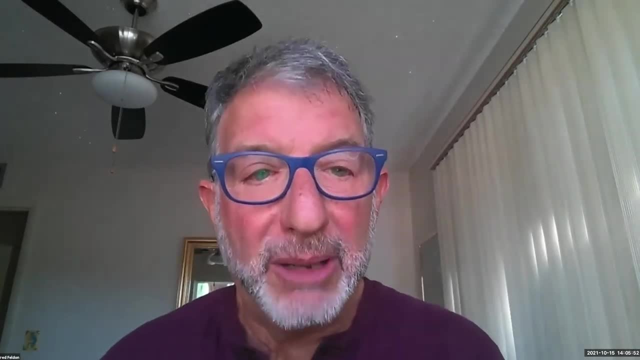 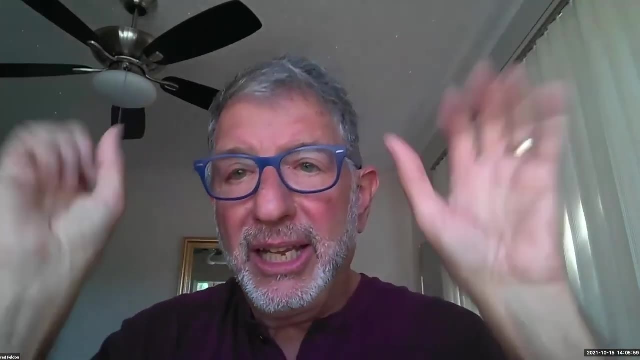 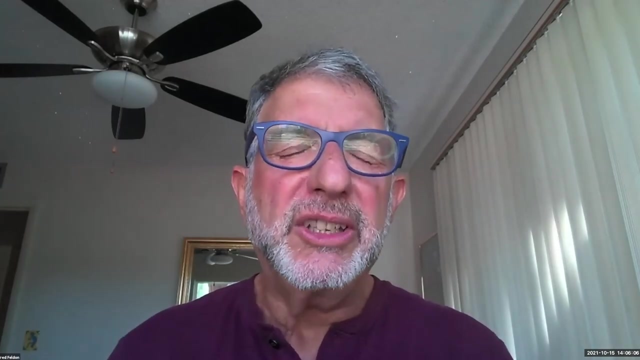 within your own mind and i post that as a discussion prompt and it ends up every semester being my most popular discussion. you know i and i'm very, i'm very uh, casual about discussion prompts. i i've been to a lot of other colleges where they have professional development. 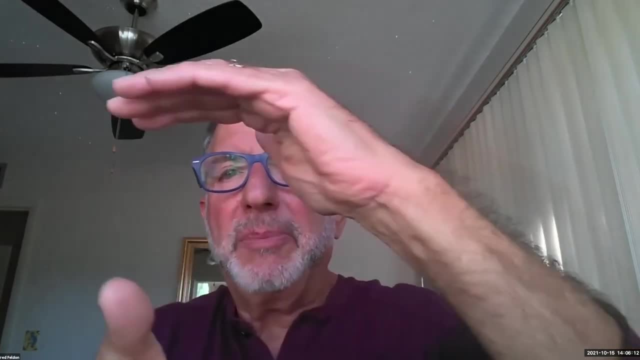 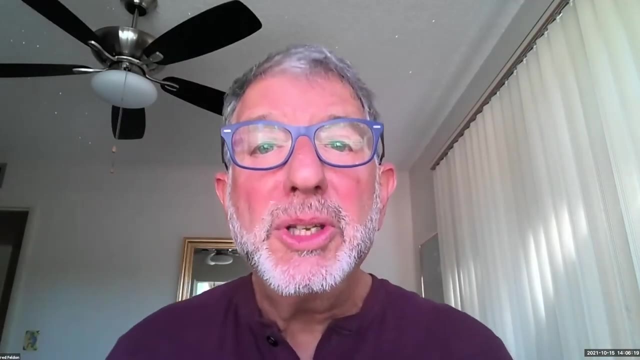 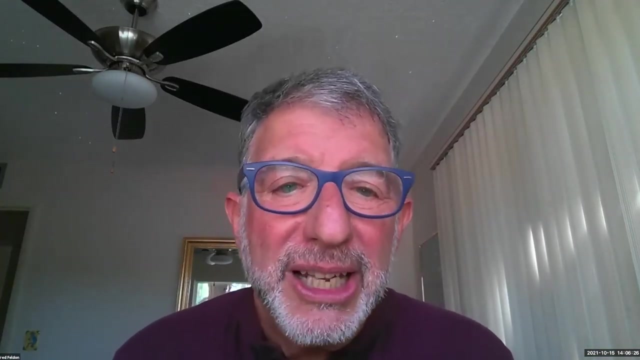 with giant handouts and and and fill in the blank questionnaires and reading assignments, and i, i just, i'd rather just post a meme or a three-minute youtube video and say, please comment. it leaves students a lot free to really do what they want, and sometimes 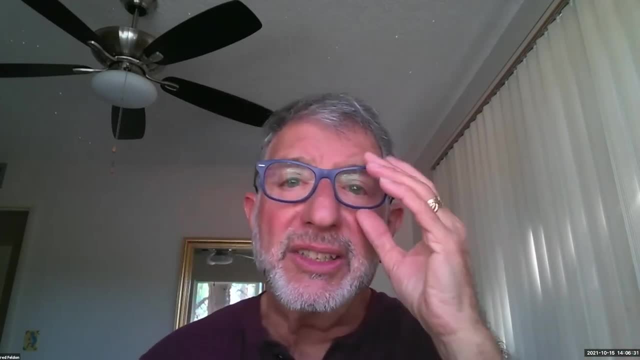 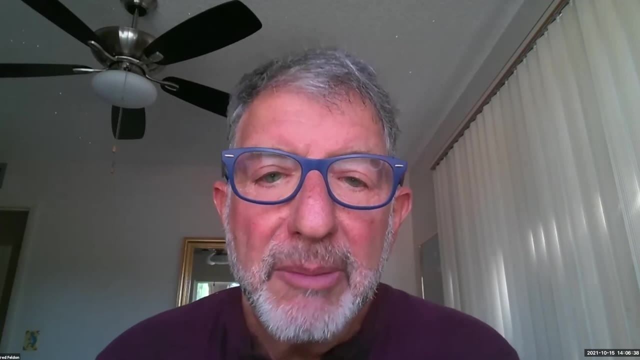 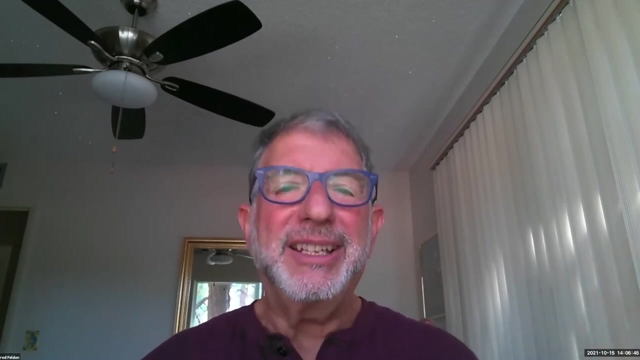 many times- not for the video i just mentioned, but for other activities- i will hide student responses until a response is posted. if that's appropriate, you can do that, but for this particular youtube video i just post it. i say for extra credit, just post a comment and it's the most popular. 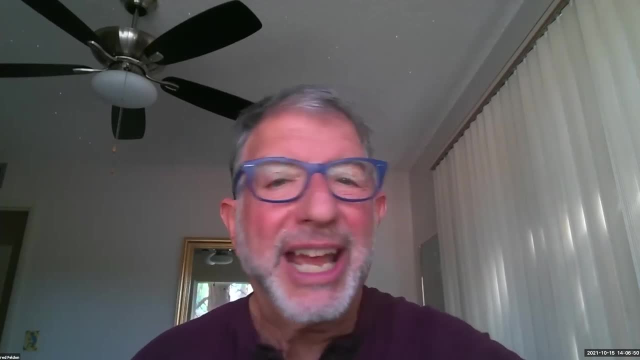 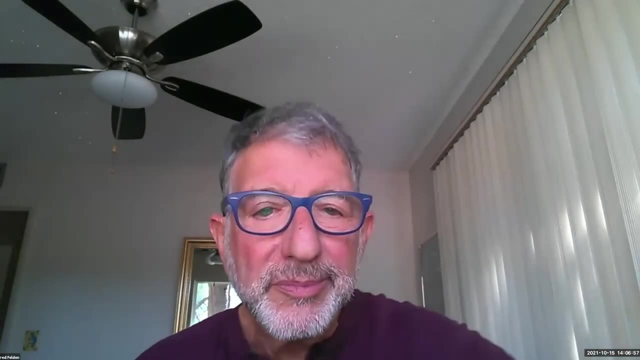 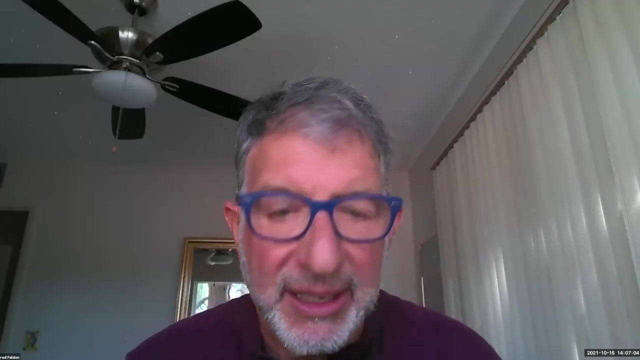 uh, extra credit activity and discussion prompt i've ever had now for many years, so try that. let me know how that works. anything else, are you able to access the q? a fred, yeah, i'm seeing. miguel said he uses that video as well. um, oh, i'm sorry. look in the answer. 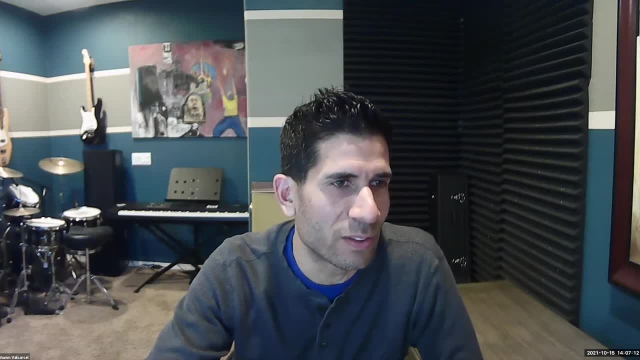 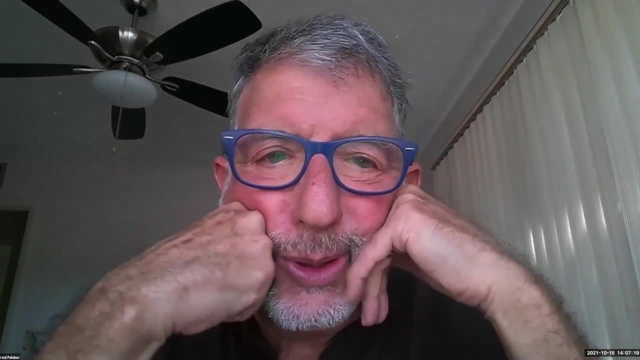 click over to the answer that. that's, that's the one that i was. oh, the q a. there we go. yeah, that's different. oh, okay, allison, another uh post. i know a lot of our students are afraid of math. oh, that's what i was just answering, so click on the answered one. 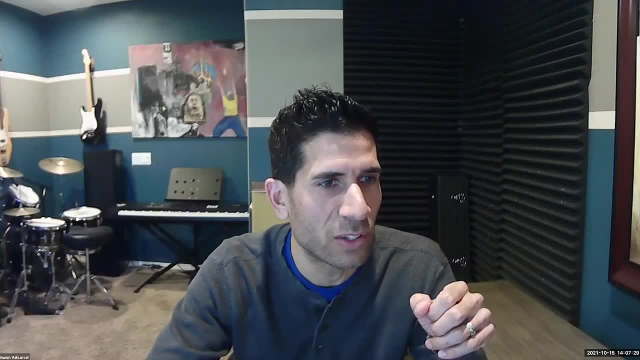 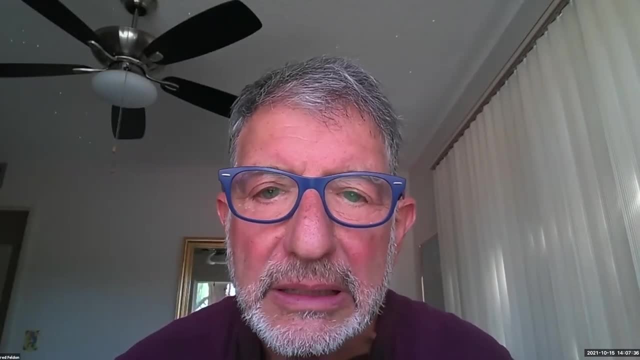 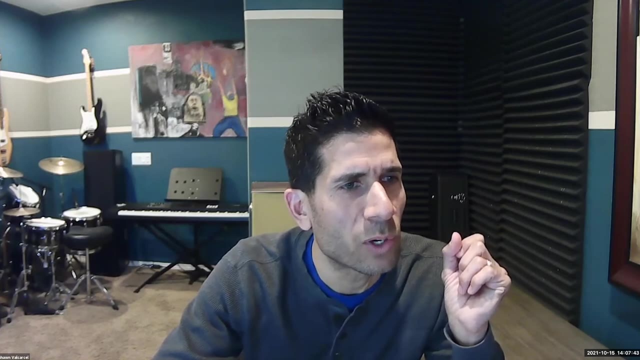 because, uh, ming had a question. you would like to answer this question live. does it give you the option to see? okay, so ming says: how do you ask students to show what they're working on? how do they transfer what they're writing or what's writing on their own paper to be visible to you and others? correct, that was one, a small part of. 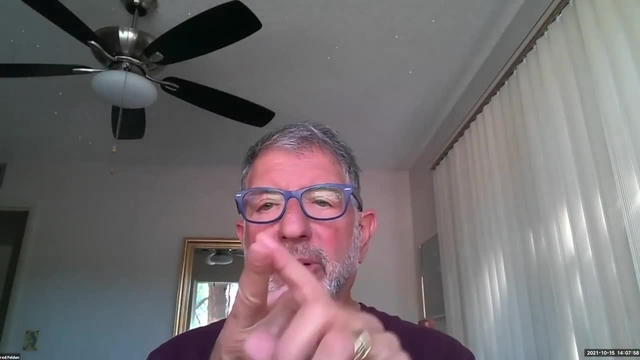 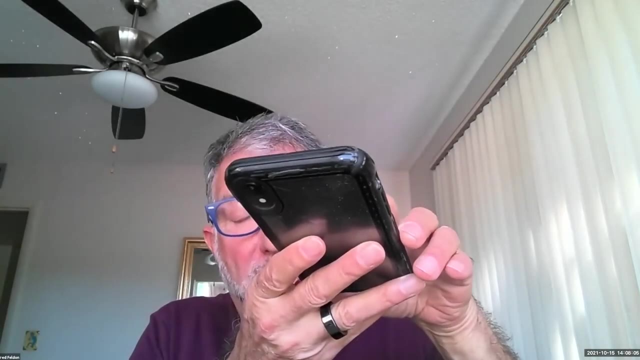 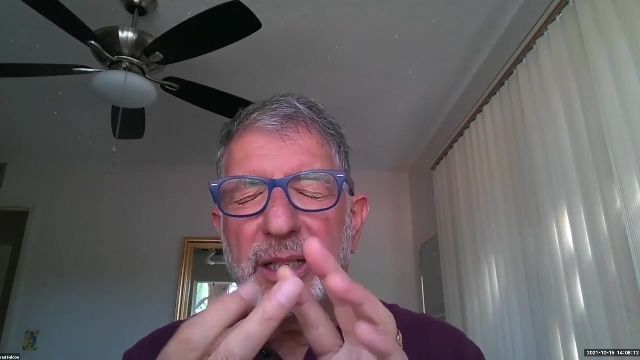 my website where where I said several things. number one: write on paper and pencil, like they're used, to take a picture of it with their cell phone and attach that to a discussion board post or a chat message. that's one way. another way is to use a Microsoft Word has a math editor and you. 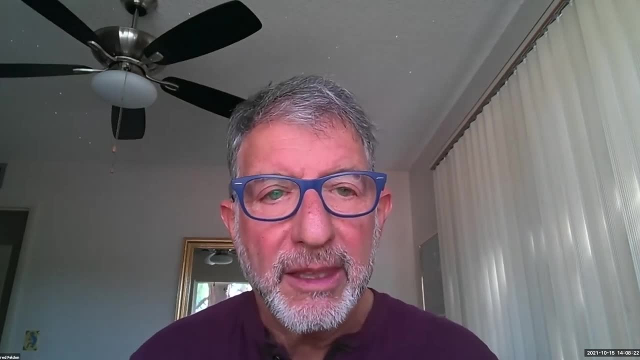 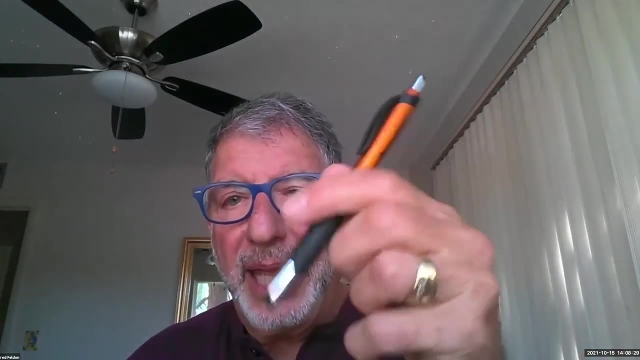 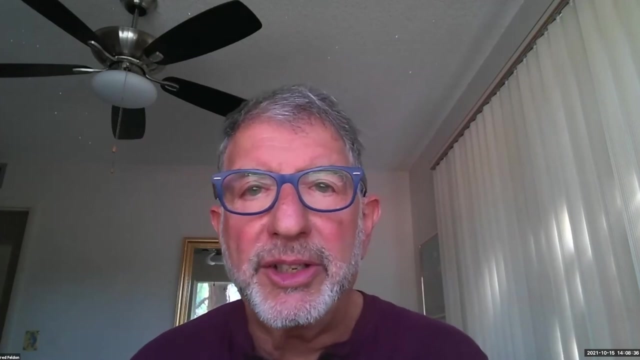 can type that into a discussion board field. another way is to mark with a thick sharpie on paper and hold that up to your webcam. I've done that many times where I've asked 20 students you know. graph this parabola and show me the vertex and the intercepts. 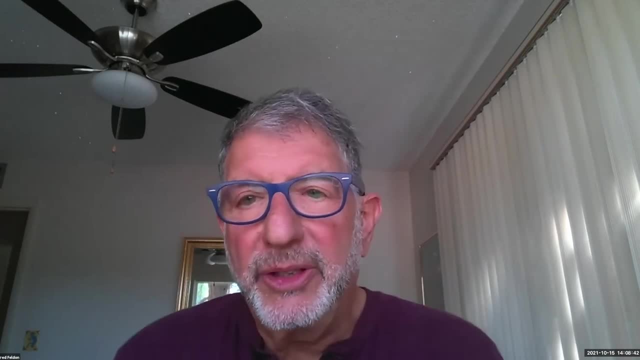 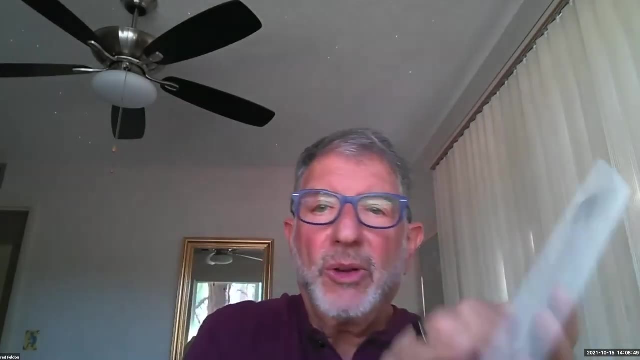 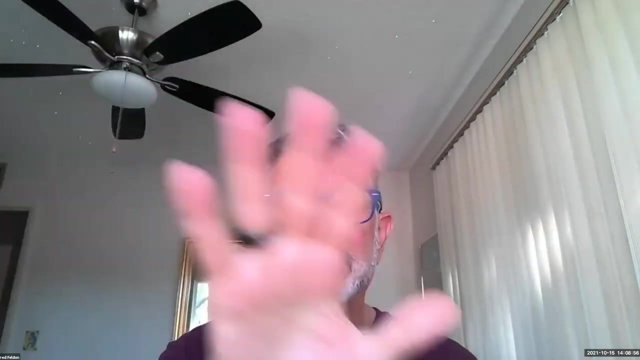 and then I walk away from the camera and give them a few minutes and then I say, okay, let's do a share out, and everybody holds up their paper, their paper to the, and I can see if we're in gallery view and I can see everybody's graph. and then the third way is the little individual mini. 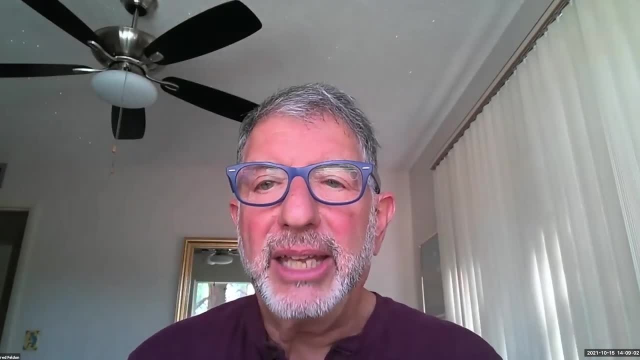 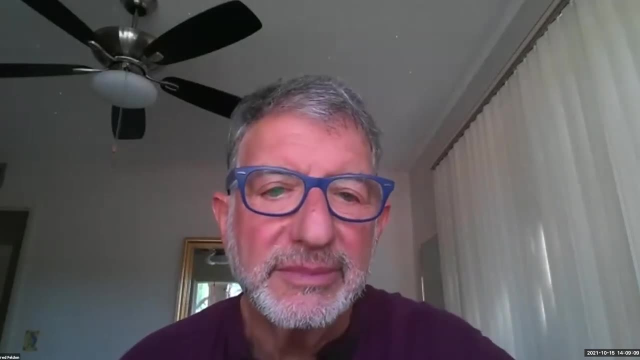 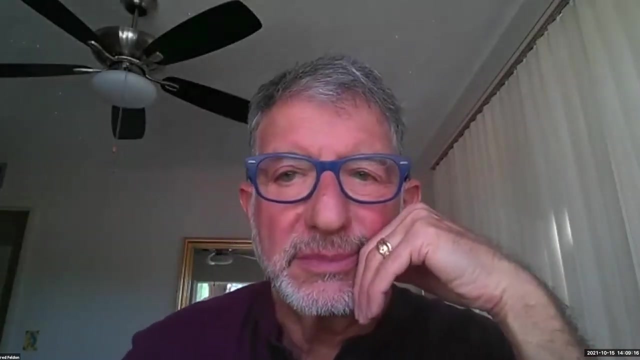 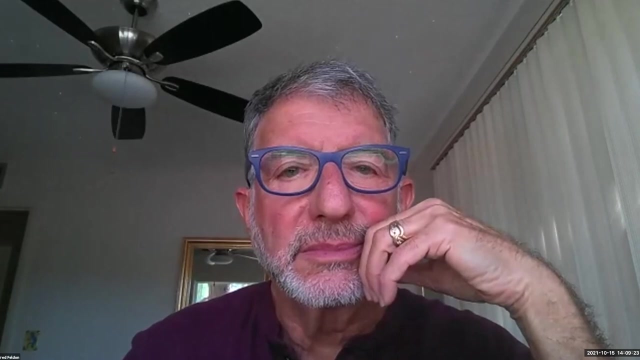 whiteboards. have students spend 10 bucks on Amazon and buy an individual mini whiteboard? can I talk? yes, okay that. I found I figured out an extremely powerful tone in the GeoGebra classroom. it means that I invite students to the classroom when they write anything. I see right away in real. 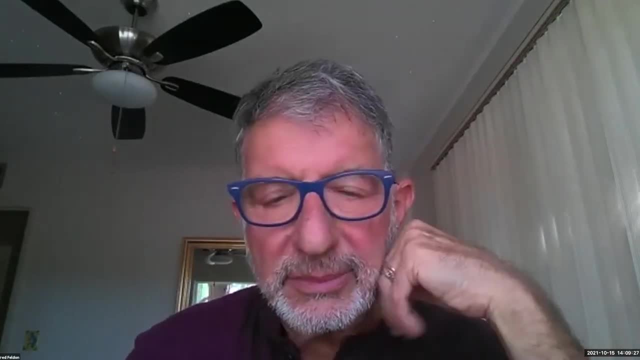 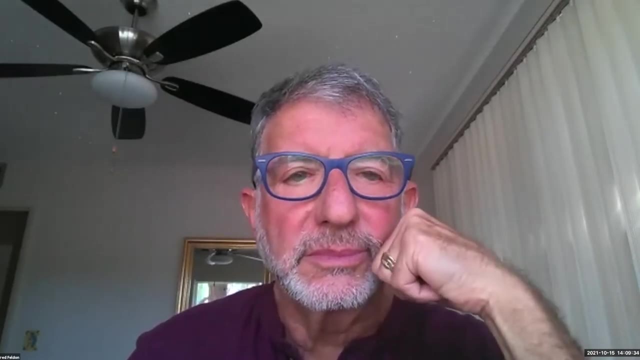 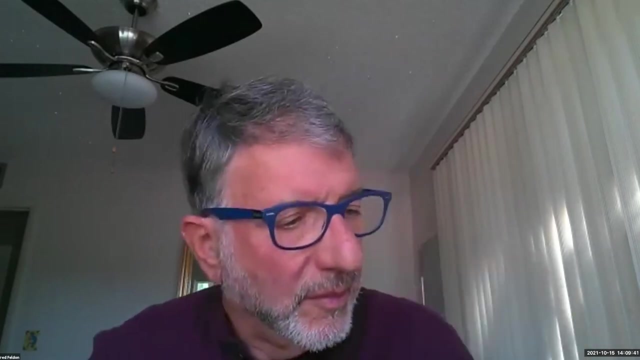 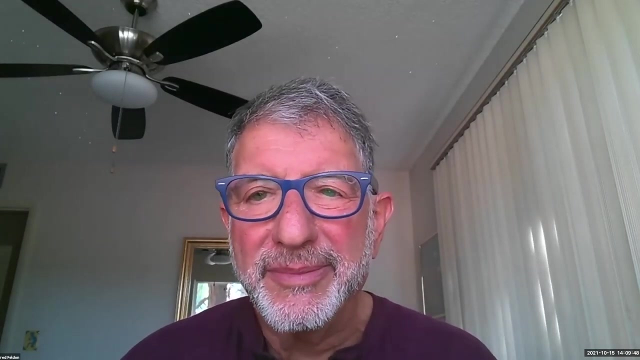 times. but that is, you create a classroom in GeoGebra and you invite students go to that. you separate in group. they like it, and when they write on that whiteboard, you see right away, right away. yeah, the problem is that's a digital whiteboard, so how do you write on that with your mouse? uh, any, yeah, because they have. it looks terrible if. 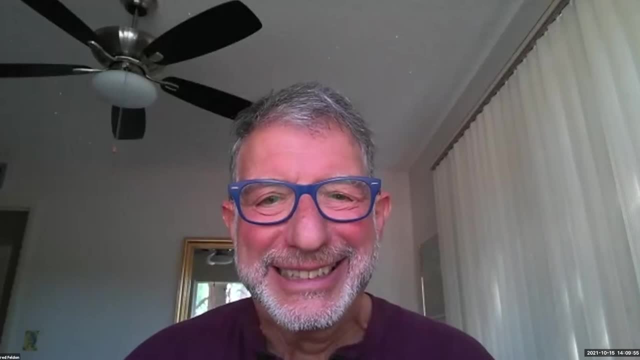 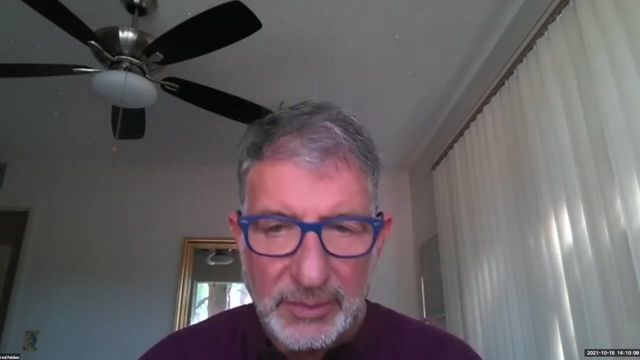 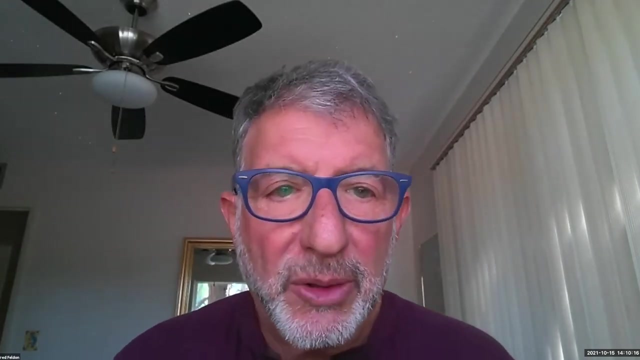 you write. try writing with your mouth. because the question of uh Ming, I think that, yeah, we like to see how students work that time when you are in breakout room. you see how they work, how they share sometime. okay, you see a- you mentioned that Asian, not a good writing, but we see how they think. did they try? I just recommend experimenting GeoGebra or 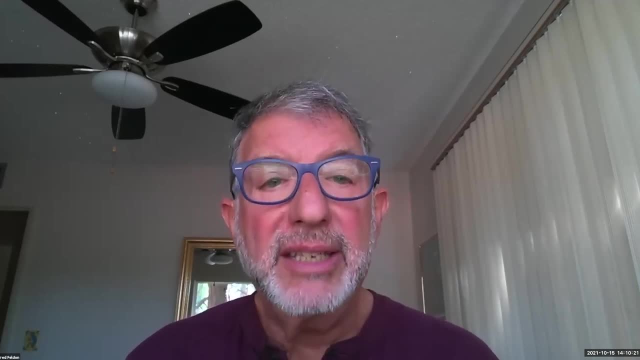 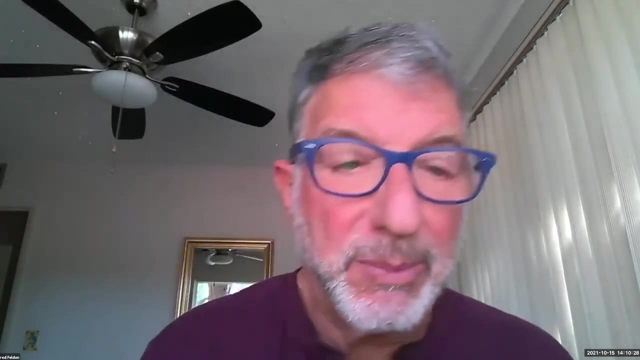 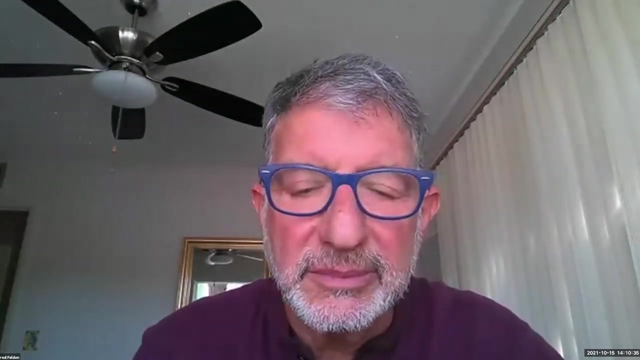 you know what other great, fantastic program is desmos, desmos? if you have not visited desmoscom, you need to find out what that's capable of. it's similar to GeoGebra I. I think it's even better. I like it even better. it's one of the. I think that we are really behind. 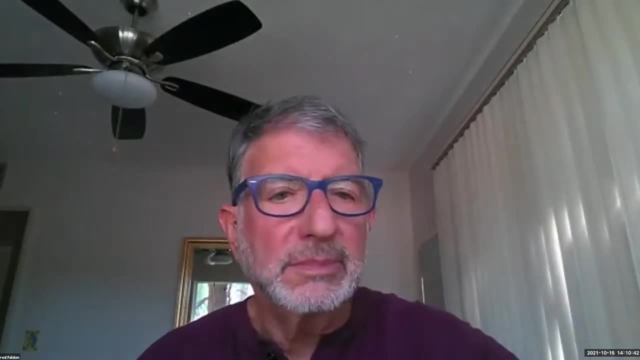 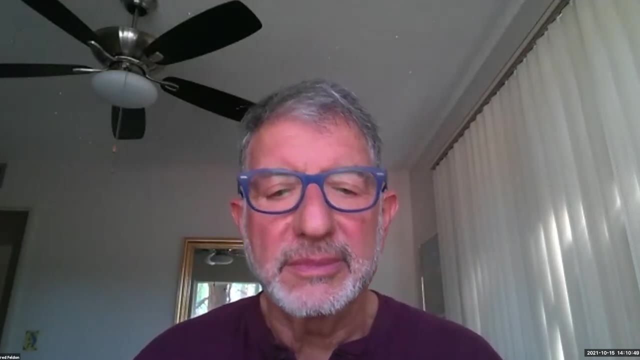 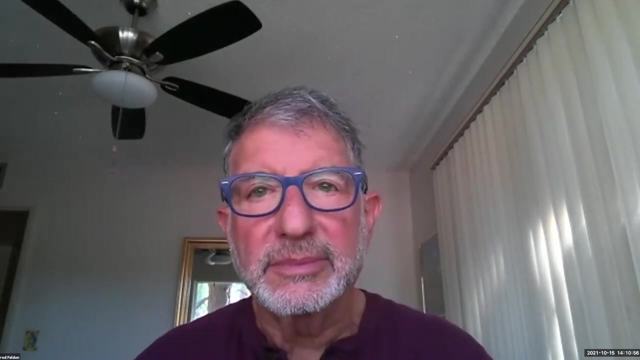 with the AI and GeoGebra GeoGebra classroom, that AI, AI and you see, that that's why we can see how student drive right away. that's what I think that the most advanced uh technology now with the, how we see students write and think in real time- that's I think that I can contribute to the main. 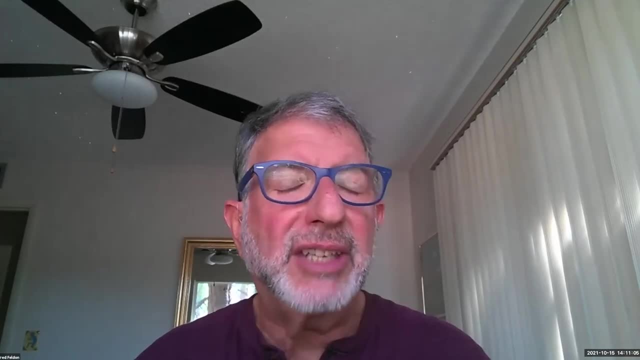 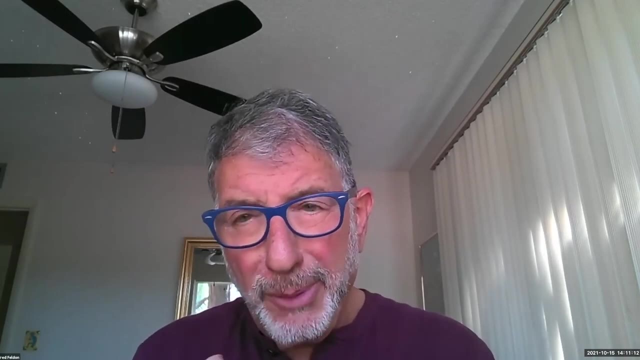 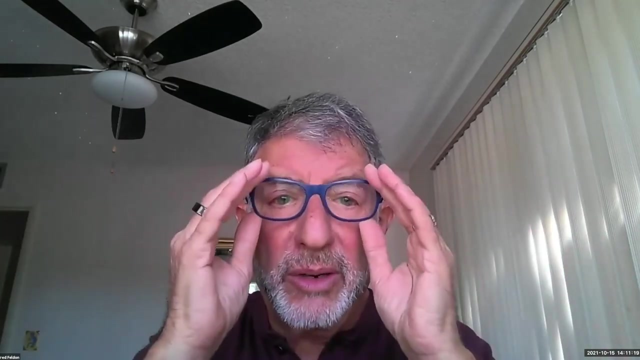 question. yeah, that that's a challenge in any stem discipline, so I recommend that you re look at GeoGebra, desmos, a mobile scanning app on your cell phone, Sharpie pens, white boards, the, the webcam, all those things- there is no one right answer- and then share out with your colleagues. 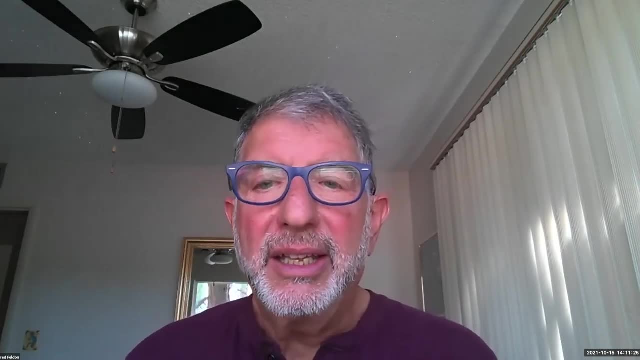 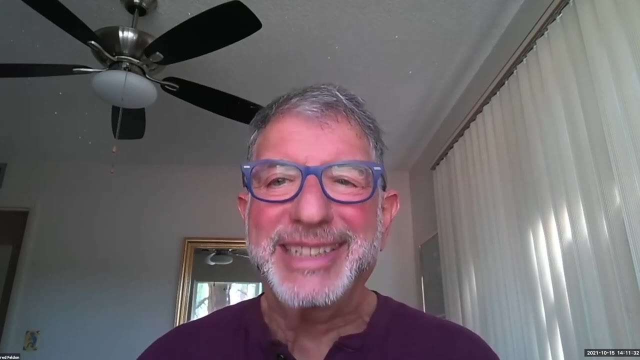 in your department meetings. share what you're doing in these types of webinars. share what you're doing and we'll feed off each other's ideas and learn from each other. that's the way to do it. yeah, I can tell you. when I first got my tablet PC, I